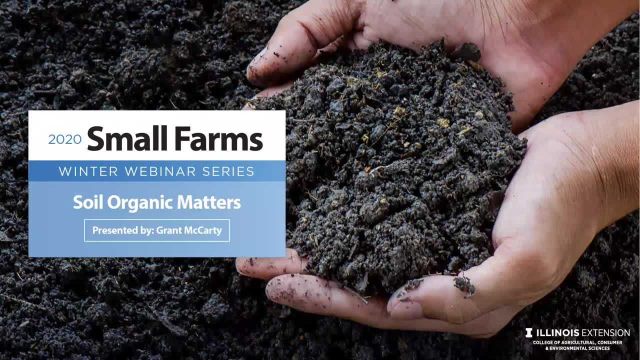 the end of the day There will also be a short online evaluation for this presentation, including the email, so we really much appreciate your feedback. You'll also see it on the last slide of Grant's presentation today. they will be a QR code that links directly to the survey so you can use your smartphone. 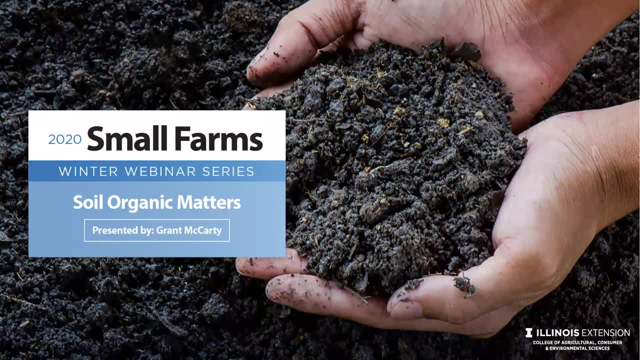 camera or your QR code or QR code reader app to directly take the evaluation at the end of today's presentation. We are using Zoom's webinar platform this year, so there's a few additional features I just want to quickly point out. There is a poll at the bottom of your screen, so if you click on the poll, I see some of 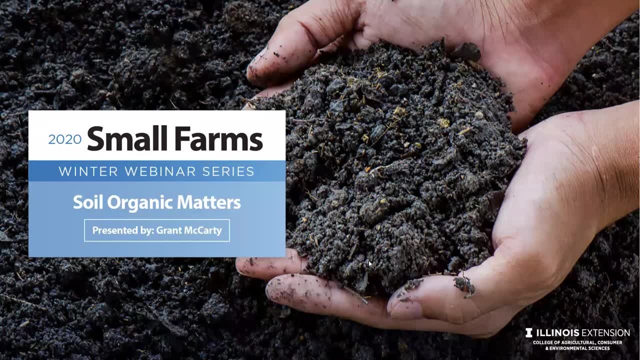 you have already begun filling out our voluntary demographic information. It's really useful for us to collect this information, so if you could go ahead and complete that, that would be great. There's also a Q&A section and a chat box, so if you could keep your the questions that you will have for Grant in the Q&A. 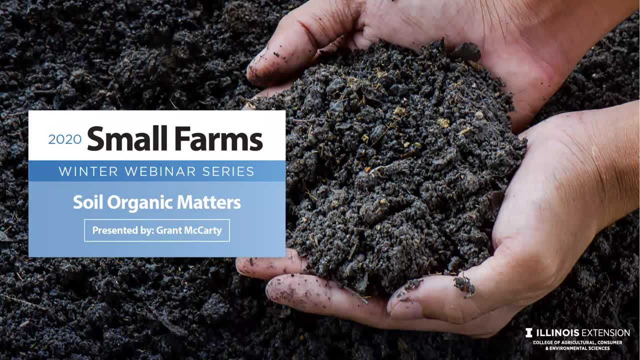 box and we'll reserve the chat for some of your technical problems that you may be having. So this week's presentation is from Grant McCarty. Grant's, my fellow local food small farm educator in Joe Davies, Stevenson, Winnebago counties. in. 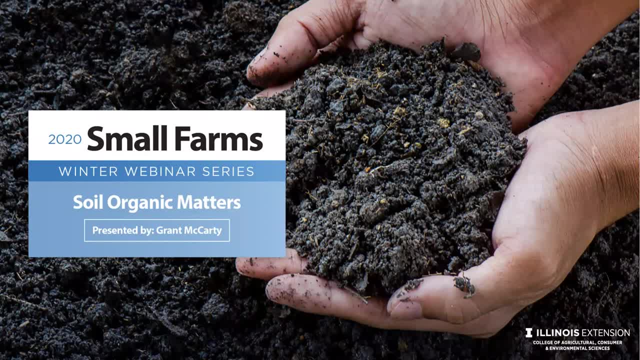 northwestern Illinois. He's originally from East Tennessee and Grant works both with commercial and backyard growers, Mainly focusing in fruit and vegetable production. He has some expertise in soil management, hops and production, or hops production, general and general organic sustainable crop production. He assists stakeholders within the local 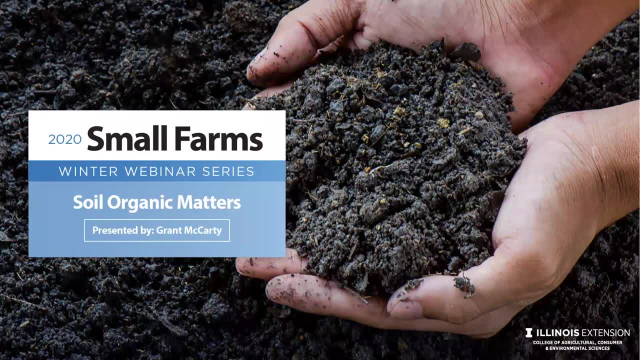 food system in helping them to expand their operation and adopt new practices and better manage their current production. Grant's educational background started with a bachelor's in sociology from Maryville College, and then he did his graduate work in plant sciences at the University of Tennessee. 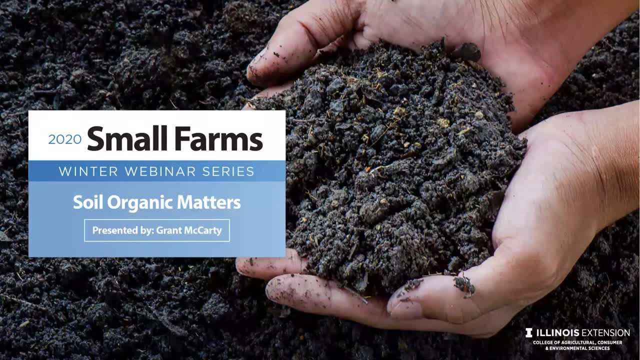 Over the next two weeks, we're going to be taking a deep dive into topics related to soil and media management. This week, Grant is going to take us on a detailed deep dive regarding soil organic matter, and next week, I will actually be discussing saturated media extract testing as an alternate soil and 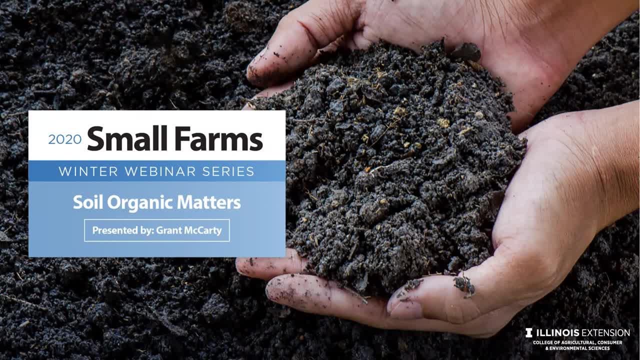 media test for certain conditions. With that, I'm gonna relinquish the floor to Grant. Go ahead and take it over, Grant. All right, well, thank you, Zach. Thank you for the introduction. I'm happy to be here with you all today, especially talking about a subject that's really something I really get excited about, and 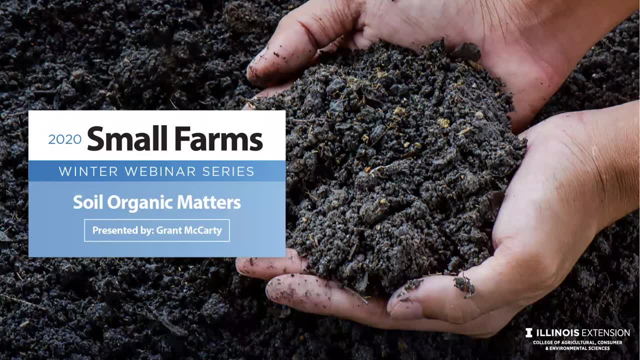 really like to share with others. Most of my work in our extension unit and kind of in our area tends to be working a lot in soil science and particularly in soil biology Over the last couple of years. we're starting to see a lot of folks. 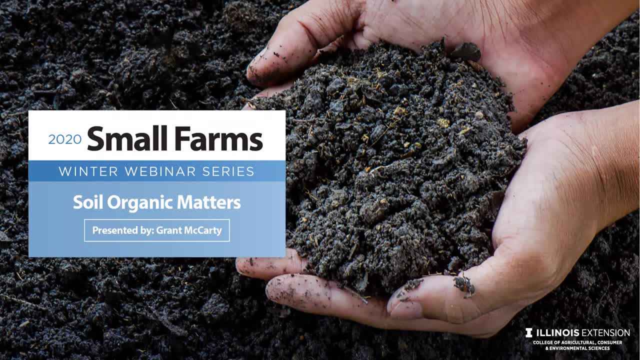 that are beginning to kind of wonder a bit more about the soil, health, organic matter that they have in their growing area and begin to kind of also wonder a bit more about how to use organic matter effectively, what they are and kind of what they're doing to the soil. So what I tried to really do today was to kind of 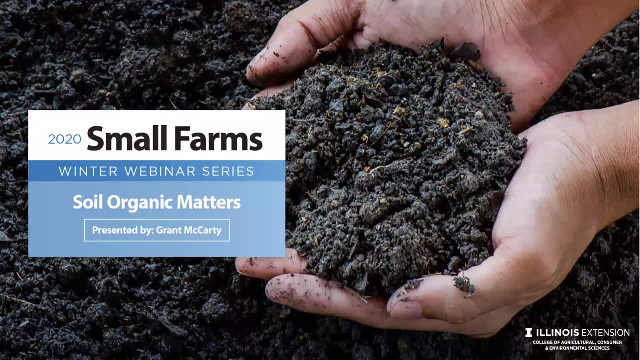 zero in and hit some of these highlights when it comes to managing and using organic matters, as well as addressing what your soil organic matter is in the soil itself. So if you are familiar with some of these principles of soil biology and soil health, this might be a bit of a refresher for you, for you today kind of. 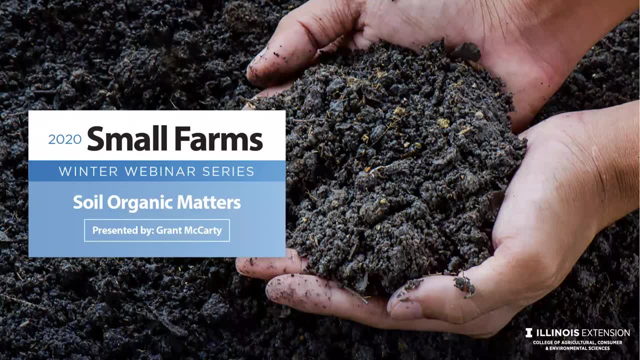 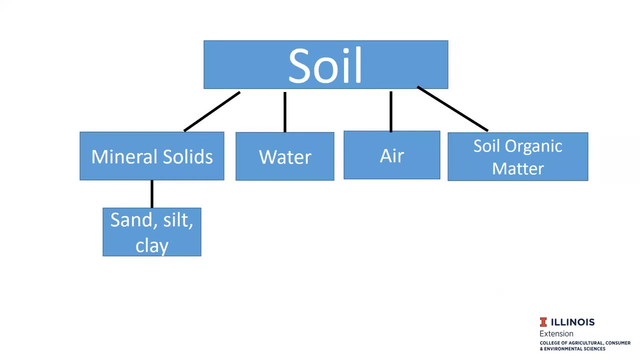 as we go along. Alright, so to get us going, you know, just as a refresher, you know what is soil, what are the four components of it. This is our mineral solids, which is our sand, our silt and clay. So that kind of that soil texture is where the mineral solids really tend to be. 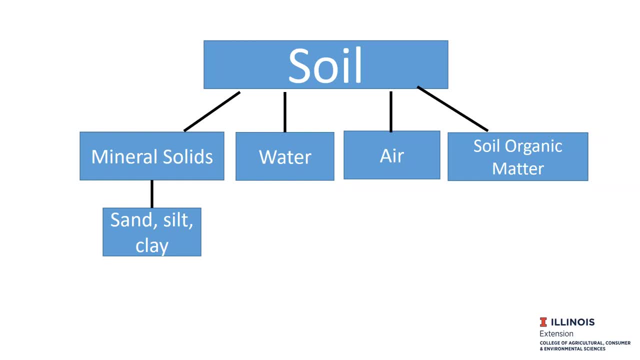 We have water in the soil, the H2O solution. We also have air in the soil, allowing for good oxygen exchange, and then we have a soil organic matter. So this SOM, which you'll hear me talk about a lot, kind of as we go along today, And 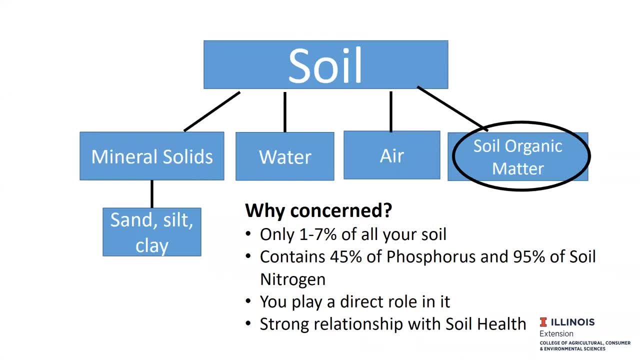 we're going to talk a little bit more about that in just a couple of minutes. And we're going to talk a little bit more about that in just a couple of minutes, And we really are talking about the soil organic matter here. When you get a 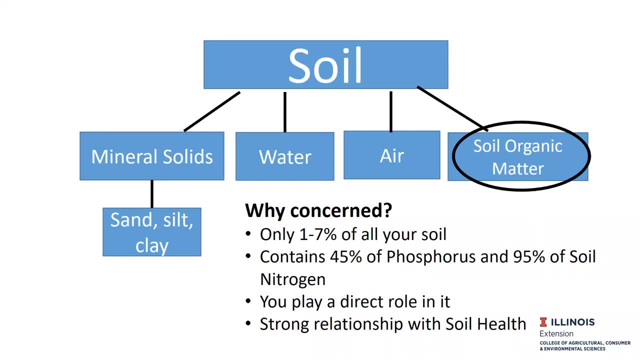 soil test done. you get this measurement back to you that lists the soil organic matter, And usually what we see in a typical soil test is that about one to seven percent of your overall soil. The issue, though, is that you know 45% of the soil phosphorus and 95% of the soil nitrogen is actually within. 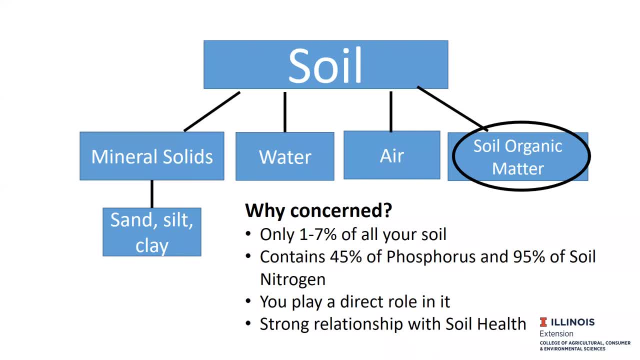 this percentage And sometimes I have soil tests that come across my desk that are two, three percent. Sometimes we see up to five, six percent. But I think it's important to realize from a grower perspective. you play a direct role in this And this is a positive thing. You could be adding compost manure growing. 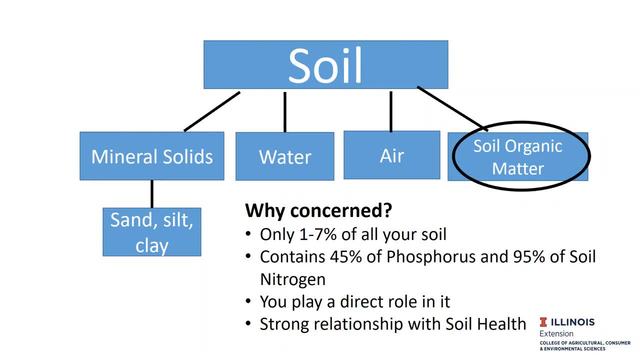 cover crops, leaf litter and so forth, which would be breaking down and eventually add to this percentage, Or you could be doing a lot of negative things. So it would maybe be doing a lot of heavy tilling every year, Not adding any organic matter, Maybe exposing the soil to soil surface. 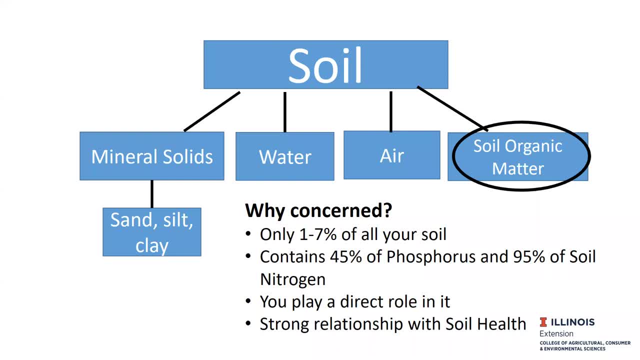 without having any kind of layer of protection. So you have a direct role here and it's very important that you kind of recognize this, especially going forward today with it, And we'll talk more about this, even more so As you look more into soil health and maybe think about that with your soil. 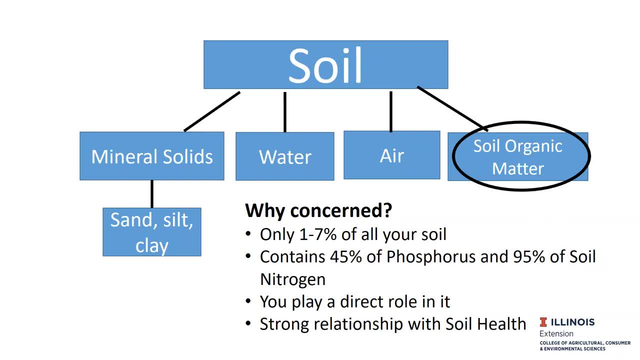 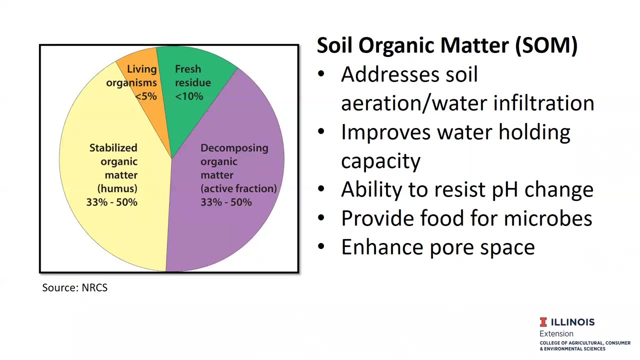 you will find that soil organic matter tends to be a very strong focus in soil reproduction, soil health and the overall soil health management of your soil- a couple of additional things that soil organic matter does. and this is where you see I, you'll see SOM, so I'll use that throughout today's presentation and I'm 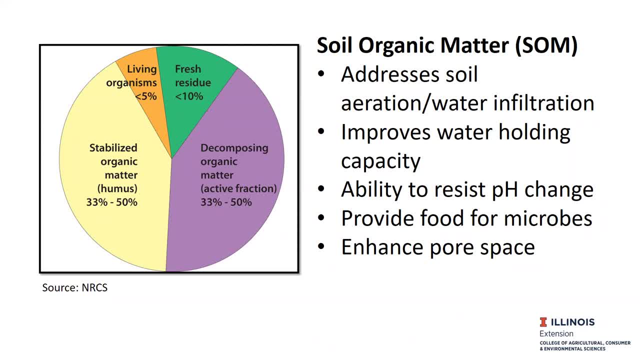 talking about soil organic matter. it addresses soil aeration, water infiltration. so it really helps both of those things. when it comes to kind of making sure the soil is resistant to compaction and allowing for good water and air exchange to occur. it also improves quite a bit of our water. 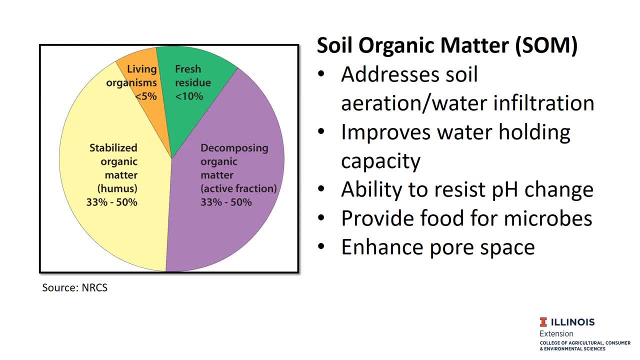 holding capacity, ability for the soil to hold water and for our plants to utilize and pick it up. it can also help quite a bit when it comes to the ability to resist any soil pH changes which you might see, and then what we'll talk a lot about today is that this soil organic matter actually provides a lot food for. 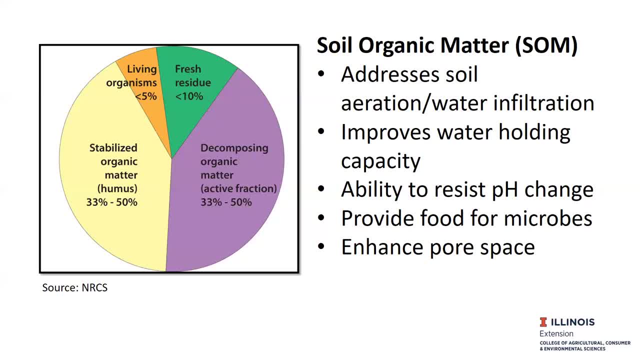 the microorganisms and the soil biological communities. you may also find that it will enhance space. so when you get a soil test and you'd say, my soil test came back and it was a two to three percent of that, two to three percent we may, you may know a. 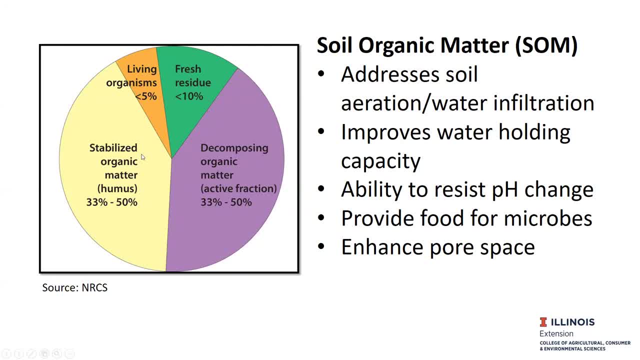 little bit. as far as you know, as you kind of see in this photo here, this two to three percent would include a percentage of decomposing organic matter that's called the active fraction. would also include a stabilized organic matter which is known as humus. So this is a fraction of that two to three percent, so kind of that. you know, between 33 to 50 percent of that two to three percent is decomposing organic matter, which is called this active fraction. 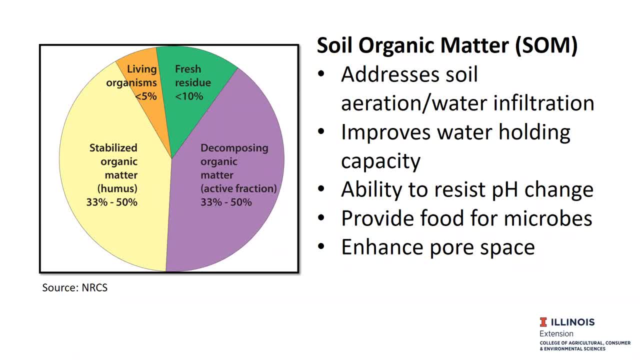 Talk a little bit more about that. as we go along today, In most cases, the organic matter that you've added in the last four to five years- your compost, your leaf litter, your cover crops that you might be growing- it is still within this category of active fraction, so it is still decomposing organic matter. 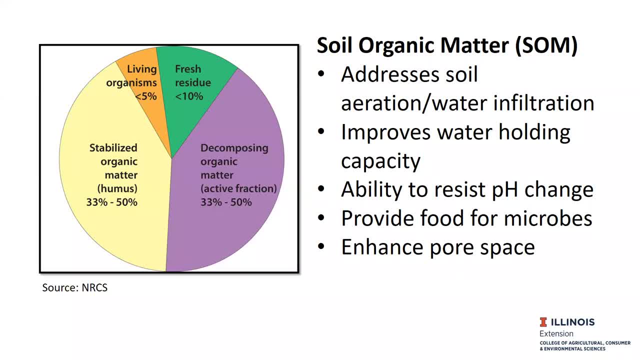 So it is still decomposing organic matter. So it is still decomposing organic matter, But our long term goal is to actually get to become the stabilized organic matter, this humus of 33 to 50 percent. But our long term goal is to actually get to become the stabilized organic matter, this humus of 33 to 50 percent. 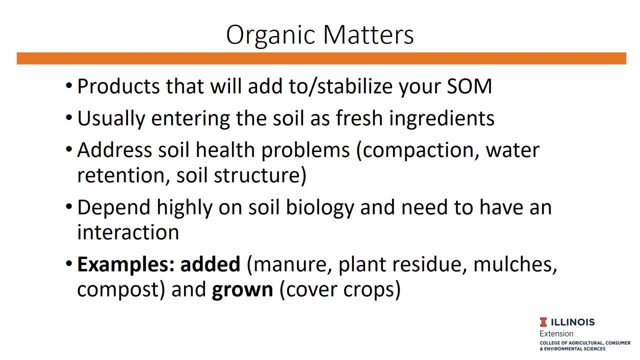 So organic matters, then, are products that will add to and stabilize your soil organic matter. When I add compost to my soil, or I add leaf litter or manure, it will be decomposing, It will be breaking down, breaking down and it will eventually, we hope, get to that percentage of soil organic matter. so it's 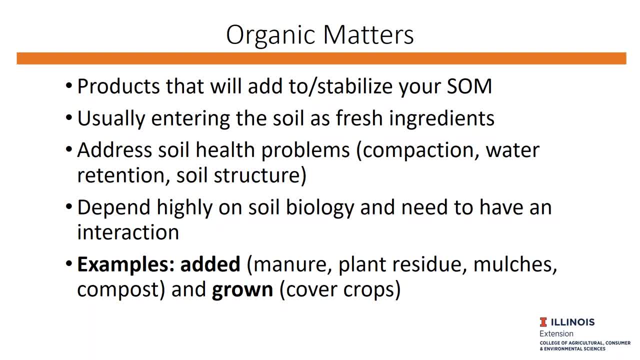 a very long game to get there. you know- and that's what we're- what's really happening when you're adding the organic matter. it's usually entering the soil as a fresh ingredient, even if it has been a little bit stabilized, say like a compost or an aged manure, perhaps it is still kind of what. 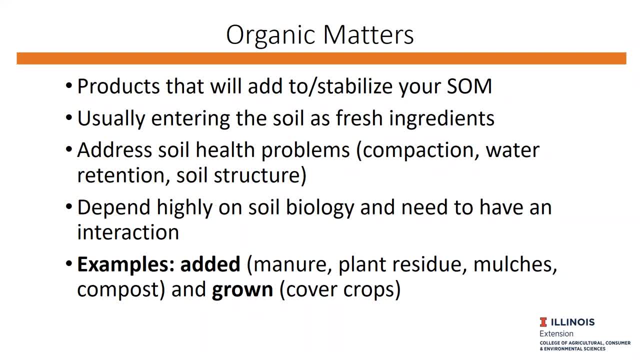 we consider a fresh ingredient at this point. it's got to be broken down and decomposed by our soil biology. it addresses soil health problems, like i've shared with you: compaction, water retention, soil structure. typically when we have a grower that we're working with that has one of these. 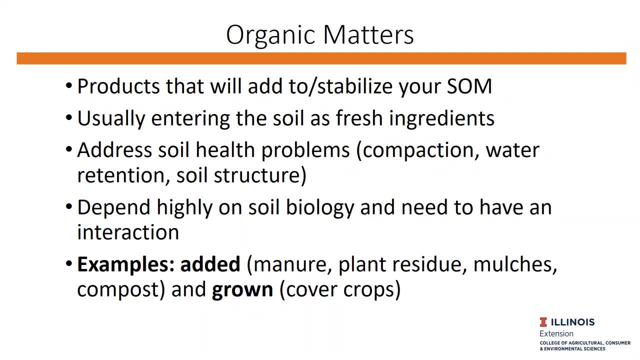 health problems. we kind of ask: you know, we kind of tend to recommend an organic matter as the best recommendation for addressing this. organic matters depend highly on soil biology and they need to have some kind of interaction. we'll talk more about this as we go along today. 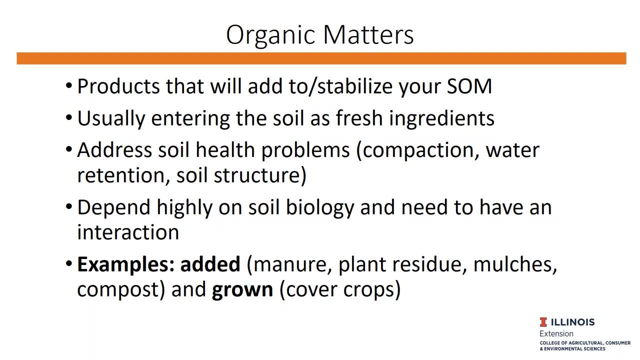 this interaction really needs to occur in order for my organic matter to break down, to eventually enter into that soil organic matter percentage. there's two broad categories of soil, of organic matters. in this case we add in, so this is something with manure plant residue mulches. 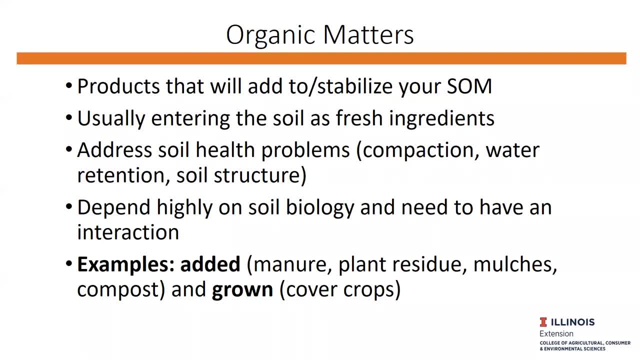 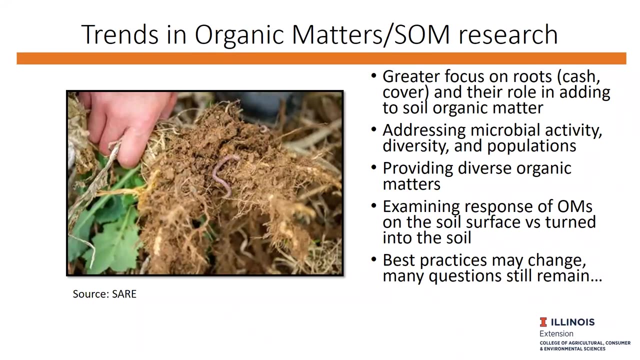 compost, something in which you're actually bringing and adding on to the soil, the soil surface, or turning into the soil itself, and then you have your grow, your cover crop. so you're actually growing your own organic matters, both above ground and below ground. in this situation, the trends in organic matters and the soil organic matter research, right now i will tell you as: 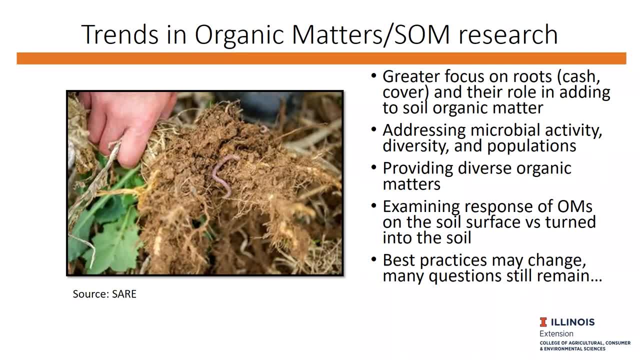 someone who really is interested and very passionate about soil biology and soil organic matter. it is a great time to be observing a lot of this research. there's a lot of new information that's been coming out in the last couple of years and we're seeing a lot of great information to kind of guide the small farmer. 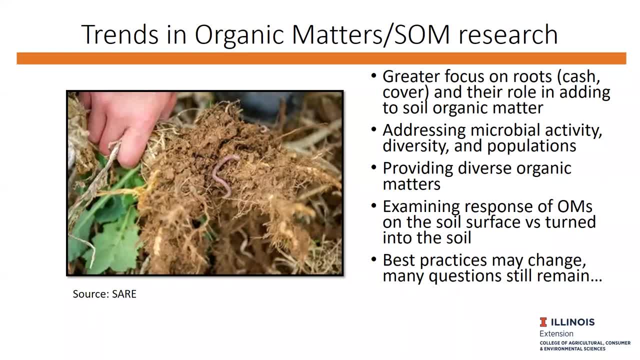 and these growers when determining how to better address your soil health and to really address the soil organic matter. as i've looked through and kind of looked through some of my resources this last week, you know what we started, have started to see, is a lot of greater focus on roots, meaning that 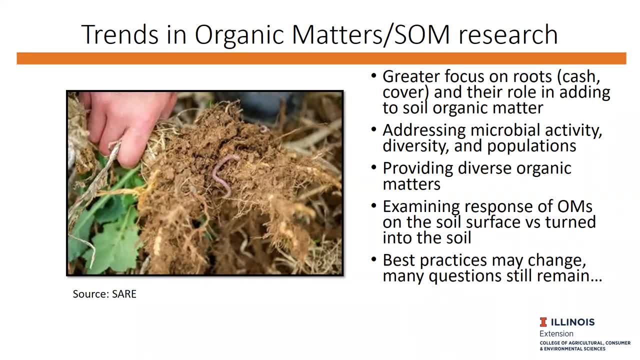 these roots from organic matter, like a cover crop or even say from a cash crop, are already growing in the soil and these roots are just covered in microbial communities that are getting root exudates and sugars off of these groups and when they start to decompose the cover crop, you know. 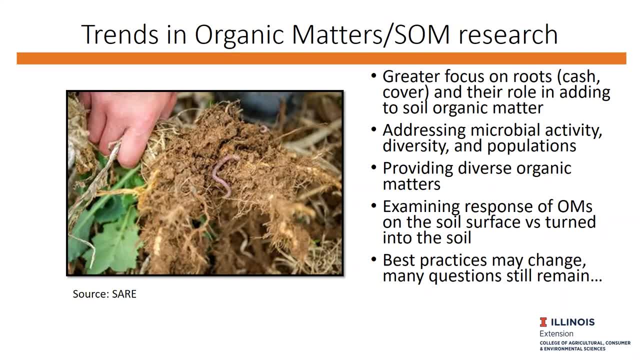 dies, or your cash crop you're done with. the roots are already in direct contact with the soil and they're breaking down pretty well, and so that is where we're starting to maybe see more organic matter research occurring, and a greater focus will be on the root systems of these organic methods. 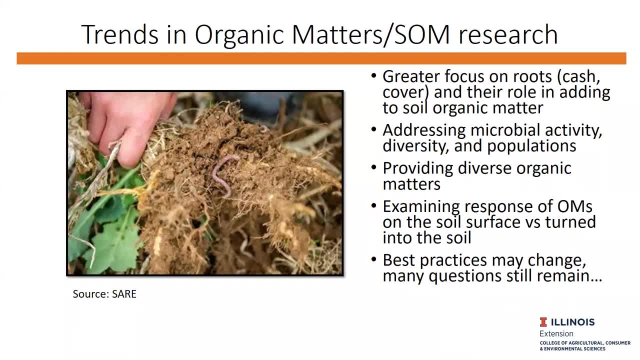 sorry, guys had a phone call um stacy, i'm on a conference call, okay, sorry cheese. um, they're providing diverse organic matters. they're examining responses of organic matters on the soil surface versus turned into to the soil surface. so i'm going to go ahead and talk a little bit more about that in just a few minutes. 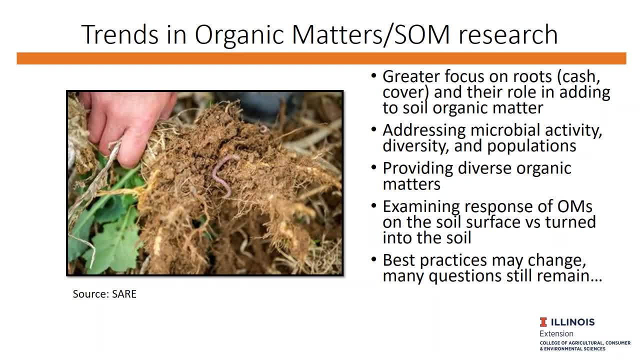 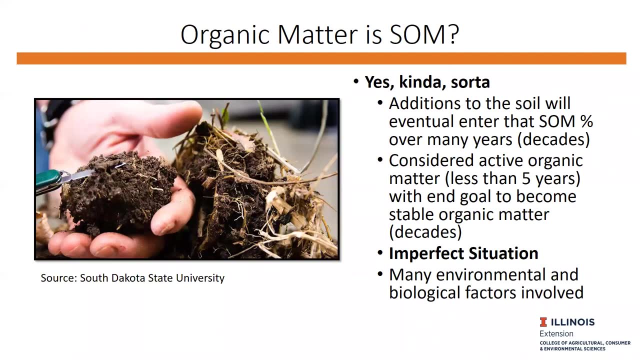 um, all that being said, you know best practices may change, but still many questions still remain. there's a lot of things that we're still trying to find out more about when it comes to organic matters. so, uh is organic matter? uh, soil? organic matter, yes, yes, kind of soil, it's a fresh ingredient. 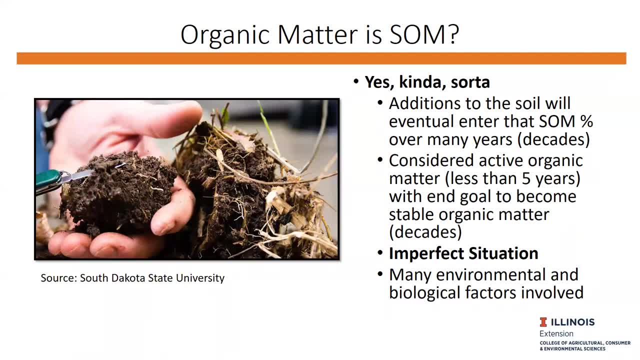 you're adding on a yearly basis. it's eventually going to get to that soil organic matter, but know that it's going to take decades. it could take, you know, three to five years to just finally be breaking down and start moving to the next step, but you still could have decades for it to actually 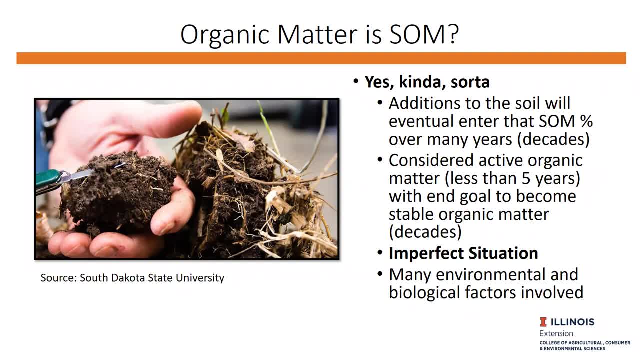 get to that end goal: soil organic matter. it's considered active organic matter. you know this is something that's less than five years that you have added to the soil. um, the end goal is, of course, to become a stable organic matter which, as i shared, we could take decades. it's a very 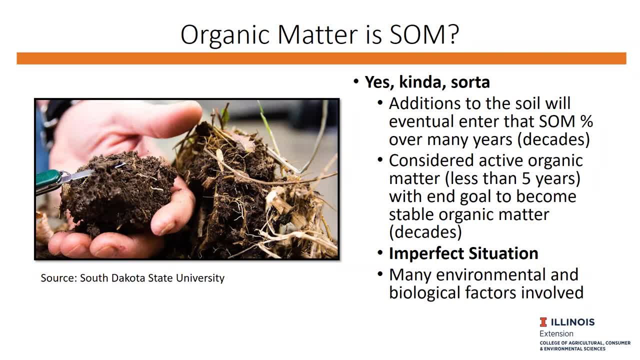 imperfect situation, though, depending on how the organic matter is added to the soil, if it's out on the soil surface, depending on your soil texture, your soil properties, the environmental changes, environmental conditions- all of those are impacting the organic matter that you're adding on a seasonal basis, eventually giving to the soil organic matter. so there's a lot to be. 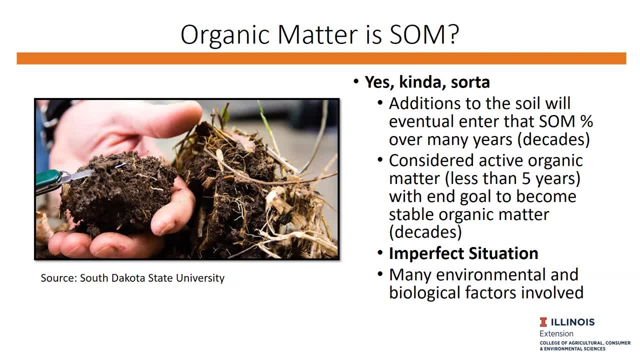 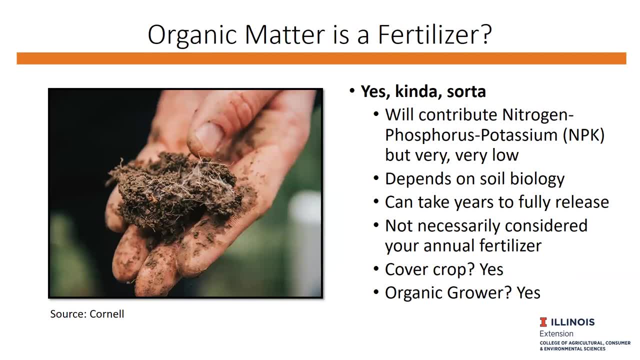 to still research and a lot to still find out. is organic matter plants? uh, organic matter is organic matter. can it be plant fertilizer? yes, kind of sorta. it does have, in most cases, some npk value in nitrogen, phosphorus and potassium, but what we really see is that organic matter has a very, very low npk value at this stage. 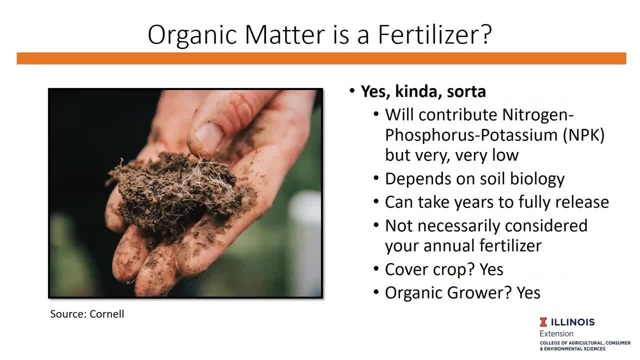 and sometimes that mpk value isn't just available yet for my plants to take up during that season, especially for an annual plant. so it will have some but it may not be enough. really, i think if i can get you on that seasonal basis, A lot of it still depends on soil biology. It's also important. 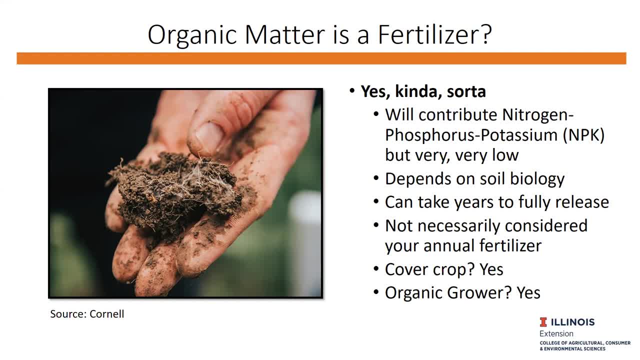 to recognize that it can sometimes take years to fully release all of that NPK value of that particular organic matter. Some of these can be easily released- the NPK values pretty quickly in a season, but some of them can take quite a bit of time. Don't always consider these your. 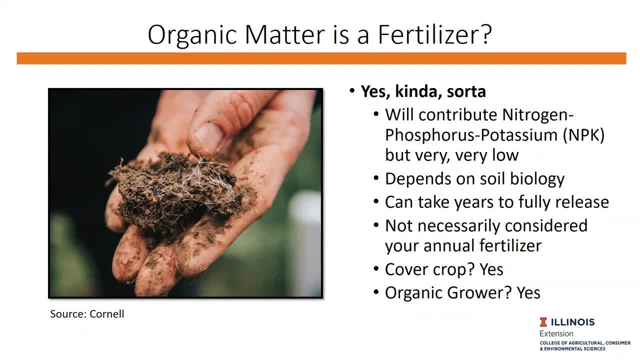 annual fertilizers but recognize that they will address sometimes nutrient issues with it. If you were to grow a cover crop that is an organic matter in most cases, some of them will have some nitrogen, especially if it's a leguminous cover crop, and that will address 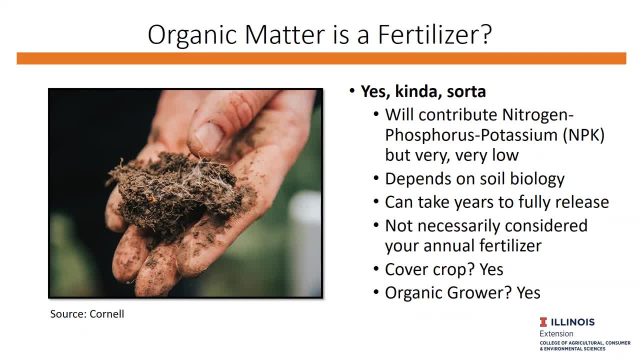 sometimes your soil fertility needs in that season Some of our cover crops will actually scavenge for nutrients further depth of the soil and bring up to the soil surface. But certainly you know you have to kind of figure out which ones you're growing in that situation. 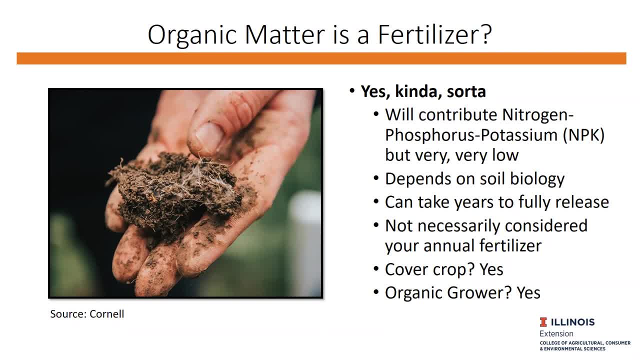 If I was an organic grower or pursue an organic certification or wanting to use some of these practices, you are depending quite heavily on the organic matters to be your fertilizer and to be providing those nutrients on a seasonal basis. That's just kind of what we really see. 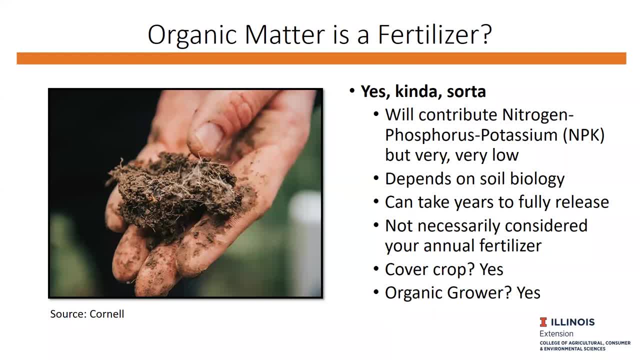 And yet again, you know you're still kind of reflecting back on what your soil test is telling you Over time. if you were continually adding organic matters, you would find that the soil tests may be able to really help you to kind of ease. 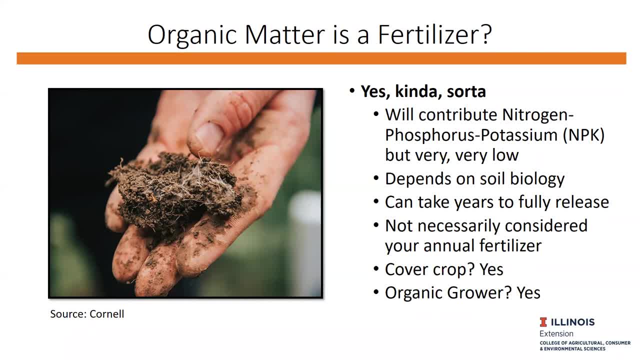 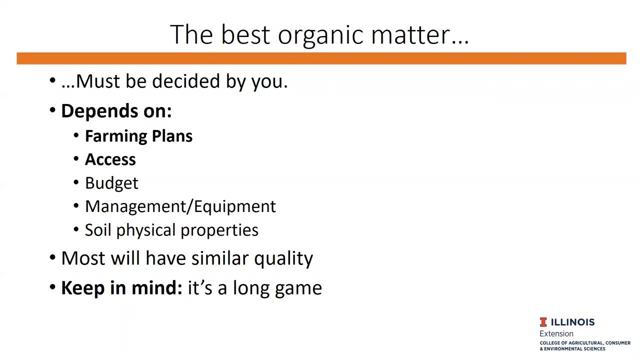 back on some of the annual fertilizers that you may be using. I get this question quite a lot. You know what is the best organic matter for me? Folks will say: you know, I tried this one. What about this one? What about this one? 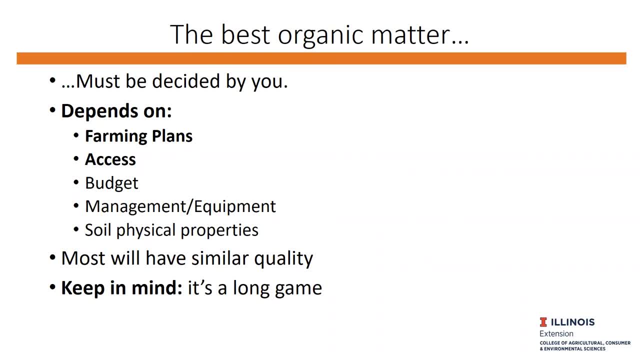 You know, I've even mushroom compost versus compost made from worms. You know it's a great question question, but i really think it has to be decided by you. i think that, depending on what your situation is, sometimes the best organic matter is the one that depends on lots of things. it could be. 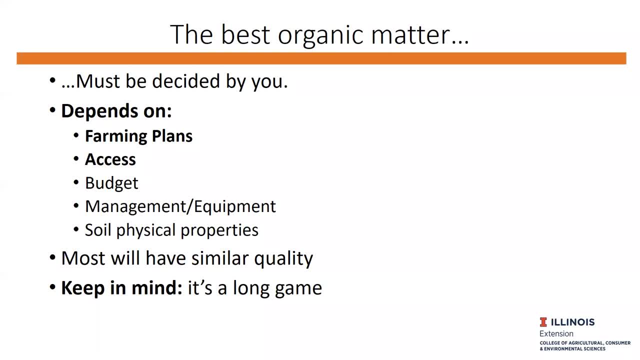 your farming plan. you know what are your long-term plans when it comes to growing fruits, growing vegetables, growing other other crops with it, and you may find that organic matters fit in well with some of these and some of them don't, when we think about, say, some of our perennial fruits. 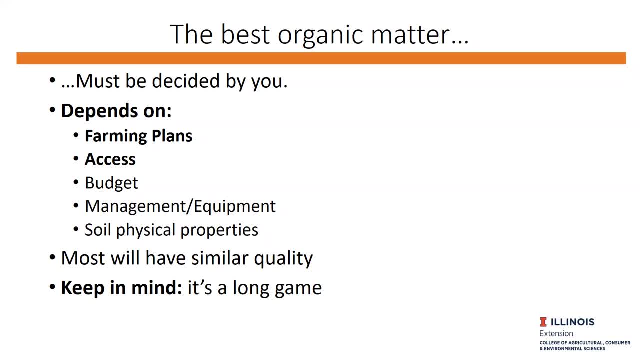 perennial berries, for instance. an organic matter for them is going to mostly look like wood chips or wood mulches that are on the soil surface, versus maybe an annual vegetable planting, where we would then see more of compost aged manure cover cropping systems that fit in well with this. i also encourage you to think about your access. you know some years you may have. 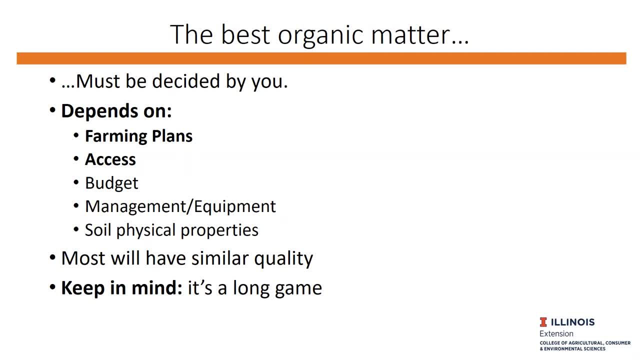 access to manure that you didn't have previously, or maybe you have. you know a couple of growers in your area and they have all kind of come together to purchase cover crop seed. so now you've got access to cover crop seeds that you didn't have otherwise. with it. budgeting can also be a factor. 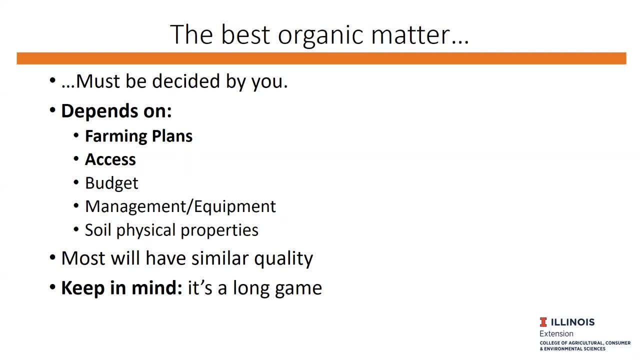 in here. you know thinking about what the budget from the yearly basis looks like for utilizing organic matters in that situation. keep in mind also management and equipment, and i think this is especially important as we think about growing our own organic matters like cover crops. you may want to have the right equipment and the right ability to manage the leaves when it comes to 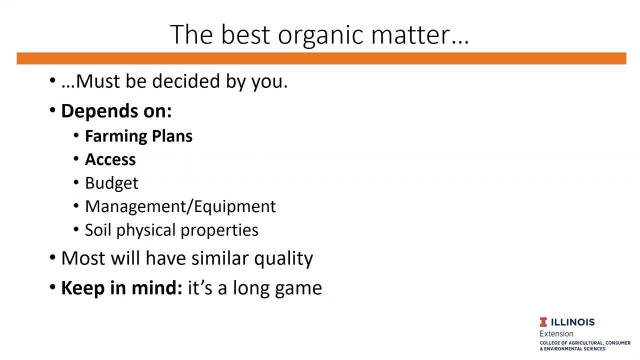 the cover crops you're planning to grow. in addition, you might look a little bit at soil physical properties. some of these organic matters may worsen a compaction issue that you may already have and not allow for as much good air flow and water exchange as you would like, so that 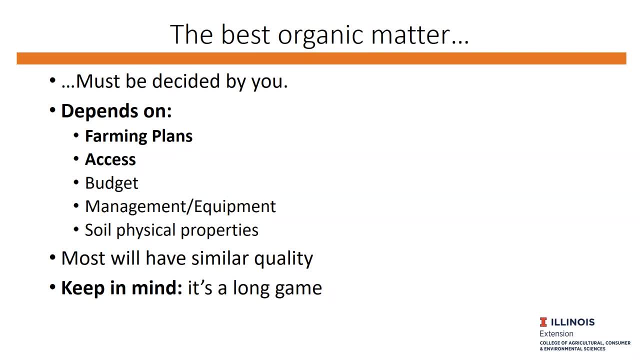 could sometimes be a factor within this. what we do somewhat see is that most will have pretty good quality, especially as we think about, you know, a compost or a manure. if you know you're debating which manure to choose, you will find some fairly similarities with the quality of it. 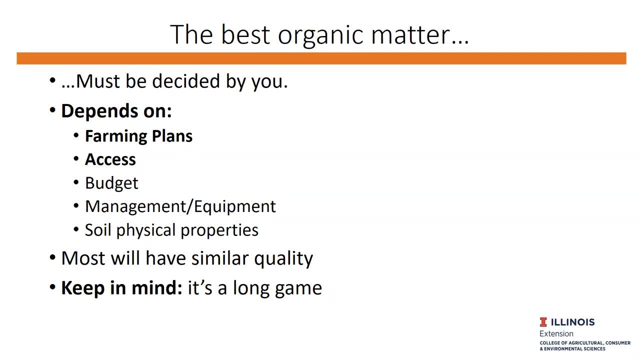 the same with your compost. compost will look a little bit similar to it too, but i encourage folks to really think about the long game here. you know, really you're thinking about diverse organic matters and adding a diverse amount of organic matters uh, throughout your farming experience. if i was adding compost last summer, in 2019 i might be looking to do a different organic 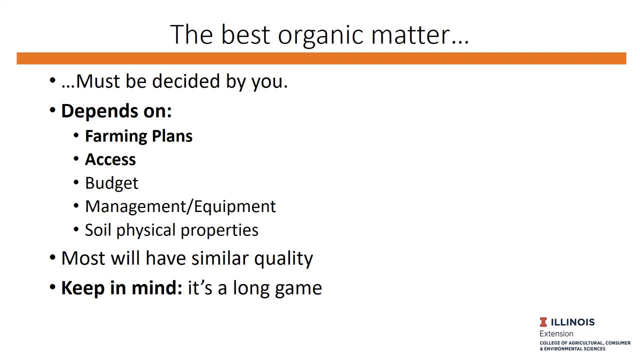 matter this upcoming year and potentially another different organic matter next year, and i would think that this is also fits in well if you think about some of your long-term crop rotations. factoring in sometimes. what your organic matter rotation could look like within here too, would be really great. we're not at a point just yet to be able to say that. 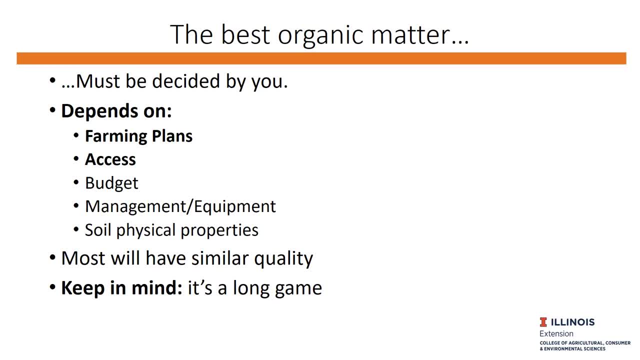 this organic matter should be followed up, followed up with this organic matter, followed up by this organic matter on a yearly basis. but i think we might be getting there at some point as we discover more and more about how the soil is responding and how our plants are responding to these biological 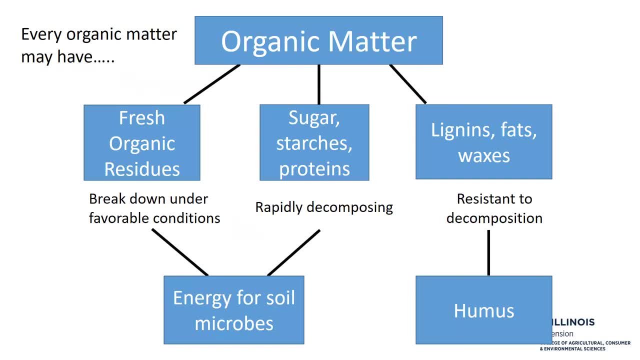 every organic matter that you choose and you utilize in your soil will tend to have many of these ingredients, so that you'll find fresh organic residues in compost, manure, uh, sometimes even some of our cover crops. you'll see this. sugar starches and proteins will also sometimes be in the organic matter that you're choosing. and then, for kind, 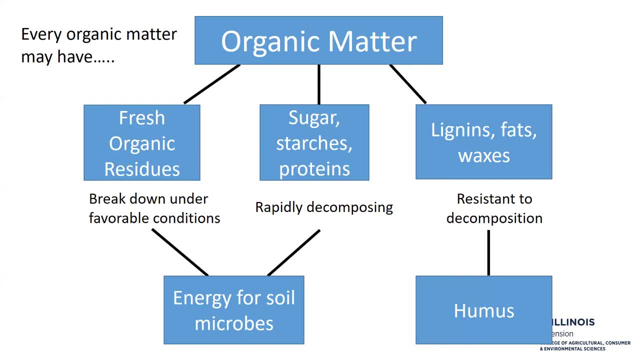 of woodier plant material we've seen. we've seen lignans and fat waxes tend to be a little bit more in our manure, uh, instead of our other organic matter to do. the last category tends to be resistant to decomposition, so it's something that the microorganisms just don't tend to gravitate. 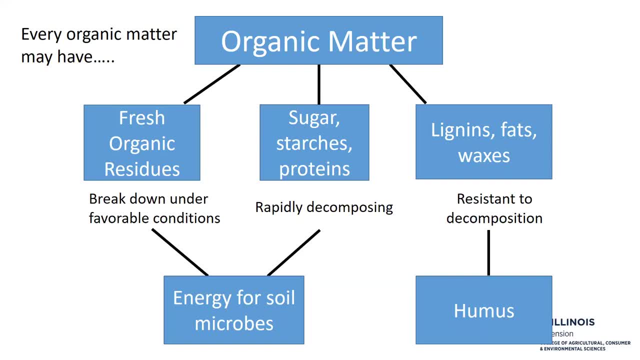 towards. you don't tend to like the organic matter that you're choosing, so that's something that we're going to look at annually as we start to think about our organic matter- and i think, rather than the organic matter itself as a separate category- is a really, really important one that has something. 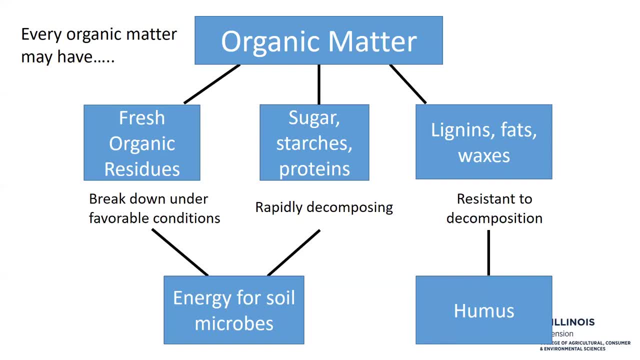 that we don't really like too much, so it tends to go straight through the humus itself. i would encourage you to really focus on these first two categories- your fresh organic bagel, as well as the sugar, starches and proteins, and that's you're going to find with. most organic matter is that? 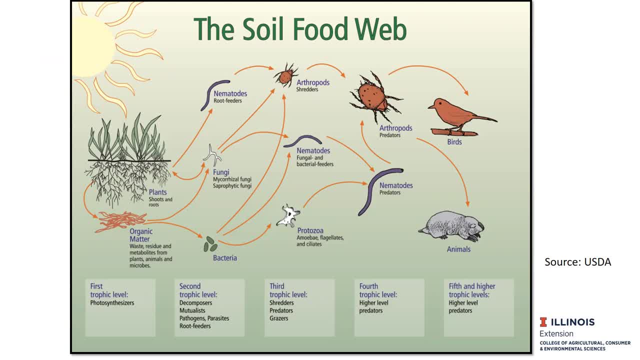 they will have these good products themselves. we have to kind of step back a little bit and think a bit about ecology. You know, in this way, as we're thinking about ecology, you know thinking about a forest food web or an ocean food web. 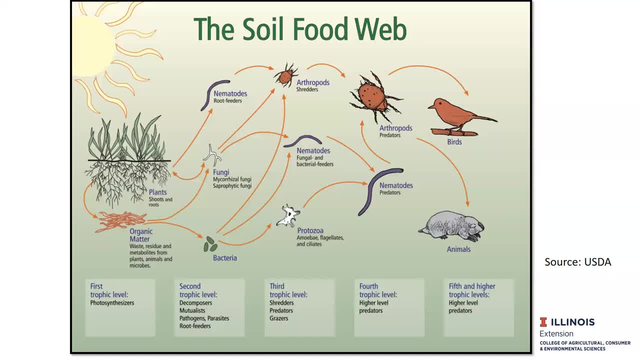 really we have a soil food web. You know, this is really what we see when we actually get samples in the soil and we actually look at the soil itself. Around the plants we have a lot of soil biological activity. The funguses, the bacteria, they're all kind of hanging out in these root systems. 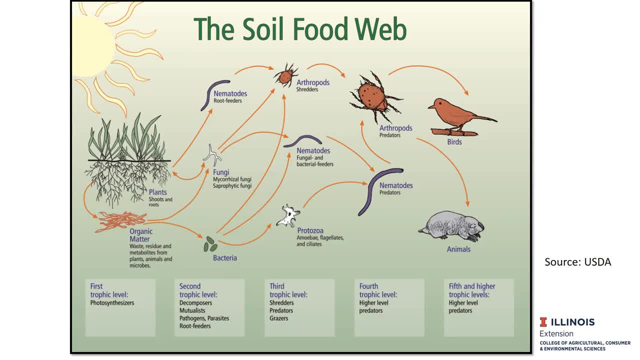 and they are kind of covering these roots and they're getting rid of pseudates and sugars and so forth. They're not attacking the roots, but they are actually giving some kind of food from these roots. At the same time, if you add organic matter, 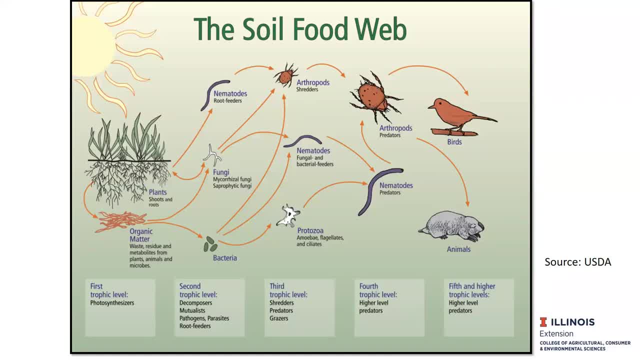 such as compost, manure and so forth or any plant residues that break down. that's also acting as food for this kind of first level of nematodes, fungi and bacteria, which are starting to eat, starting to decompose. 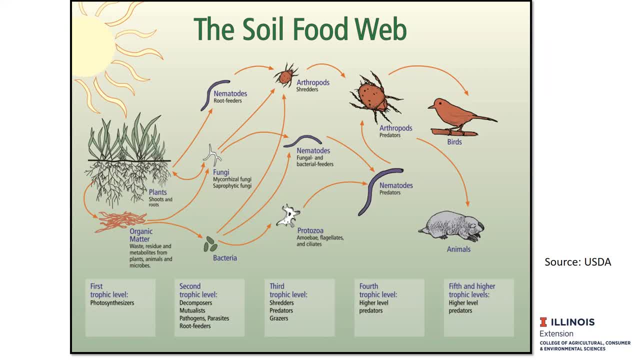 and as their populations get bigger, as they reproduce, we then have our predators that move in, such as protozoa, nematode, and they will then consume and eat their prey and it gets bigger and bigger and bigger. at this point, you know. 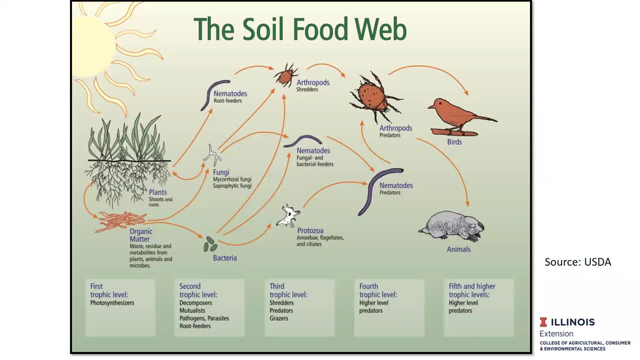 when we have bigger predators that move into this system. So this is really what's happening. you know, when you add an organic matter to the soil or when you actually have plants growing in the soil, is that this is happening. You know, the soil food web is. you know, it's just. you know, it's just. you know, it's just. 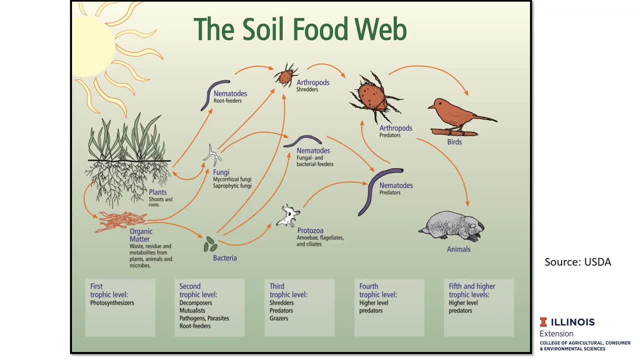 it's occurring In a perennial system where the plant roots are stable and you're not changing it. this soil food web tends to be pretty closed. You know, we tend to maybe see some fluctuations of these microbial communities versus an annual system where we may see some fluctuations depending on the season itself. 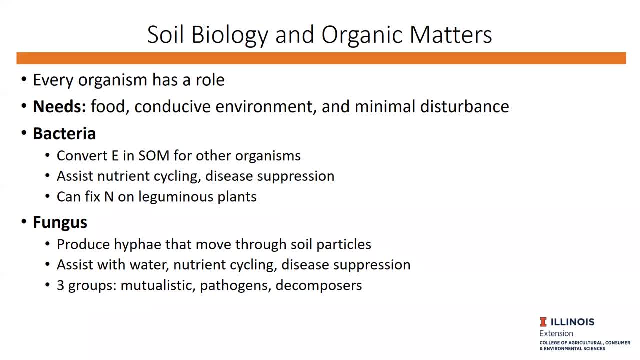 More about this, then. Every organism has a role. The needs of these organisms tend to be that they need food. okay, that's kind of expected. they need to have some kind of food source to eat. they need a conducive environment, something that allows for them. 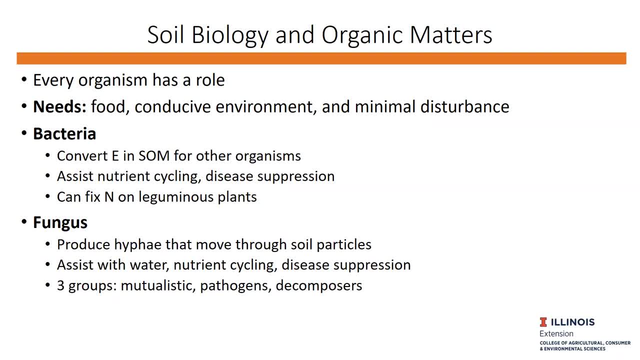 to reproduce, to respire, to grow and to eat, build up their communities, and then they also need a bit of a minimal disturbance- That's really kind of what they're after here- in order to kind of create and keep this soil. 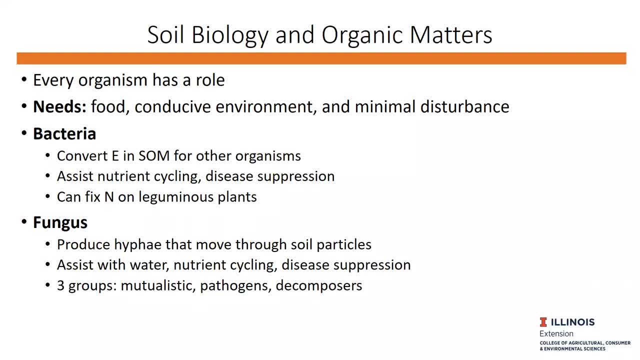 food web and their biological needs met. To share with you what some of the main ones do: Bacteria see converts energy into soil- organic matter. for other organisms it assists quite a bit in nutrient cycling, sometimes with plant pathogen disease, depression and soil. 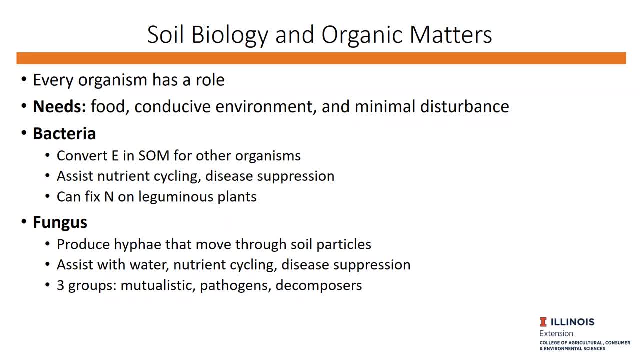 It can fix nitrogen on leguminous crops from the atmosphere Fungus. they tend to produce hyphae that move through soil particles. That helps quite a bit when it comes to kind of making sure that we're getting good airflow and water infiltration too. 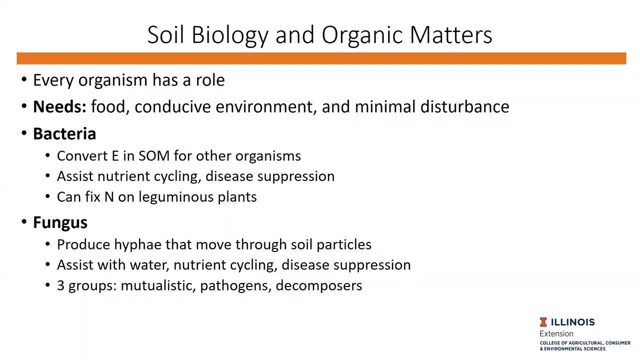 They assist quite a bit with water, Nutrient cycling, disease suppression. you have three groups of them: mutualistic, pathogenic or pathogens, as well as a decomposer. Mutualistic, you will sometimes see, is mycorrhizal. Most root systems on the plant will have some sort of mycorrhizal development which allows 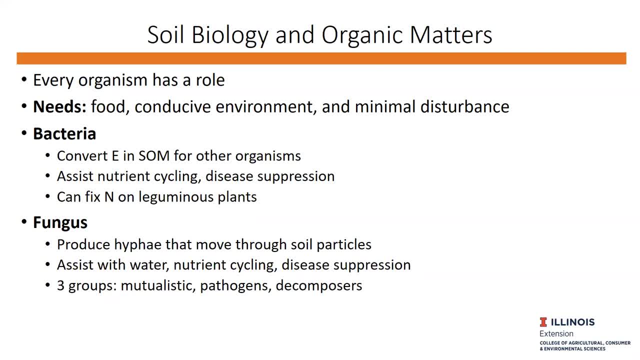 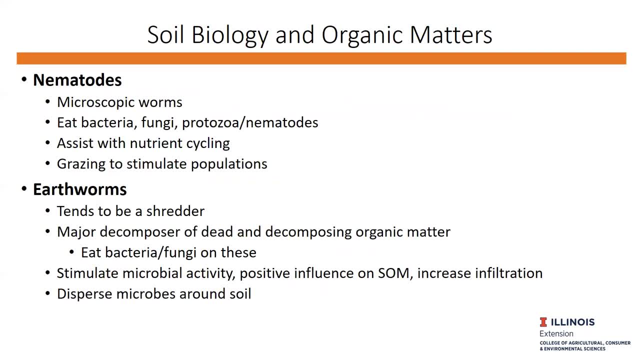 for that plant to have a greater surface area and allows for their roots to kind of go to and kind of spread out too. For nematodes, we have a lot of them, We have a lot of them, We have a lot of them. 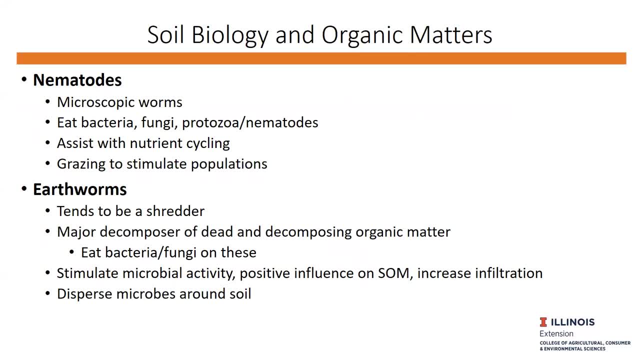 We have a lot of nematodes. These are, of course, microscopic worms that eat bacteria, fungi, protozoa and other nematodes, so kind of acting as a predator in this situation, When a nematode eats bacteria and excretes, this excretion usually has many of the soil. 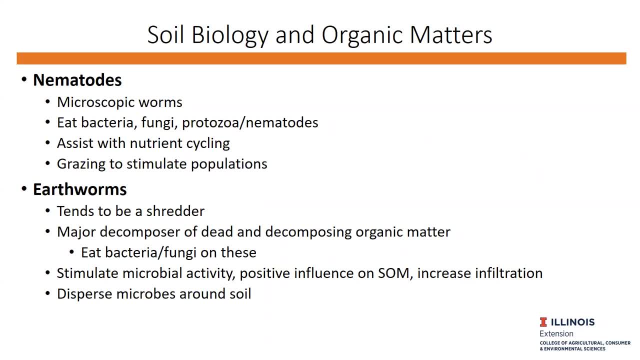 nutrients that my plants need. so it is kind of through that predation that we will sometimes have nitrogen and other things enter the nutrient cycle Through eating of bacteria. Grazing also tends to stimulate populations, so they will tend to kind of, if there is. 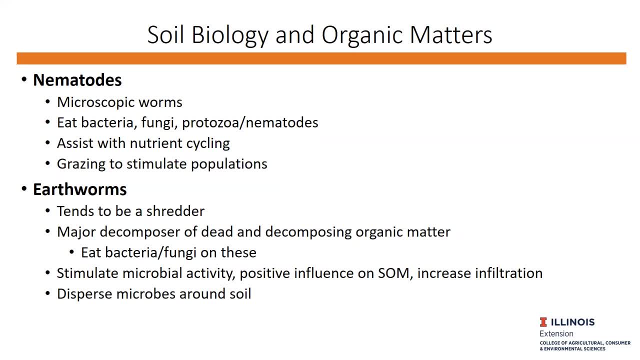 more food for them. they will kind of graze a bit more to it, especially with soil, biological use that might build up a bit more. Our earthworms and some of our other worms tend to be a shredder, a major decomposer. 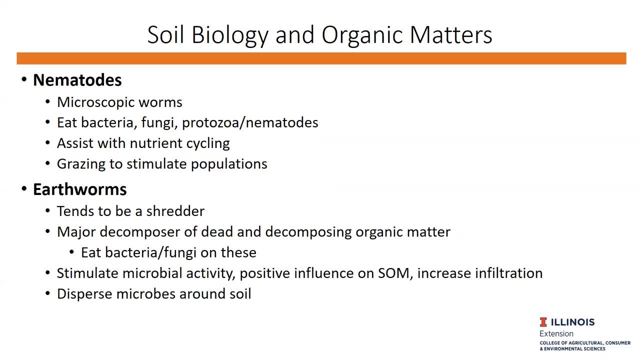 of dead and decomposing organic matter. They sometimes will pull organic matter above the soil kind of surface down to lower soil depth. Think of this a bit like if you have, say, a mulch on the soil surface layer. you may find that some of the earthworms are actually pulling down some of that organic matter into. 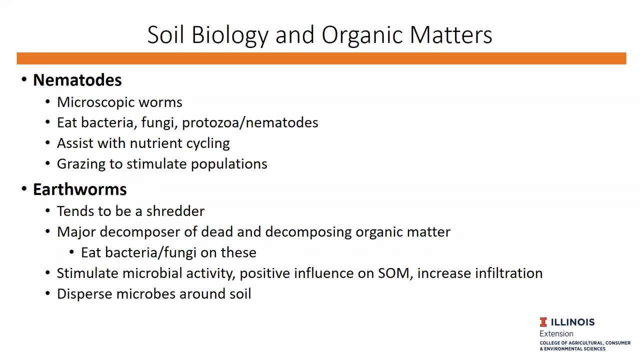 the soil to help it decompose so that it can also eat it too. They tend to stimulate microbial activity. they have a very positive influence on soil organic matter and, of course, also help a lot with water infiltration. Another thing they do is they tend to disperse microbes around the soil. 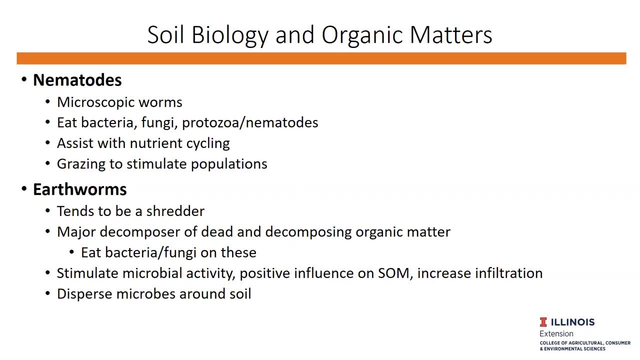 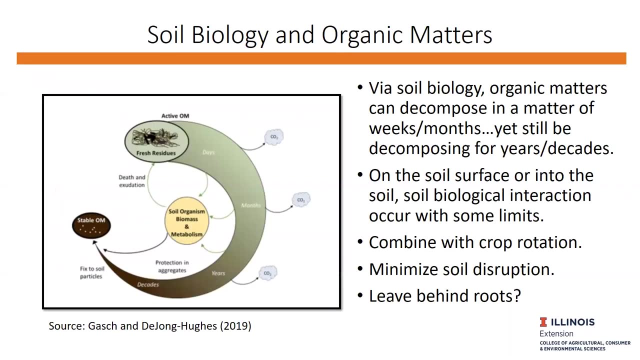 I tend to think of this that you know, a lot of our earthworms tend to disperse microbes around the soil. They kind of hitchhike on the earthworms, and as the earthworms are moving through the soil, these hitchhikers are also being distributed to it. 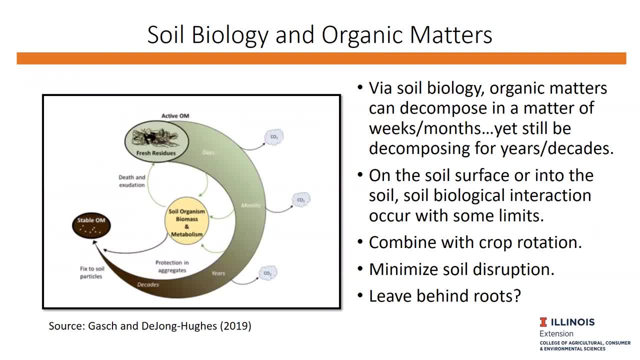 So via soil biology, organic matters can decompose in a matter of weeks, months, yet they can still be decomposing for years and decades. The photo that you see here kind of shows this in some capacity. You can see that there are fresh residue breaking down after days with soil organicism. 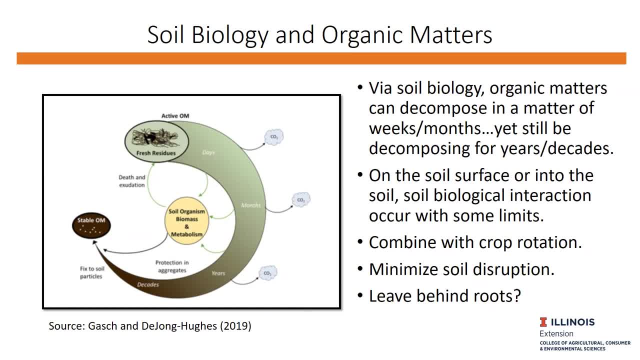 biomass and metabolism. After months and years, the same product is still breaking down, and then it could be decades before it finally enters the stable organic matter. Yet again, we are still losing some of this to the atmosphere. in most cases, If it's on the soil surface or into the soil, you may find some soil biological interactions. 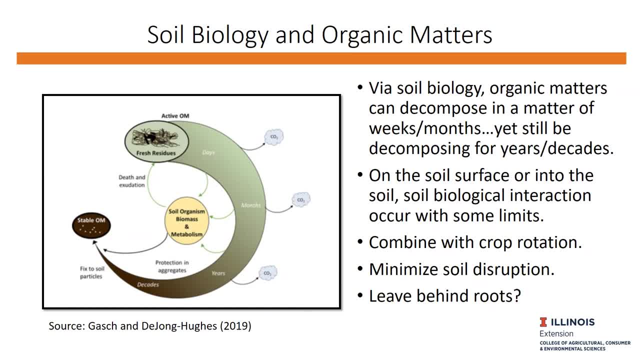 occur with some of the patients. We do tend to see that, you know, direct contact into that actual zero to six inches tends to be where a lot of biological activity really occurs. It allows for these organic matters to really break down. At the same time, I'd be remiss to not mention that having something on the soil surface 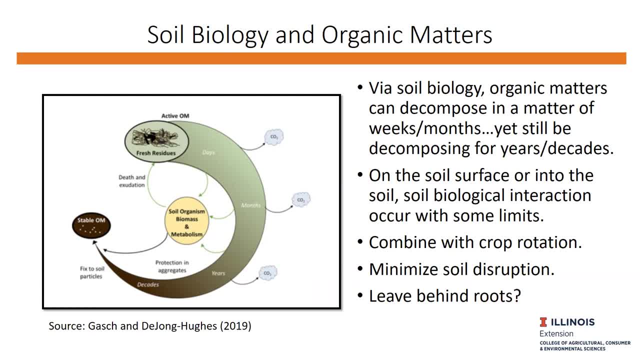 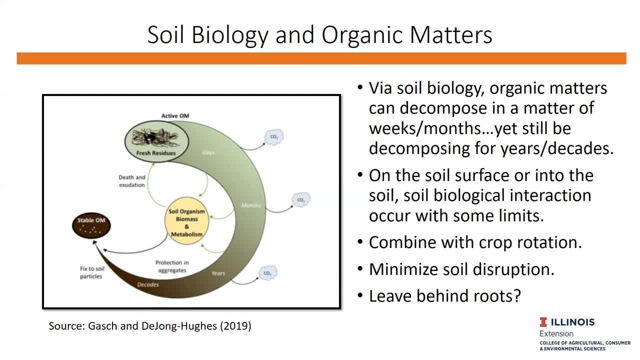 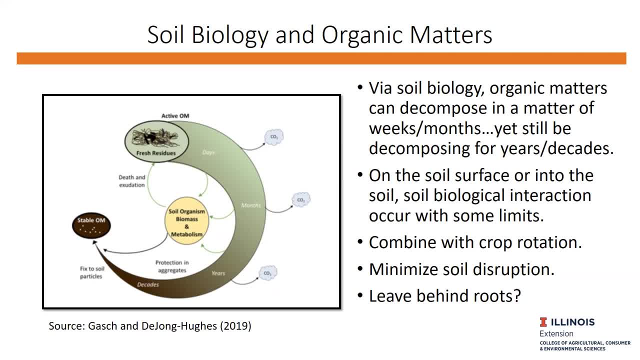 your growing area. it's going to help quite a bit with soil biological diversity, and that's something that I really encourage you to consider and think about. As I've shared with you today already, there's a lot of more interest in research on the. 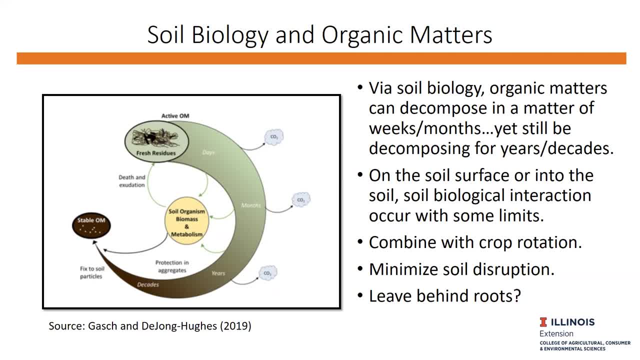 root systems and in thinking about leaving behind root systems of the plants you may be growing. If this was something that grew on the soil surface, I don't think you'd be able to consider and think about. You, of course, would have to really think if it fits in well with your farming plans. 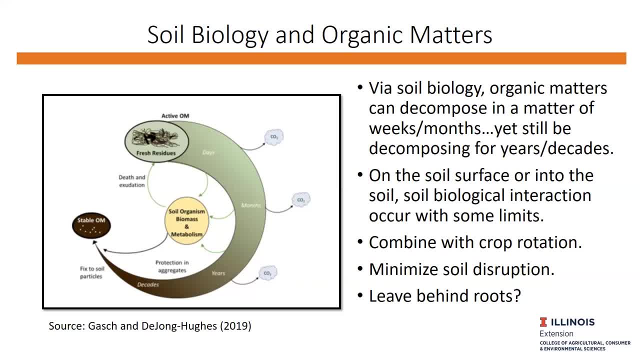 and you would still want to combine it with crop rotation and other systems. But ideally this might be something where at the end of your annual vegetable growing system season, you remove much of the crop debris, especially those that might have disease and other pathogens on it or potentially have them, and then you're leaving behind that. 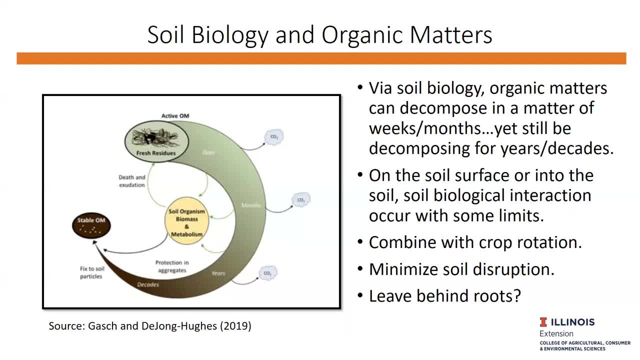 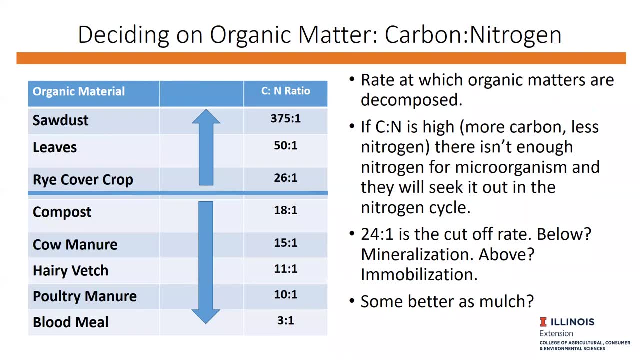 root system to overwinter and to just then break down into that next year. It's still a lot to be done, It's still a lot to be said with this and I'm not fully on board to yet just endorse it fully yet. but I think that may be where we start to shift some of our thinking. 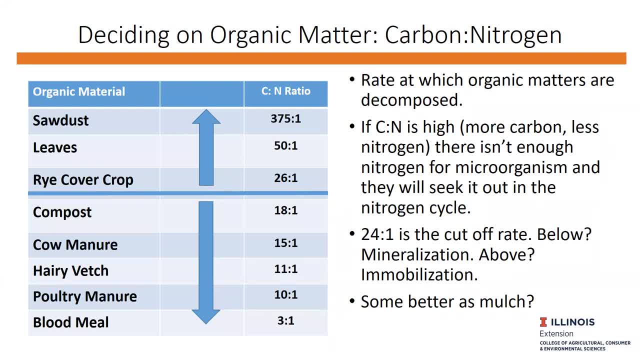 Another factor that you're going to have to consider is the organic matter, the carbon to nitrogen ratio, which you see here, And this tends to be the rate at which organic matters are decomposed If a carbon to nitrogen ratio is high. so they have, say, more carbon versus less nitrogen. 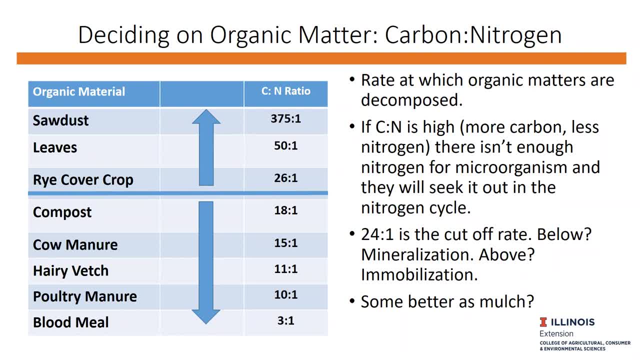 which you kind of see there with sawdust, a very high C to the N of 371,, 5.1,. there tends to not be enough nitrogen in that product for the microorganism to utilize and break down, So then they will then tend to seek that nitrogen somewhere else, typically from the nitrogen. 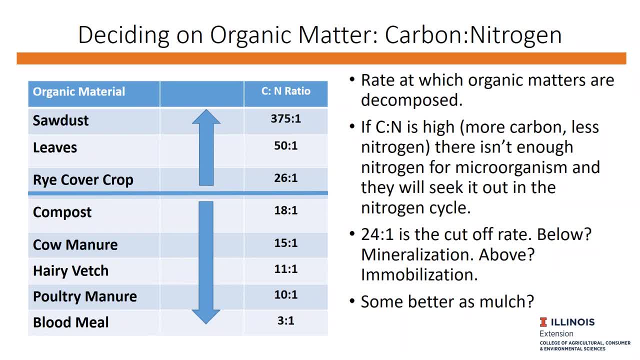 cycle that's in your soil system. So what that then means is that that nitrogen that would have been available for the plant is no longer available because my microorganisms- I've had to borrow it for a little bit of time. 24 to 1 tends to be the cutoff rate for microbial communities to use their carbon to nitrogen. 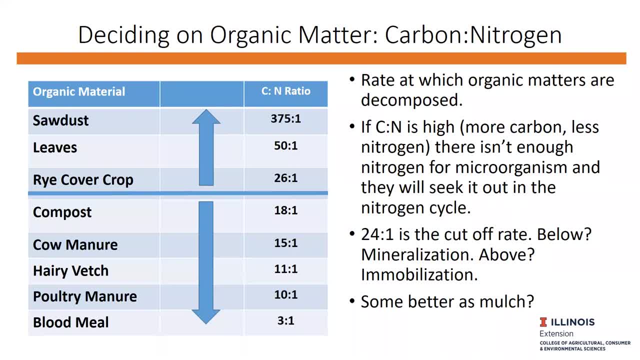 ratio Below, we just tend to see mineralization occur. Above it, immobilization occurs, And I'll talk to you a little bit more what this kind of tends to mean. At the same time, a lot of times the C to the N really dictates a organic matter that 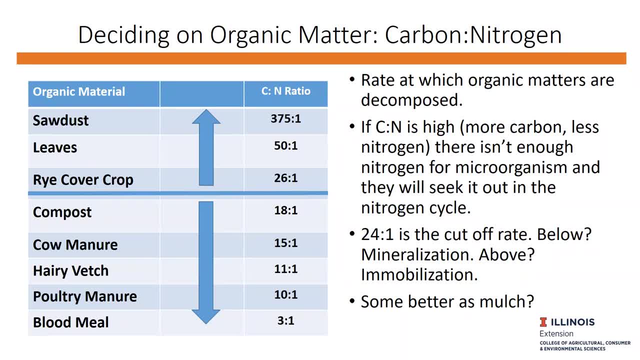 just may be better as a mulch, Because it won't, Because it wouldn't necessarily lock as much of that nitrogen away from my microorganisms and their ability to not connect my plants and their ability not to get it. You do see some common organic matters below this line of compost: cow manure, hairy veg. 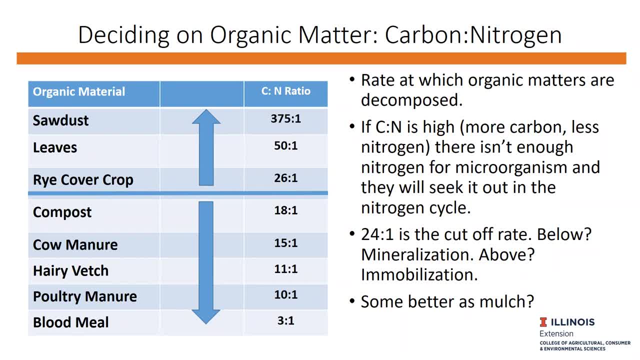 poultry, manure, blood, milk- all have much lower than that 24 to 1 ratio, And most of them really are what we consider organic matters that would break down into the soil and ones that we need to turn to the soil versus those that are really above. 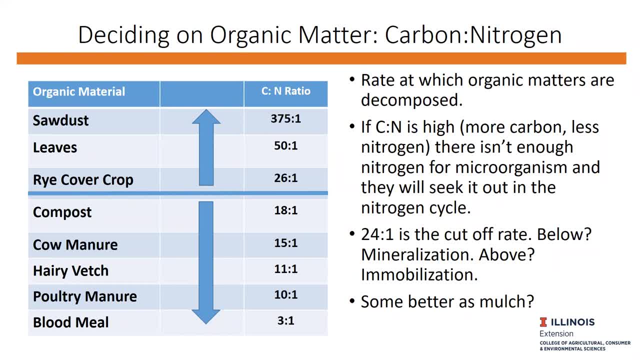 that line that tend to be more of a mulch on the soil surface level. It is a very common practice to combine, So to combine, say, a leaf with, say, your compost, So you are getting kind of a balancing out perhaps of these organic matters, if you are. 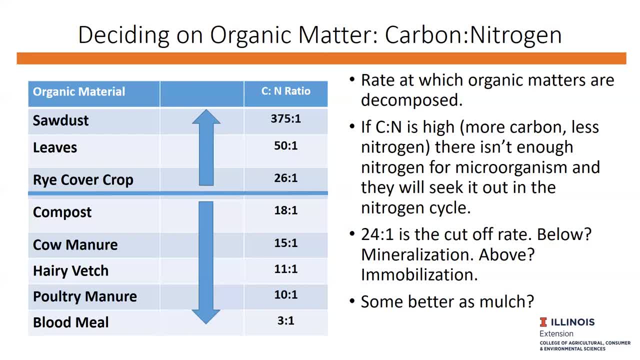 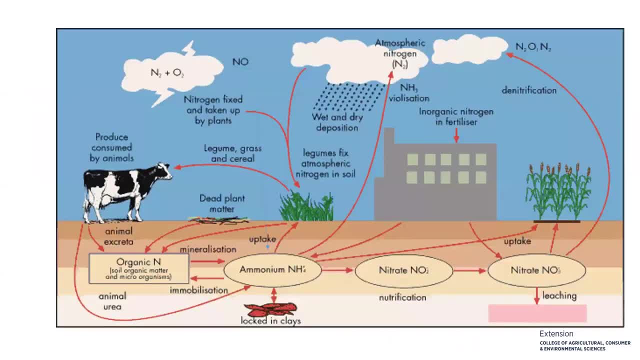 to use them Yet again. I think sometimes it gets back to your access and what is available to you and maybe what is not available to you. This is the nitrogen cycle. A lot of us have seen this before, But just to kind of mention kind of what you, you know, sometimes see here kind of within. 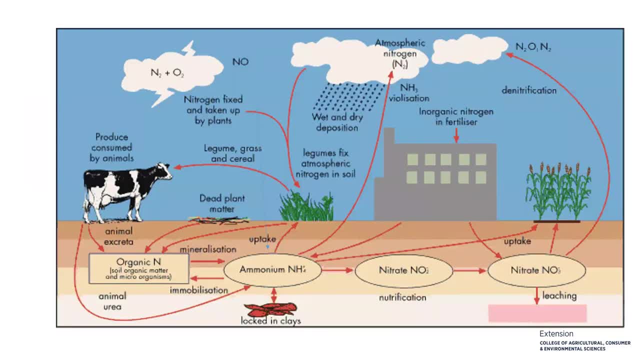 this organic N. You can kind of see kind of what I'm talking about here, where we have this organic N right here And this is that period- the mineralization or immobilization- where, depending on the C to N ratio, it may become immobilized. 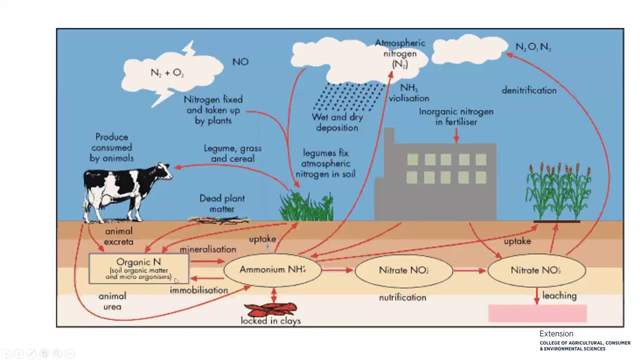 So it is being activated. So it is being activated, It is broken down, It is immobilized And it is basically kind of locked within this organic N versus a C to N that is below that 24, where, when it breaks down to the organic N nitrogen, you could further transform. 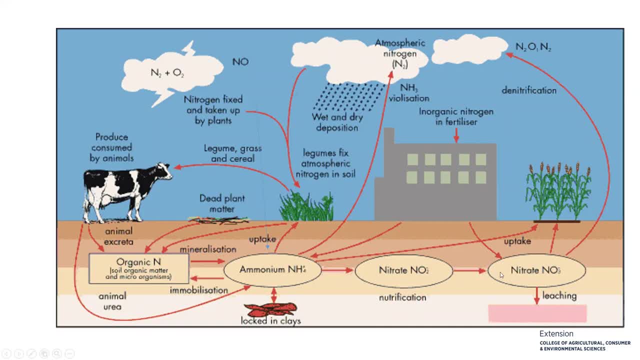 and mineralize to ammonium nitrate as well as that kind of potential nitrate system. It is not always a perfect system And we should be kind of upfront about that. You know, you may not have it as perfect as it could be. 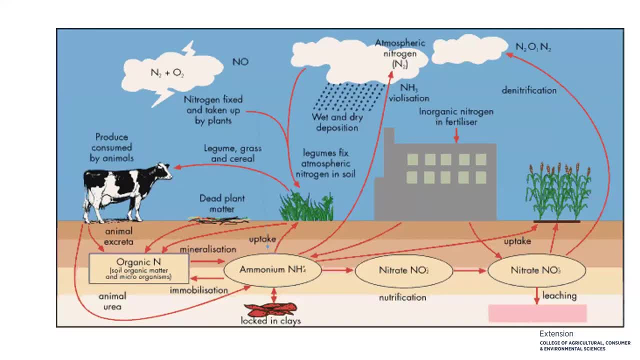 But that's kind of what you're looking at there and what the concern can sometimes be. If I was more of an advanced farmer and had been farming for a couple years, I would lean heavier and kind of worry a little bit more about this kind of C to N ratio versus if 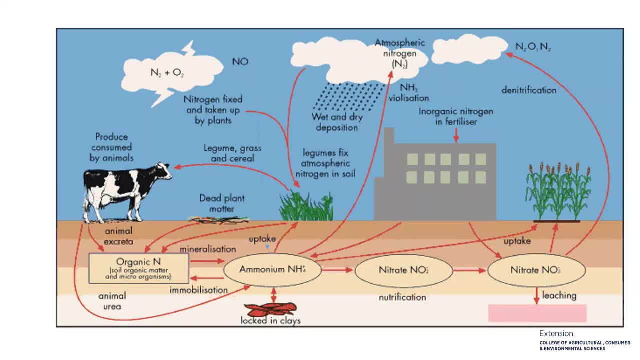 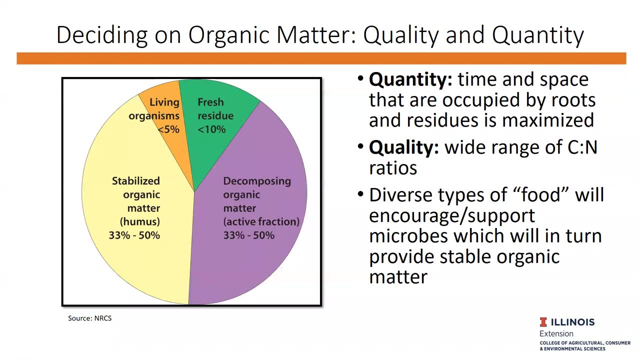 I was more of a beginning farmer, just kind of getting started. Another factor to consider here is quality and quantity. So quantity- is kind of the time and space that is occupied by roots as well as residues- is maximized, versus quality. We have a wide range of carbon to nitrogen ratios, kind of mixed in together to kind of 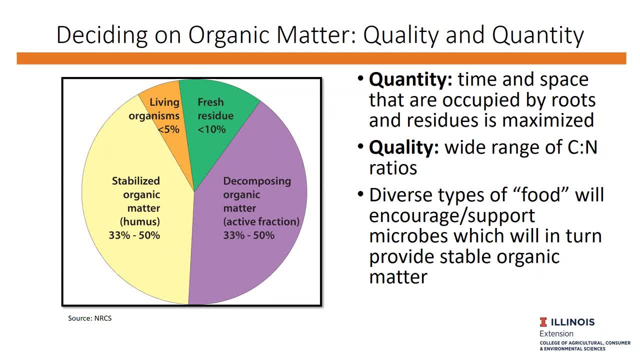 help quite a bit with this. As such, you know, encouraging diverse types of food will encourage, support microbes And that will in turn provide very stable organic matter that will address your soil organic matter. So it is kind of these factors. 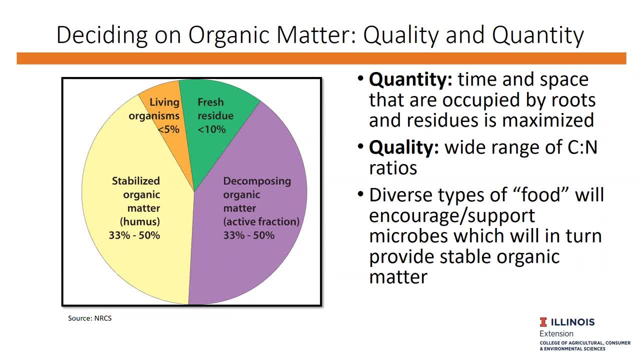 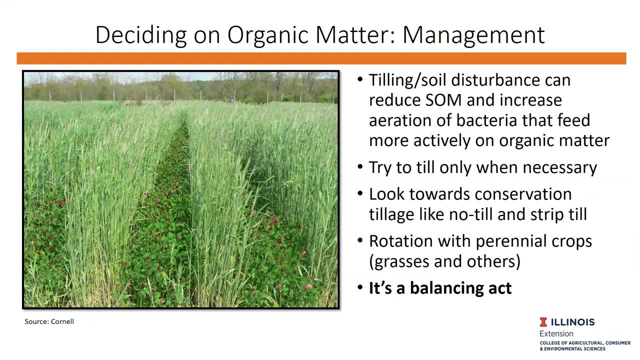 And you'll see this a little bit more when you think more about your soil organic matter. So it is kind of these factors And you'll see this a little bit more when you think more about your soil organic matter. A crucial step here, also with organic matter management, is going to be management. 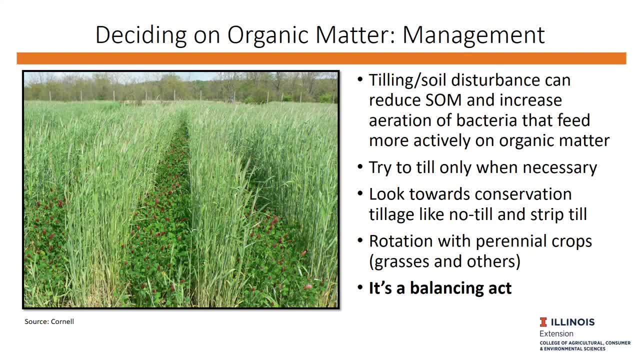 So what we do see is that tilling and soil disturbance can reduce soil organic matter And this can increase aeration of bacteria that will feed more actively on organic matter. So we could actually not get as much of that organic matter long term transformed into. 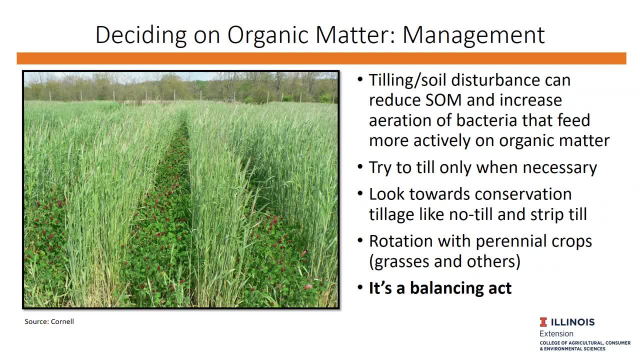 that stable organic matter that we're after. So that's a bit of a balancing act here, Because for a lot of these organic matters they do need to have some sort of soil contact And this disturbance in that soil is really crucial. But yet we still want to really think about, you know, trying to till only when necessary. 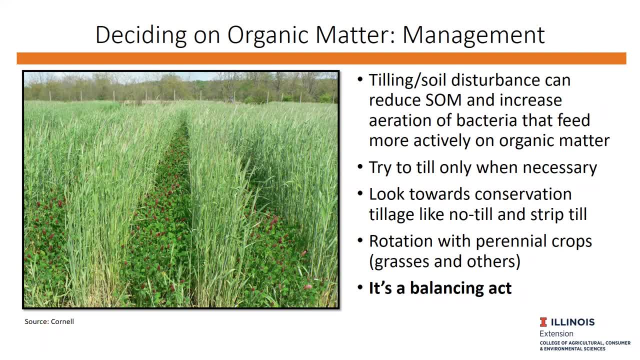 And you may look for conservation tillage like no-till, or looking for some strip tillage situations, as well as rotation with perennial crops. So considering giving, say, certain growing areas a bit of a break and allowing them to just have continual cover cropping systems on them and in place. 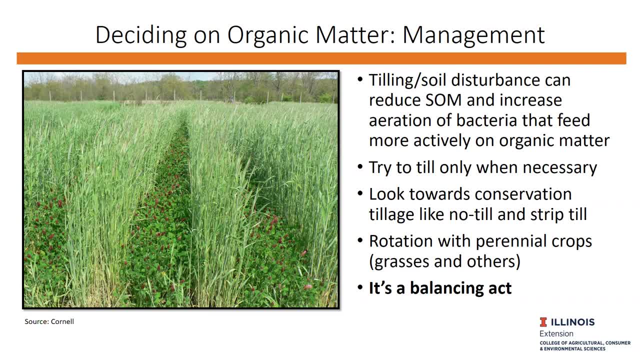 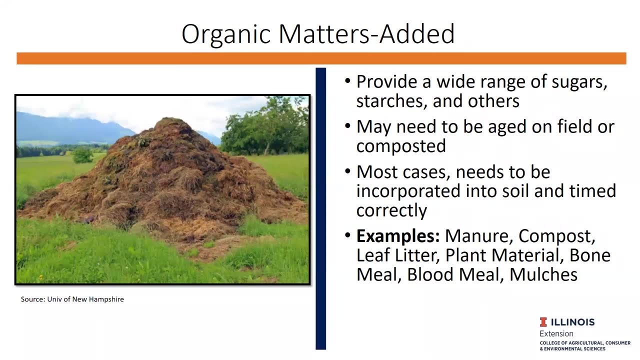 But, as I share with you, it's a bit of a balancing act And we are growing most of the annual crops that do require some sort of annual disturbance for us to actually plant these plants in that growing area. So organic matter is added. 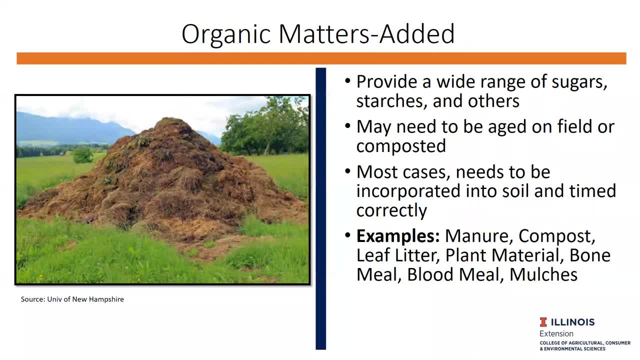 They provide a wide range of sugars, starches and other things- other products- in there. They tend to need to be aged on field or compost In most cases. We also need to think that many of them need to be incorporated to the soil and also consider 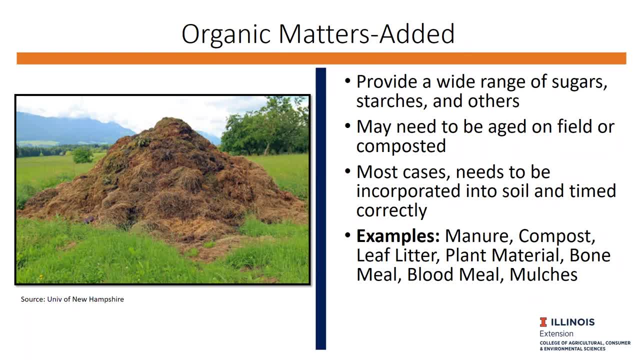 timing these correctly, You will find that sometimes they just need to be timed a bit more than other ones tend to do. This includes manure, compost, leaf litter, kind of any plant material debris. It also can include bone mill and blood mill, two of which have some pretty nice NPK values. 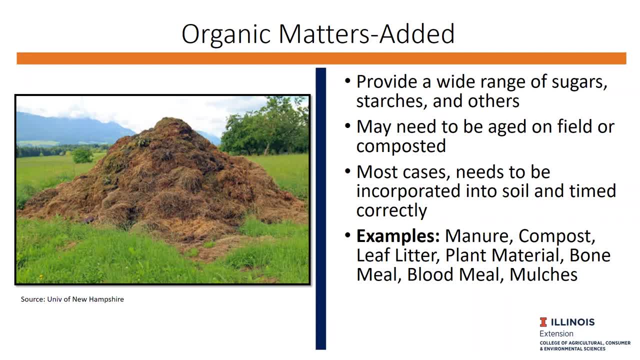 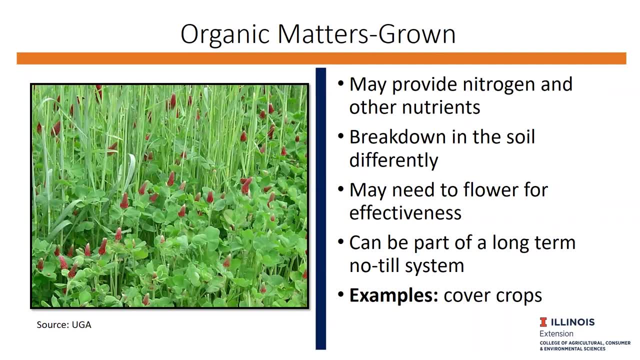 as well as kind of our common mulches. in this system too, These are your added ones. Cover crops are rather organic matter that are grown. They provide nitrogen and other nutrients. Nitrogen: if it is a little bit of a luminous cover crop, they will break down in the soil. 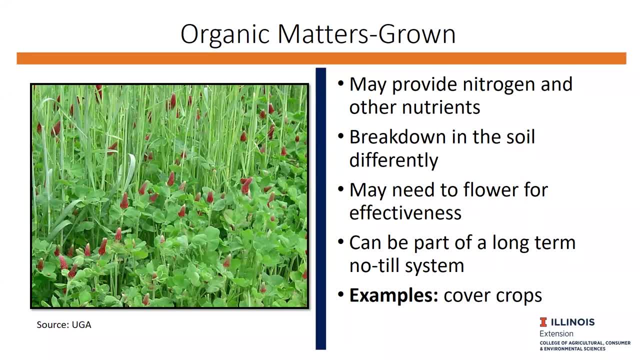 very differently, So you will have to factor in that carbon to nitrogen ratio a little bit when it comes to this. Many of them also need to flower for full effectiveness of getting the most bang for your buck. when it comes to utilizing cover crops, They can, of course, be part of a long-term no-till system. 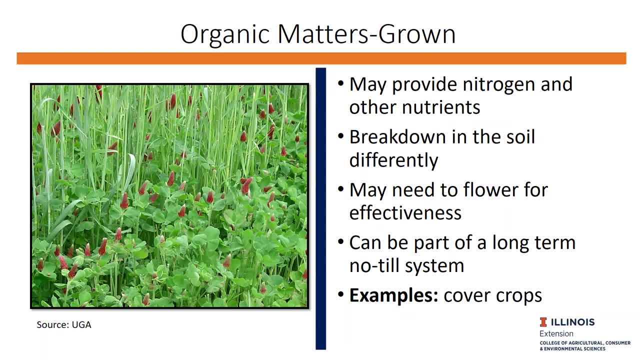 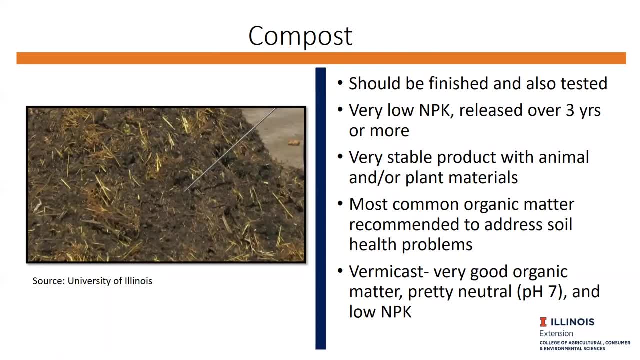 And you also want to think about choosing, Using a cover crop, like an organic matter that's grown, that can address your other soil problems too. So compost as an added organic matter, it should be finessed, It should also be tested. You know, of course, that compost has a very low NPK value. 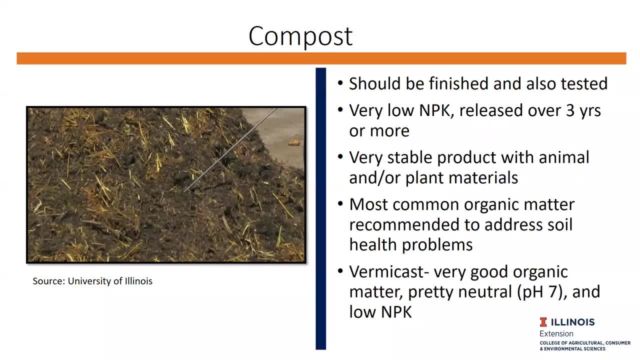 And this tends to be released over three years or even more. It tends to be a very stable product with animal and or plant materials, depending on the product that you have and the product that you might use. It also is sometimes the most common organic matter that's recommended to address soil. 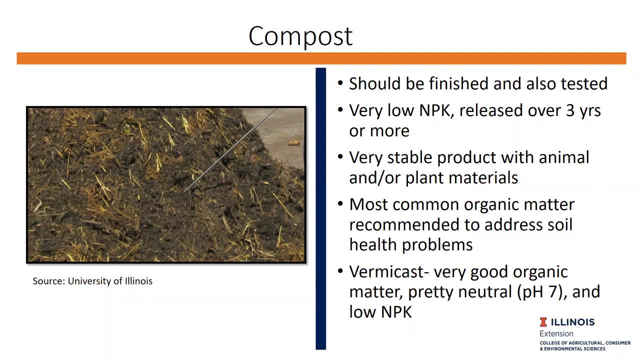 health problems. When folks have compaction problems, when they have other related problems with soil health, I tend to recommend some compost to hopefully address what some of them are. You commonly see vermicast or vermicompost made from earthworms. 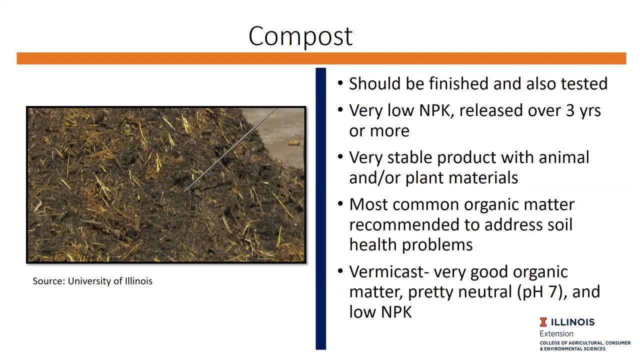 It can be a little bit expensive. Know that it is a very good organic matter, Pretty neutral, with soil pH of seven, But also, like other composts, a very low NPK value within it. So yet again, you know, just kind of be a little cautious- that it should not necessarily. 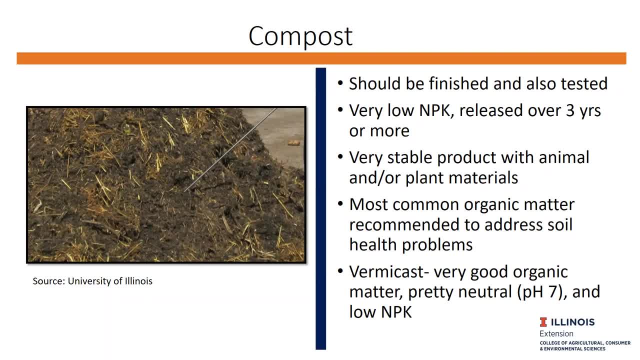 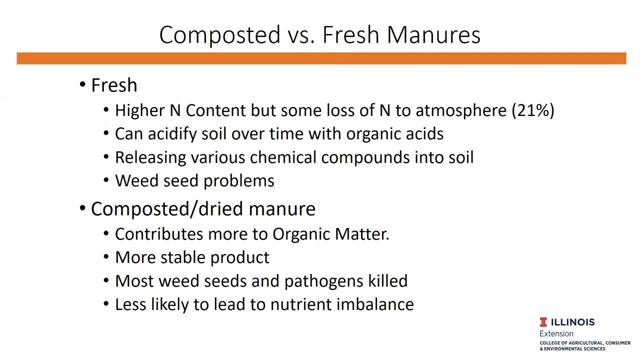 be your annual fertility fertilizer needs, just because the NPK value is going to be very low For manure. you're going to have kind of two broad categories. You'll have fresh and you'll have composted or dried manure. Composted dried manure: you may also see that it's called aged manure. 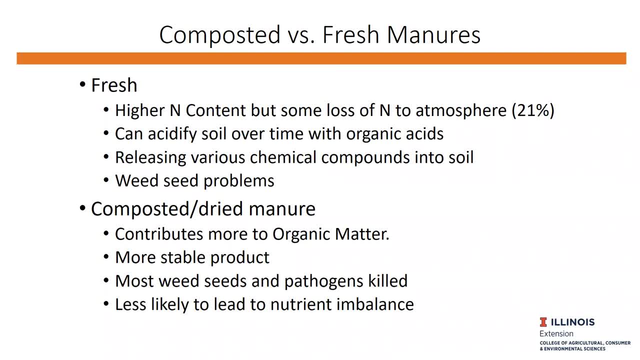 That's kind of a common term too- A fresh manure typically. we see you know higher nitrogen content, but we lose a lot of it to the atmosphere- about 21%. It can also acidify our soil over time with lots of organic acids that are broken down. 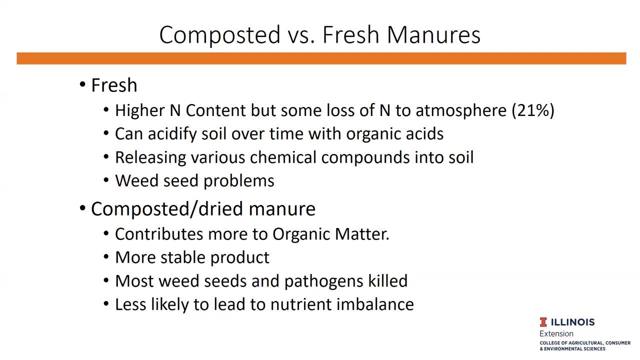 through the soil. Be a little cautious of that. In most cases, our vegetables do need some acidity and need to be grown in acidic conditions. They can release various chemical compounds to the soil. I should clarify here that I'm talking more about still yet again, organic acids. 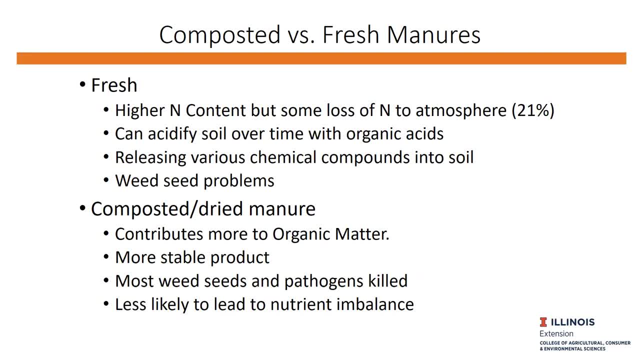 Also- I'm not going to go into all the details here. They can also can cause some kind of a material change, But again, just the fact that you're growing here in this particular world. there's absolutely no danger that you're going to have change or you will never be able to see another soil. 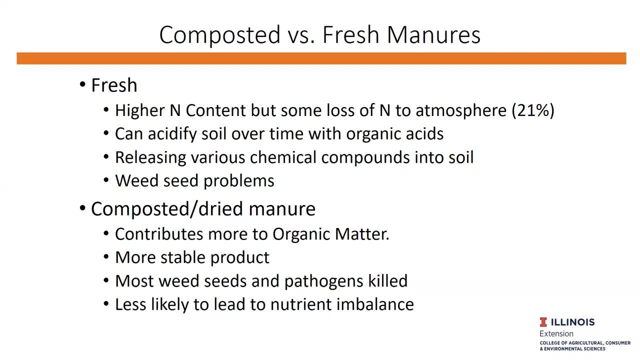 and nutrients that would eventually go into there or nutrients that will go into the soil nutrient cycle. Some of them can also have substantial weed seed problems. especially coarse manure- It tends to have a lot of weed seeds in it. The composted, dried manure, aged manure- it tends to contribute more to organic matter. 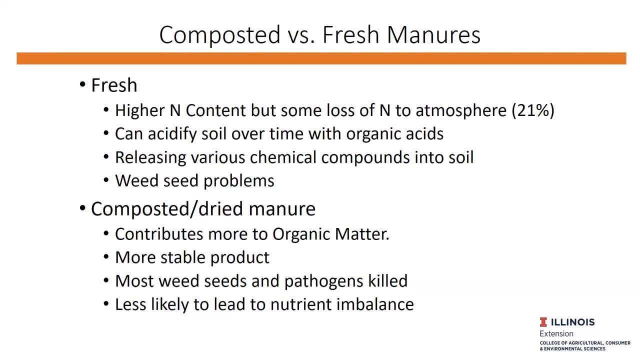 as it's already kind of a stable condition, or you have used it in making your compost, and so it actually is one that can just be pretty, pretty neutral with it. We do tend to see a lot of natural samples of organic matter, but I don't think we're 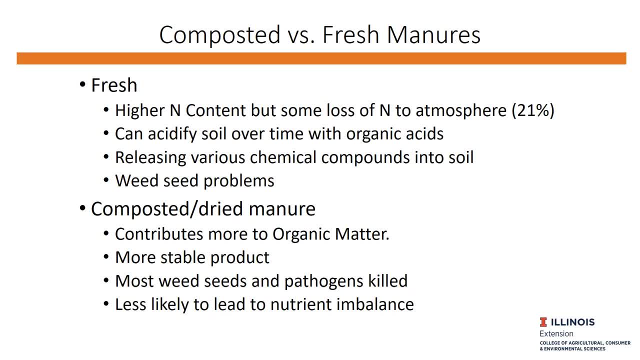 going to see that here most weed season pathogens are killed. this is especially true if you're. you are making manure into compost and you are taking temperatures to ensure that it's getting to that right temperature. to ensure this, it tends to also be less likely to lead to a nutrient imbalance as well. 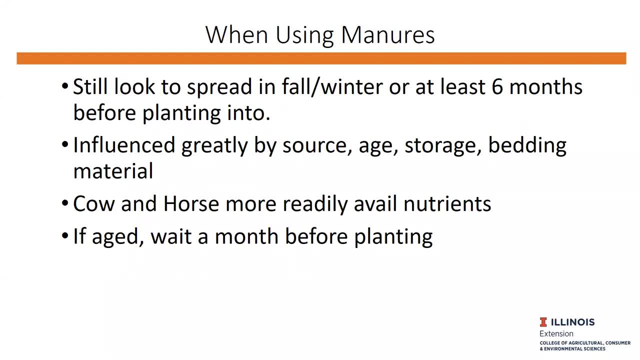 when using manure still look to spread into the fall, winter or at least six months before planting into it. it can also be influenced greatly by source, age, storage, bedding material. all that goes into factor when it comes to utilizing this manure. cow, horse tends to have. 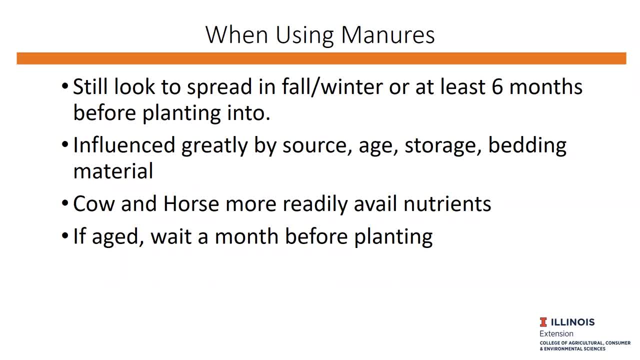 more readily available nutrients. even if it was an aged manure, i still kind of recommend a month before planting. the reason for this is i think you just really need to give your soil biological community a month to kind of get ready to go before planting. if it's an aged manure, we don't. 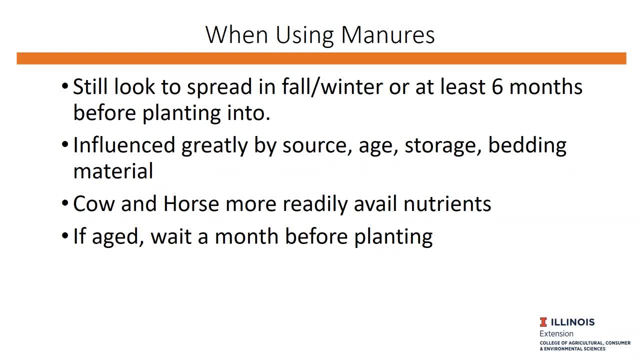 really tend to see that it's going to burn if it's an aged manure. we don't really tend to see that it's going to burn if it's an aged manure. we don't really tend to see that it's going to burn in the plants, compared to, say, kind of those raw manures, where it does yet again the raw manure. 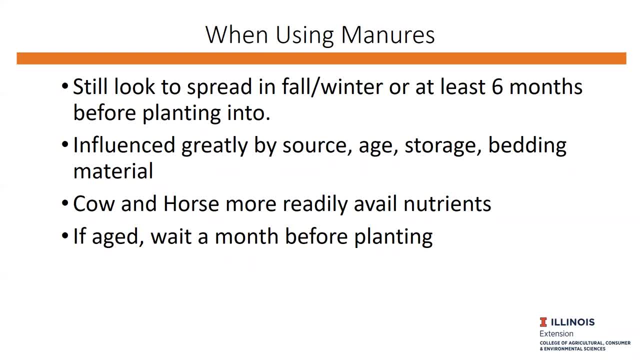 application is different, the time period is, but i still tend to think about a good month of eight of the aged manure at the soil can really help kind of get your soil biological communities woken up. not mentioned on this slide is that if you're a certified organic grower you do have 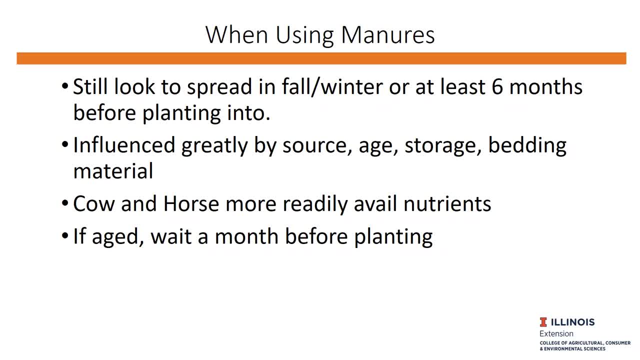 the 90 to 120 day rule, where you can apply raw manure if it is a, if you're going to be growing crops, in which case you um the edible portion does not come to contact with the soil. so that would be 90 days of raw manure for something like a tomato versus 120 days you. 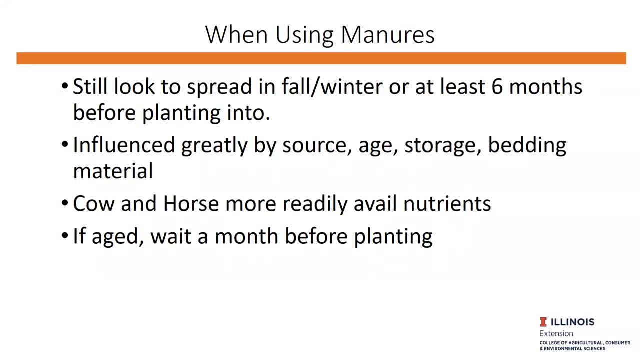 might see something like a cabbage, for instance, with it. those rules may change, so kind of keep that in mind. but yet again, we still tend to take more of the fall winter application. this chart gives you a little bit of an overview of the npk values of a wide 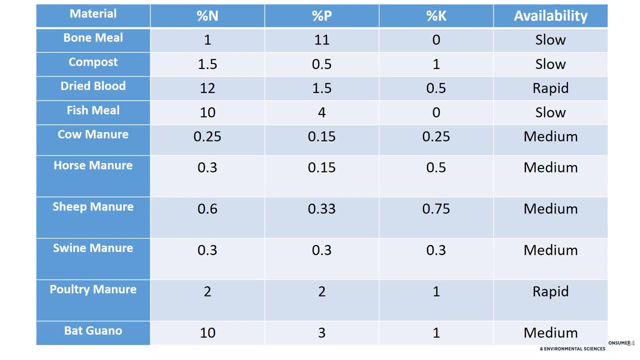 range of organic matter. it also it gives you a the far, uh the far column shows you the availability of these nutrients. just to give you some context as to will these be available in a seasonal basis. versus uh may take a couple of years. these are all averages, so you actually may find that the npk 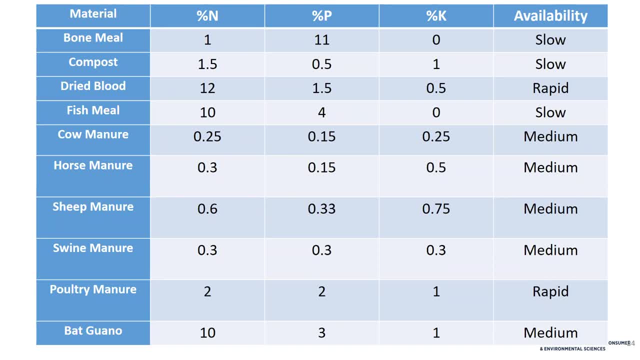 value for a certain organic matter you might be using is is much different than this. you will note that if it says slow, that tends to be a little bit slower, and if it says slow, that tends to be a little bit slower to be, that we expect about a third of that. 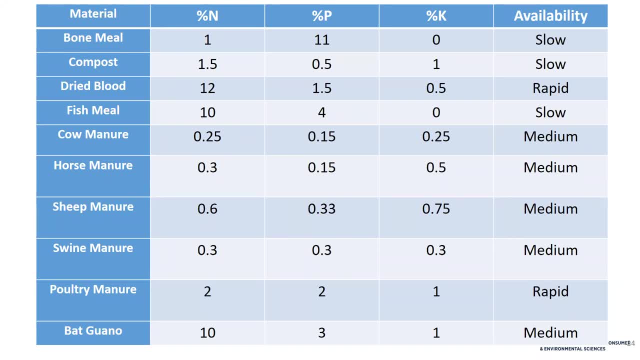 npk value to be released, uh, every year for the next three years. that's especially true for compost and some of our other products too. a more rapid release. you will find that tends to be released pretty, pretty quickly in that seasonal basis, and the same with some of our medium ones as well. 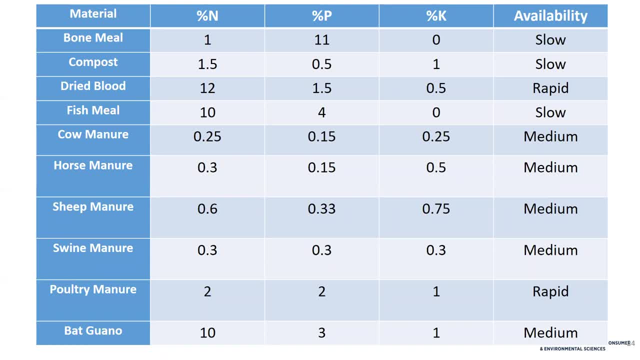 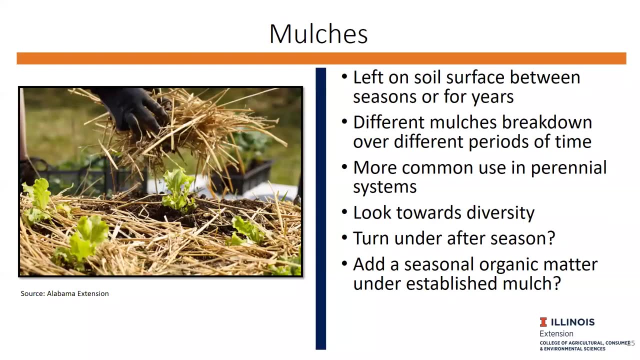 with it. yet again. i'm combining a lot of this information with soil past to ensure that i'm applying kind of the wet soilכשau and the added material, to make sure that when you're settings regarding un methods as well, this right amount and what needs to also be applied Mulch is then left on sole. 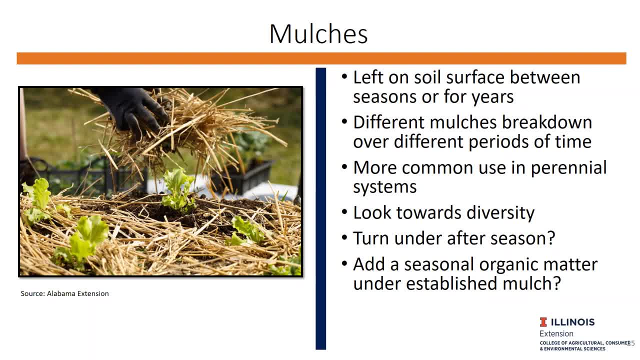 surface between seasons, or this could also be something for years to come, especially in a perennial system. Different mulches also break down over different periods of time, so you will find that situation More common use. like I share with you in perennial systems, I would still maybe look a little bit. 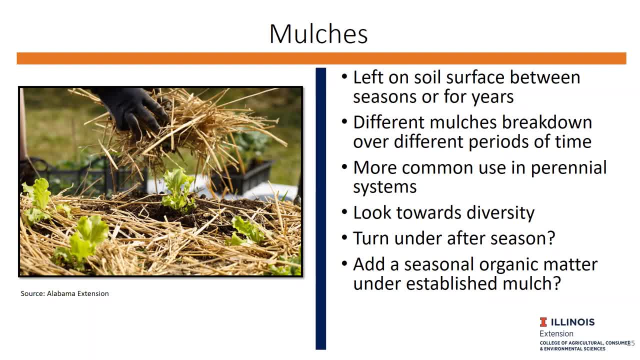 towards diversity in your mulching systems, especially as they will break down a little bit differently- and we hope they will break down really well to organic matter, Because it is on that soil surface. we do expect to lose some of it to the atmosphere and to environmental conditions, so it may not. 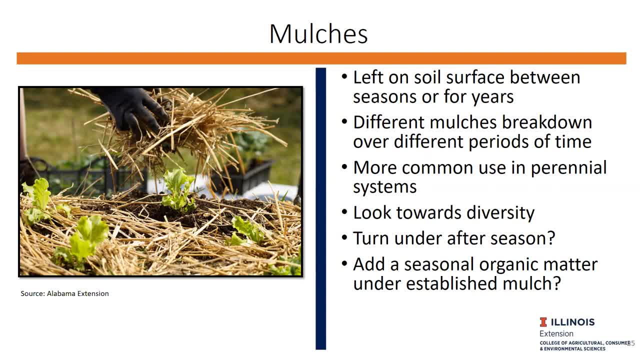 truly get to the end goal of that soil organic matter, because we are losing some to the atmosphere and so forth For some of our annual plants. I would also encourage you to think about maybe turning it under after the season, because that could then kind of break down a little bit further. If I had 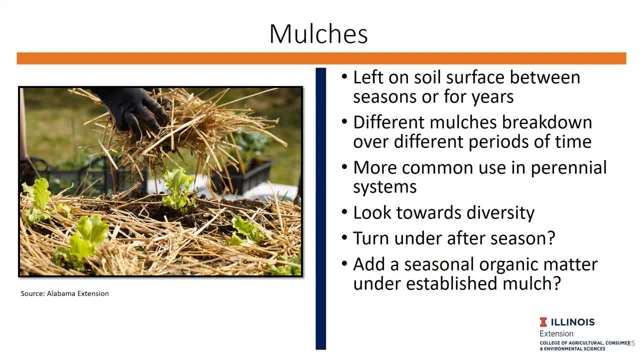 perennial systems- and I had a perennial system I would probably want to look at- had organic or mulches in place on the soil surface. I might still put some compost or some maybe aged manure around the base of these perennial plants just to have additional organic matter in there. 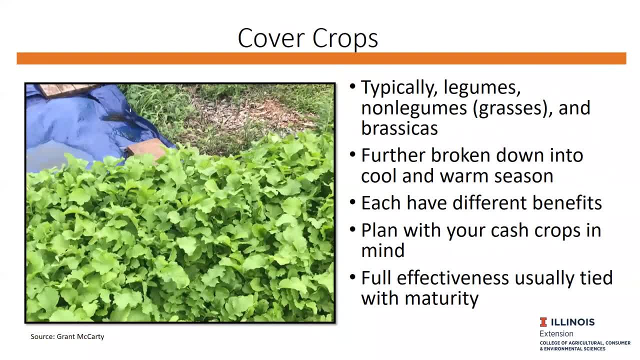 under that established mulch. So my grown organic matter, this is cover crops, So typically legumes, non-legumes and brassicas. Non-legumes tends to be my grasses, my grass family. These are cool season, warm season cover cropping systems. 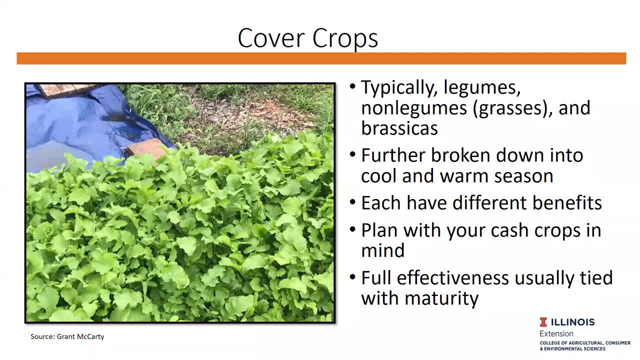 Each has lots of different benefits. They each have very different organic matters with them. Always think about planning your cash crops in mind And then note that full effectiveness, like I shared with you, tends to be tied to when it actually starts to flower. 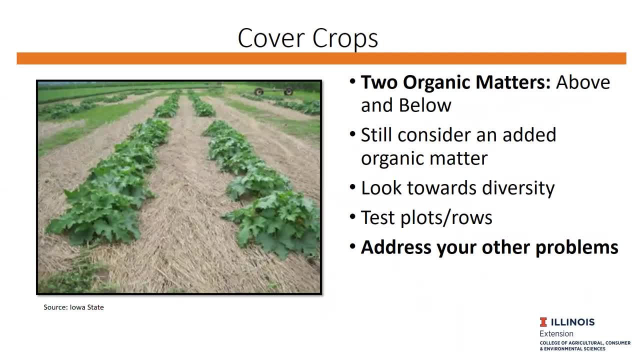 The benefit with cover crops is that you actually are growing too organic matter. We don't always recognize that, But the above and the below ground organic matters are really important. when it comes to adding to your soil organic matter, I would still maybe play around with adding. 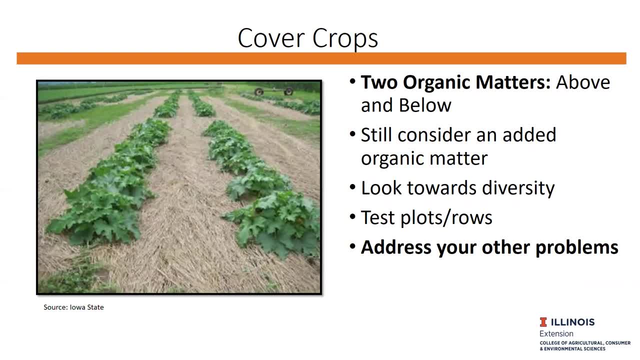 another organic matter, especially an added one. if you could Look towards diversity, especially with the cover cropping systems, You will find so many different ones out there: Test pots, rows. this is all crucial to having a good experience with cover crops. 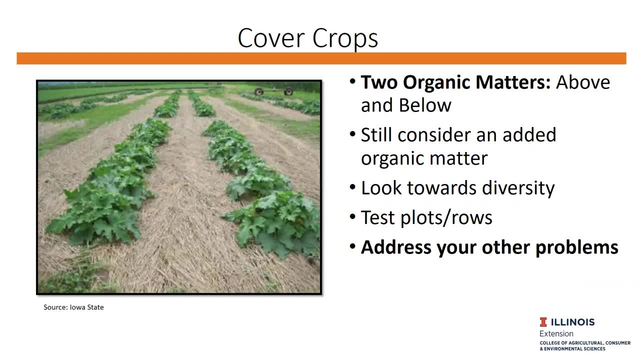 and utilizing them effectively in your organic matter systems and addressing soil organic matter Also. combine this with those that could address your other problems. A cover crop, of course, is going to have great organic matter, but there are some that could help with compaction. 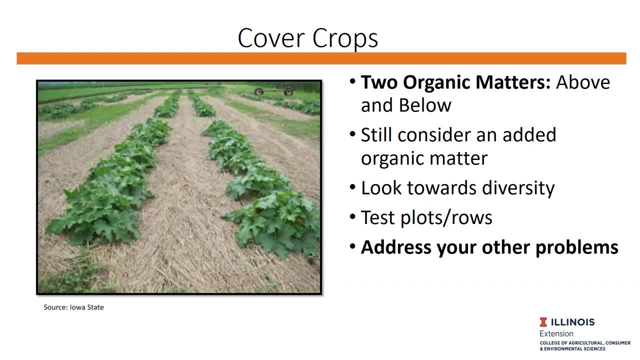 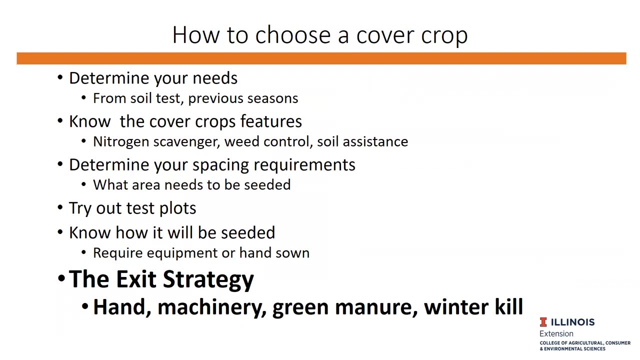 There are some that could help with nutrient foraging. There are some that could help with weed control, But there's lots of other benefits to them, along with this great organic matter that will be added to the soil. This is a kind of an overview of how to choose a cover crop. 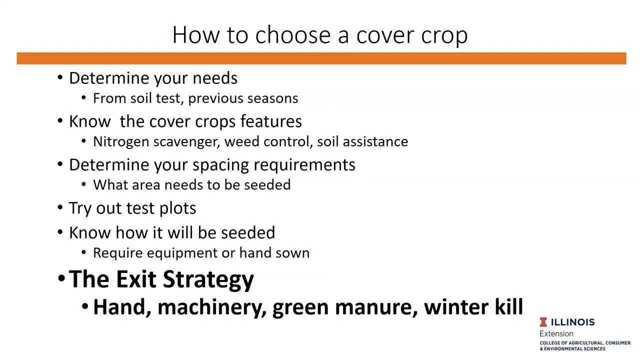 The one thing to kind of highlight and kind of talk a little more is this excess soil. The excess soil is one of the factors that can really make a difference in your organic matter strategy, And this is taken from Dr Ajay Nair at Iowa State. 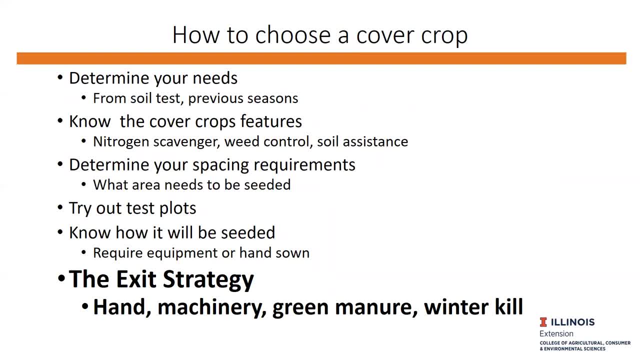 in some of his cover crop commandments or his cover crop presentations. But I really encourage you to kind of know how you're going to get rid of that cover crop and address the cover crop, Because we want you to utilize it but we also want you to grow that cash crop with vegetables. 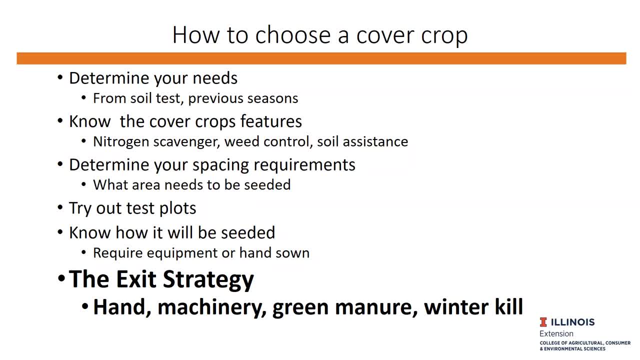 fruits and other things. So you need to know how you need to get rid of it or kill it or actually have it be prepared and ready for your next season. So know an exit strategy as you're thinking about the cover crops and how you're. 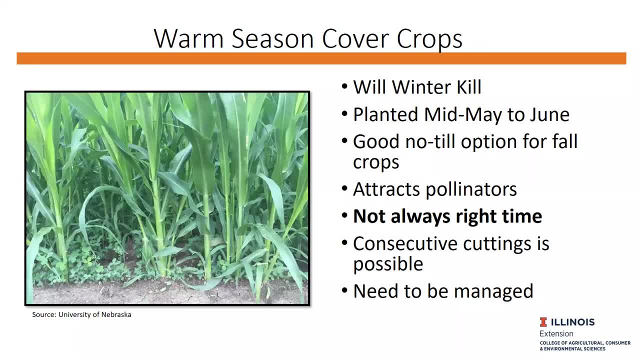 going to get out of it. Warm season cover crops. just briefly. they winter kill. They tend to be planted in mid-May to June. We see this very common in northern Illinois that we have to kind of plant around that time You might be able to get away with it a little bit earlier. 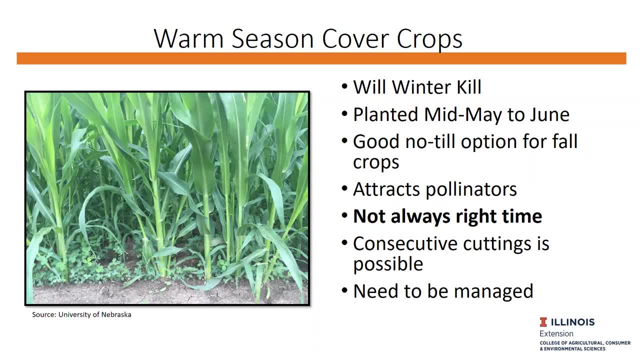 depending on your growing area. Some of them will flower. They tend to attract pollinators, but all of them tend to do that They do. The biomass can be pretty substantial for some of them, Something like sorghum sudangrass, which you see here. 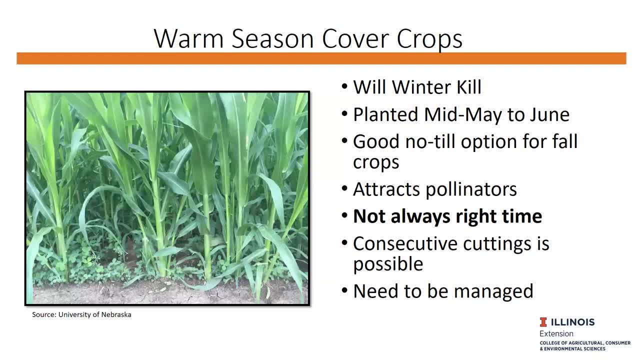 a lot of biomass in the summer And yet that might be what you really need for your soil organic matter system. They tend to need to be managed, especially the summer ones, And you also have to think about maybe consecutive cuttings Potentially might be possible in this situation. 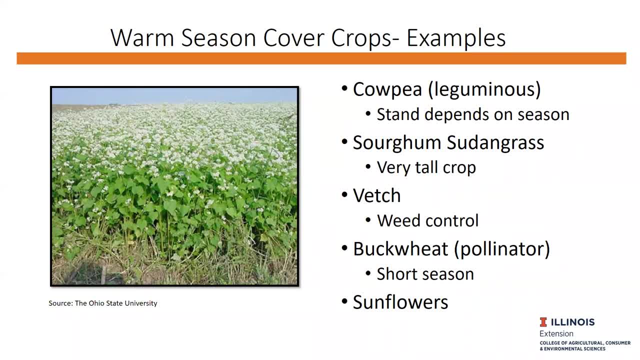 Some warm season cover crops. examples: cowpea, sorghum, sudangrass, buckwheat. cowpea is leguminous, which is what we like, So it gets a question of nitrogen soil. Buckwheat, as you see here in this photo. 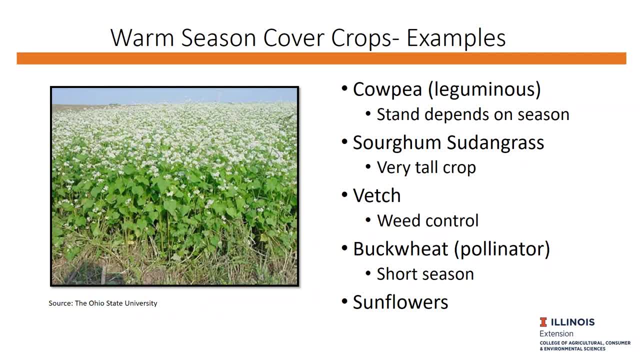 tends to be a good pollinator, but also very short season- 45, 50 days before it starts to flower and goes to seed And you've got to address it. You have to address buckwheat as it starts to flower. 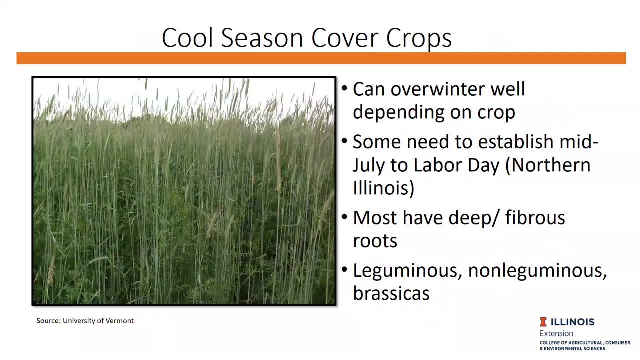 And usually this will mean cutting it and laying on the soil surface The cool season cover crops. these are usually over winter. well, depending on the crop, Most of them have very deep fibrous roots with them. This is leguminous, non-leguminous. 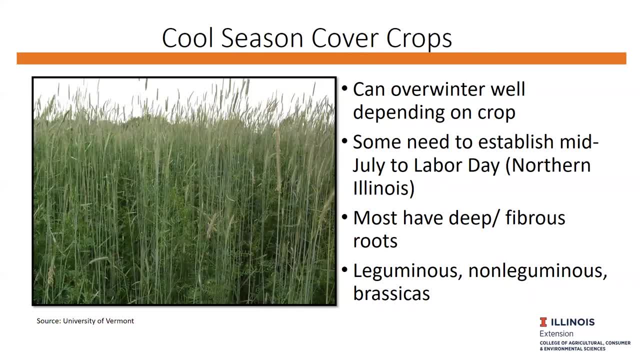 as well as brassicas. In northern Illinois we tend to see establish that sometimes mid-July is the labor day. We can go a little bit into October, but sometimes we don't see as much of a great establishment as we would like for these cool season cover crops. 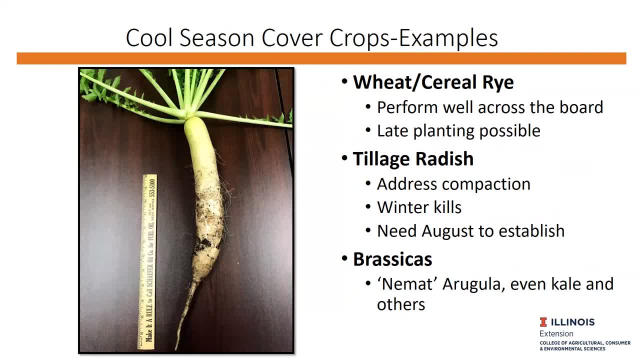 Wheat, cereal rye, the most common ones for the cool season cover crops. They just perform well across the board. Late planting can be possible with them. As far as just good organic matter, good root systems, you really see that they do a lot of good here. 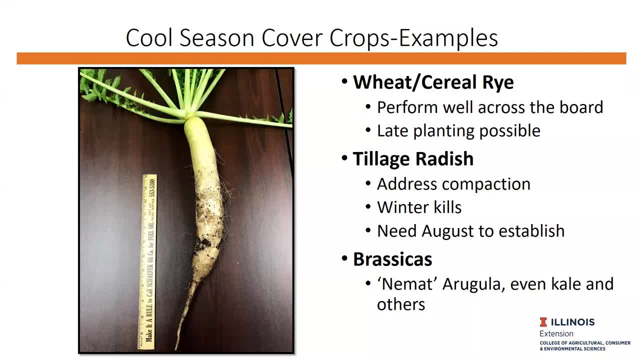 Tillage radish as you see in this photo. you sometimes see it as daikon radish as well. We have it growing in some of our raised beds here at the Extension Office. This was harvested about two months into planting, So we planted about the first week of August. 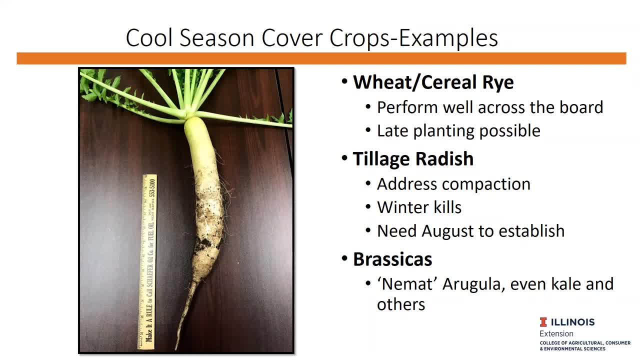 and then we followed up at the end of September and I harvested this And you can actually see we had lots of good root growth in the matter of two months. So it can grow well, but it has to be established in August or else you will not get this type of organic matter. 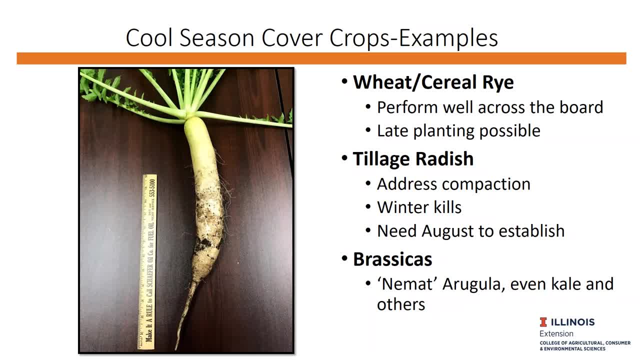 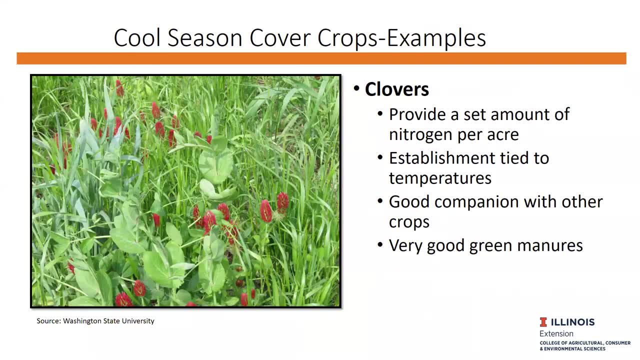 And in winter, kills. it's breaking down right now under the soil cover or the snow cover rather up here in northern Illinois. Clover is another category, of course too. Lots of good organic matter, a good amount of nitrogenized soil surface as well, rather into the soil system. 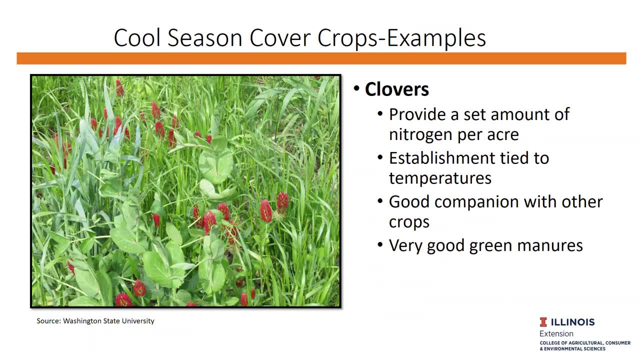 It can be a good companion plant with other crops. It can also be a very good green manure in that system too, But one that I can balance out my soil fertility here. One way that some folks will kill certain cover crops is with green manure. 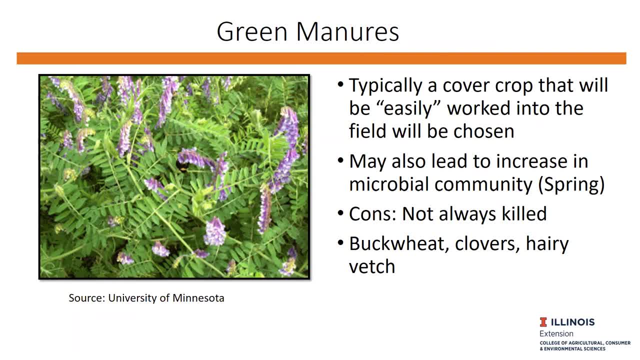 So this is an ax where I'm actually kind of turning them underneath the soil surface into the soil, usually with some form of a tiller or some kind of other apparatus. So it will kill it. It will tend to kind of increase his microbial community. 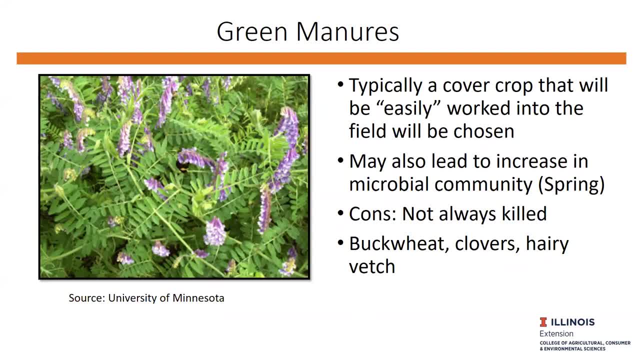 especially in the springtime when it's done. So you're kind of giving them good fresh residues to actually actually start breaking down. The issue, though, is that it's not always killed. It can be a little troublesome Hairy vex, which you see in this photo. 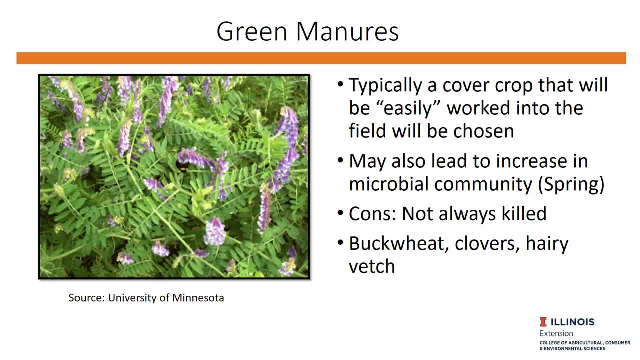 is also one where, yes, it is a green manure, But, my goodness, if you've tried to actually till this under the vining characteristics- can be pretty hard to work with and pretty hard to deal with. Living mulch is also where a lot of organic matter discussion. 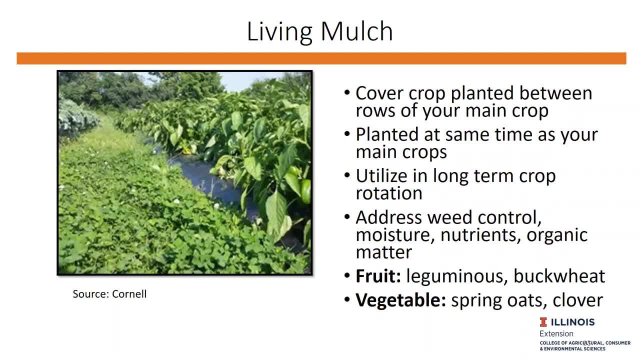 is going growing your own kind of living mulching system with cover crops, where you could then be giving a break to some of your rows of plants that you're growing on a seasonal basis. So this long-term crop rotation is really where we start to see a lot of interest in it. 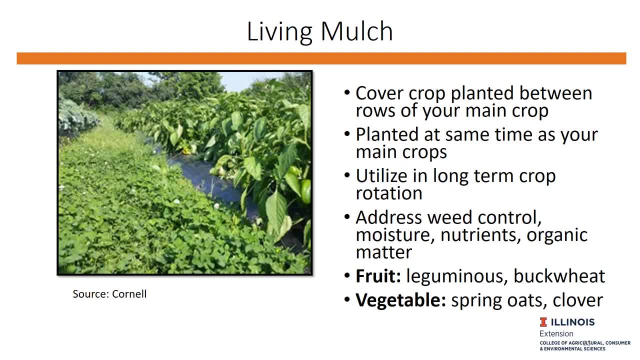 It could address. weed control could help with moisture nutrients, but also some really good organic matter For fruit production. this looks to be leguminous buckwheat or vegetables. sometimes spring oats, as well as clovers, fit within the system. 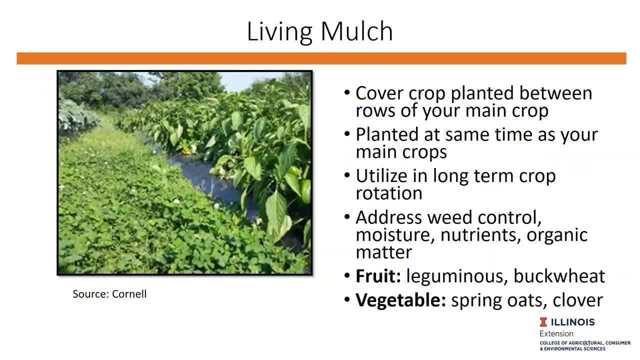 pretty well too. But it is basically a cover crop planted between the rows of your main crop, And this could allow for you to kind of add more organic matter between seasons for certain growing areas on your operation and not grow anything in there. And, yes, it is acting as weed control. 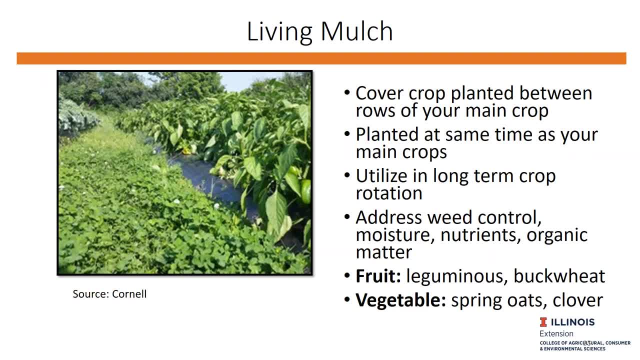 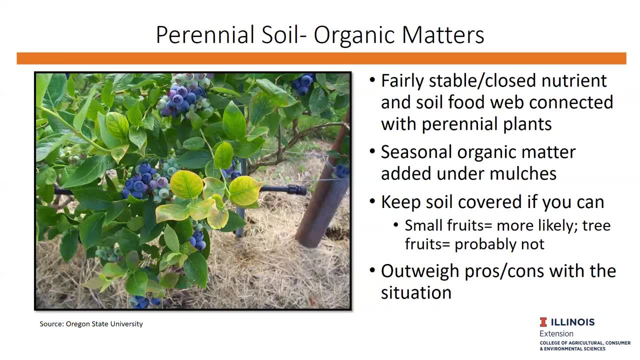 but it also could be adding additional good organic matter for those rows. that kind of need maybe a little bit of a break between seasons. A lot of what we've talked about today is a little bit more annual plant-focused. I want to just kind of mention here: 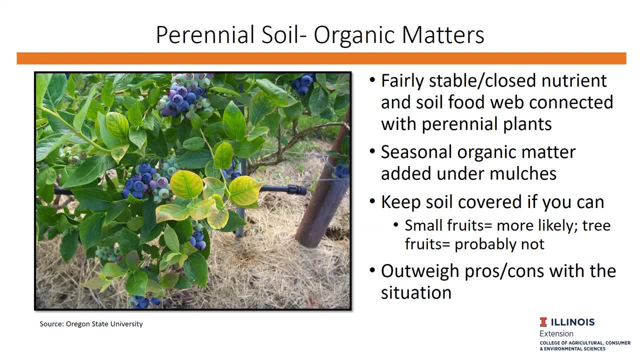 that perennial soil organic matters fairly stable. We see soil biological communities really stable. when it comes to these perennial plants, They have a very closed nutrient system in most cases And they also tend to be kind of a soil food web. that's connected. 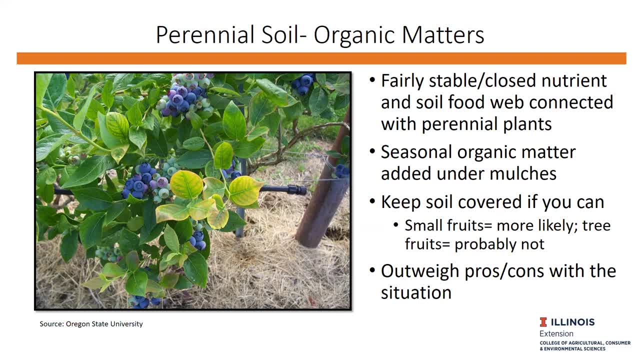 quite well with these roots and the rhizospheres Still look towards seed, Seasonal organic matter added under the mulches. if you can Still kind of see if it's possible for you to kind of pull back some of the mulches that you might have in place, put some compost down. 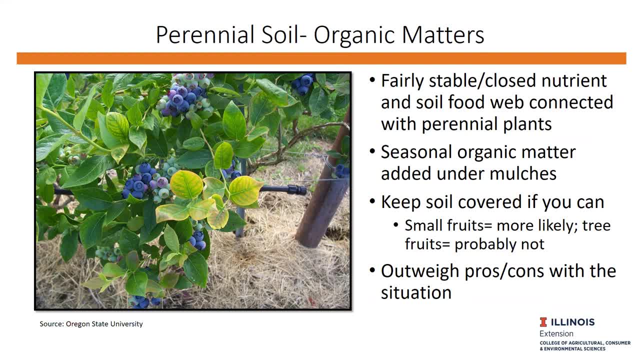 put some aged manure down, have it in some capacity with them. This is probably more likely for small fruits, for berries, for brambles, Tree fruits. it may not be, And that tends to be just because we're trying to be a little concerned about managing. 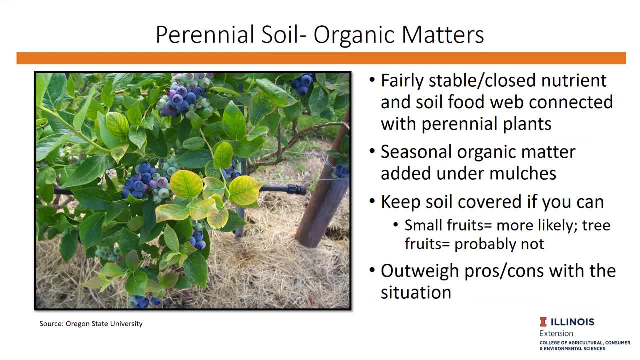 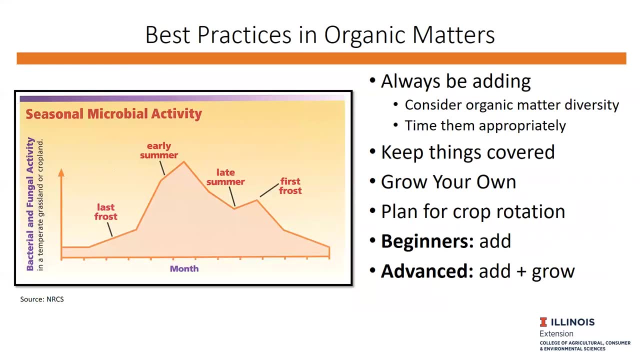 some of our wildlife and wildlife, especially moles and other smaller animals, will find a place to harbor and hang out around a mulch system, around your fruit trees, So we may not see that too much. So really look at the pros and the cons here with the situation. 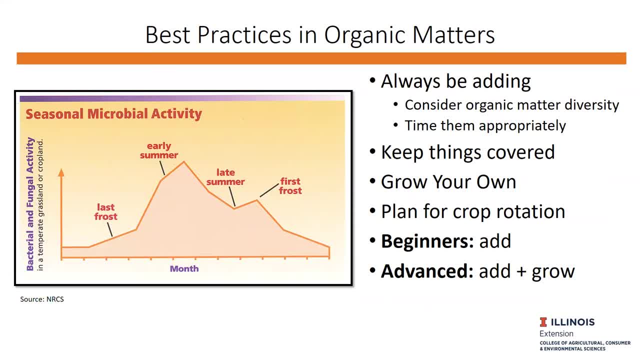 So best practices in organic matters, then I tend to be on the camp of always be adding, And while you may be at a place where you've added so much that you're like you know, maybe I'll take a break there, And I do recognize that. 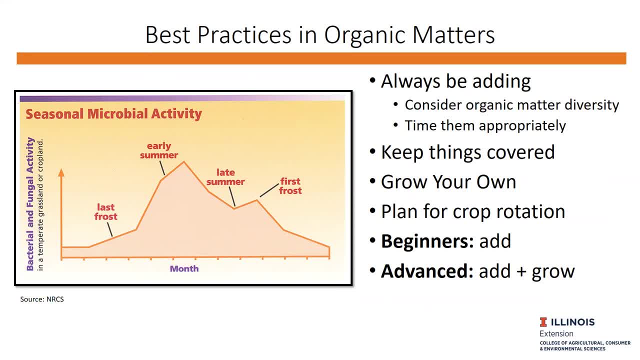 But I think, especially if you're growing in a new area that you've not grown before, you're growing lots of annual plants- this is really a good time to really start thinking about adding and really focusing a lot of organic matter diversity. I also think about timing things appropriately. 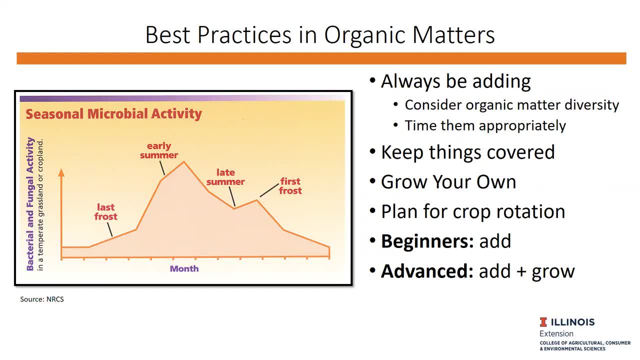 You see this chart from NRCS And we actually see that there is an increase in bacterial and fungal activity. that happens around early summer. So thinking about, say, end of May, into June we start to see activity. This is a time where these 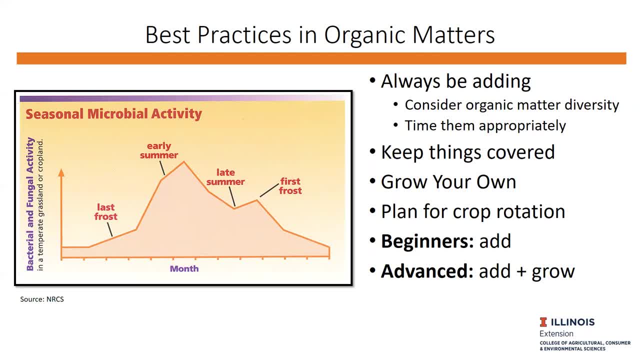 OK. Communities could really use some food and really think about where your compost application is. This might mean the end of April. This might mean mid-April, where you might apply the good organic matter. Try to keep things covered. Have some kind of surface mulch layer in place. 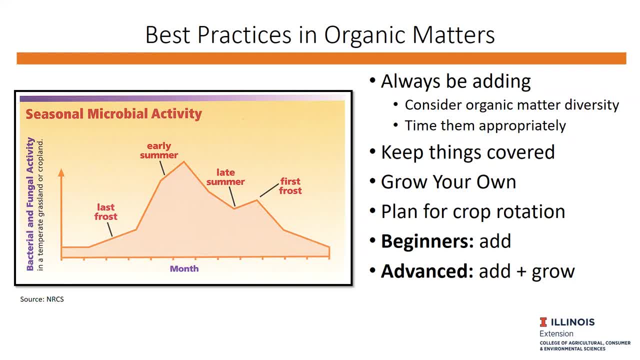 Grow your own cover crops, Grow your own organic matter. Still plan for crop rotation. That's something to not let go of because it can help with that. From a beginner point of view, you're probably in the adding stage. as you become more advanced, you want to do adding. 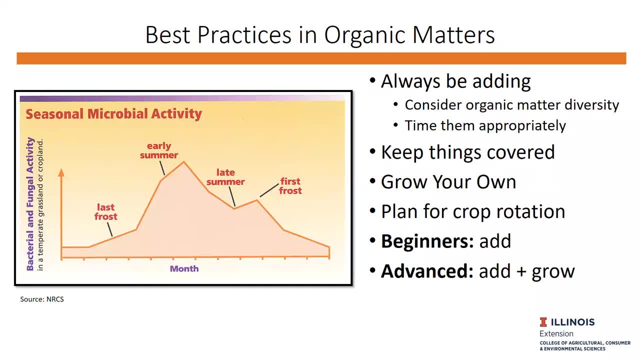 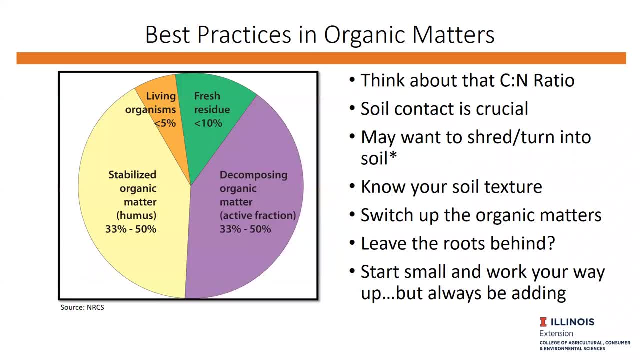 And you also want to consider growing your own cover crops, because you're going to find some really great benefits for your soil organic matter by actually growing your own organic matter More here, consider a bit about that C to N ratio. I think it's especially crucial when 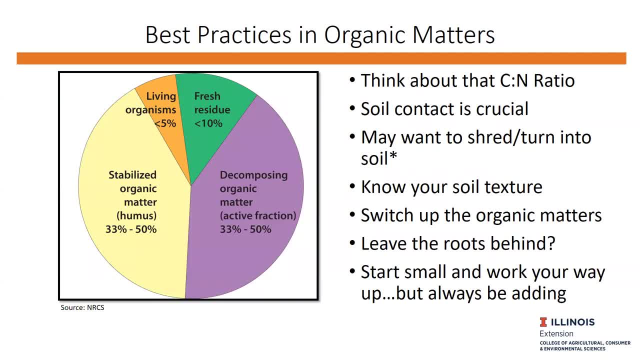 it comes to maybe some of the mulches that you might be using for organic matter, that you might be using as well Soil can. contact is crucial here too. If you're using any kind of plastic mulch system, know that you've got to get the organic matter. 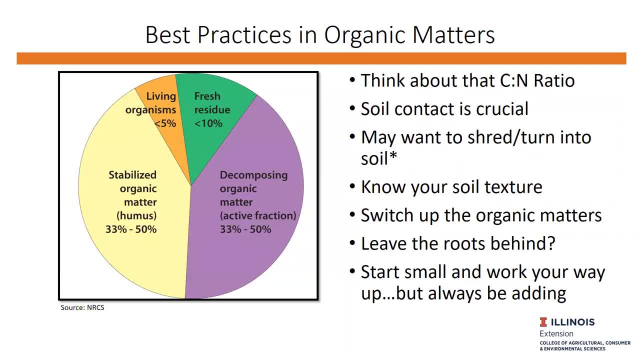 in touching that soil in some capacity, So that maybe it's around the base of the plants that season, or it actually is at the start of the season, where you're adding the organic matter and then you're covering up with the plastic mulch. 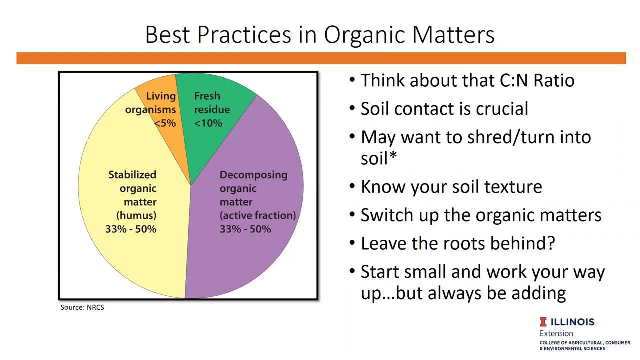 But you've got to have contact there. They may want to shred some of these organic matter and turn to the soil just to kind of help decomposition. Consider too your soil texture. You may find that that may be limited to sometimes what organic matters make the most sense to you. 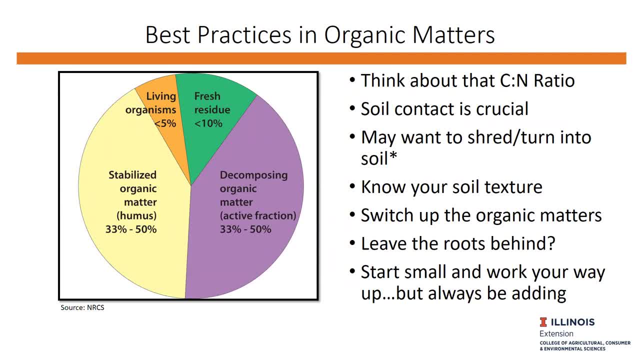 So which of the organic matters? And then maybe it's time to think about leaving those roots behind, And yet again, we're still thinking a little bit more about this. for some of our annual systems, We might be at a place of thinking that these good root systems could really 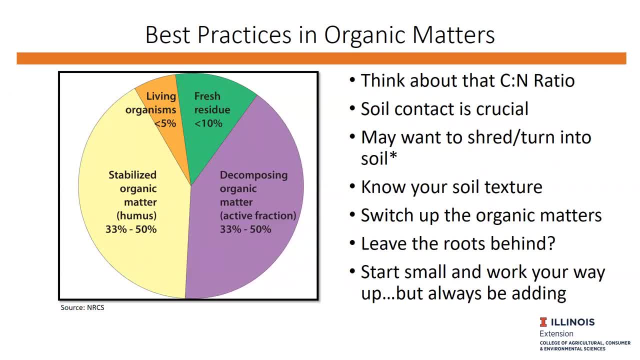 be providing a lot of good for us within this capacity. Yet again, I'm still wrapping my head around what this could look like, other than just removing the upper portion of those crops that you might be growing. Start small, Work your way up. 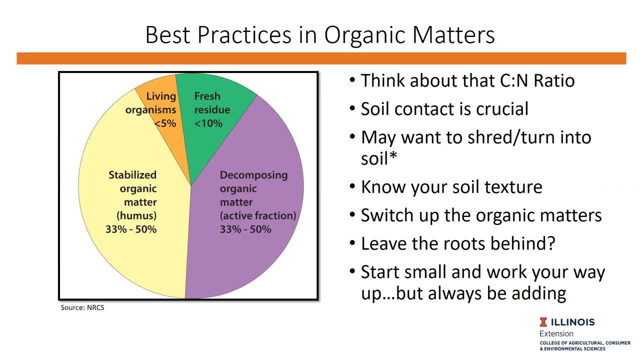 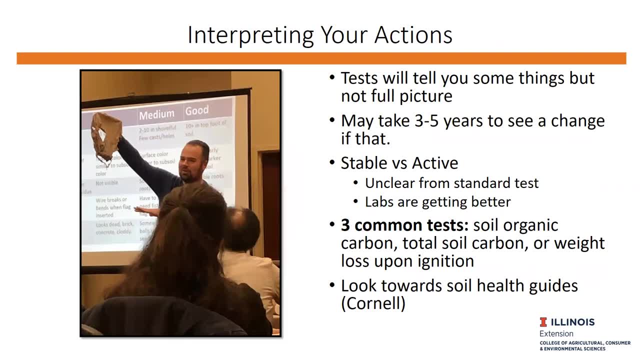 Get a soil test, Figure out what's going on, But really think about adding to that system. So interpreting your actions. If you were in my classroom today and we were talking about this, you would get to see the underwear test which you see here in this photo. 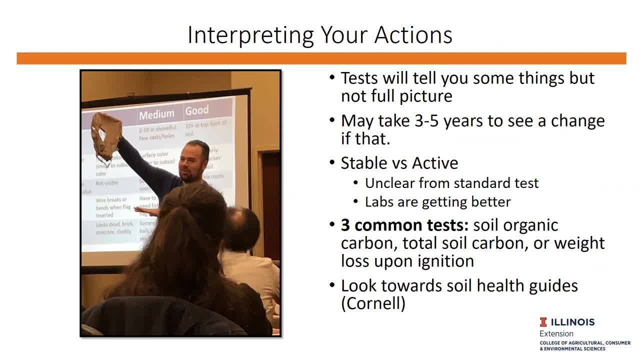 The underwear test is done to kind of measure soil biology. So you're planting a pair of men's white cotton briefs, usually during the mid-summer. You're planting them for about two months or in about a depth of two to three inches. 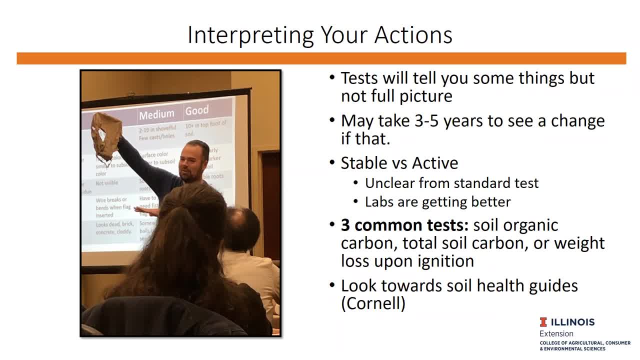 You unbury them, these men's briefs, And because it is a food source, you actually see a lot of decomposition on this to then show that you've got some really good soil biological activity occurring. It's purely anecdotal, but it sometimes 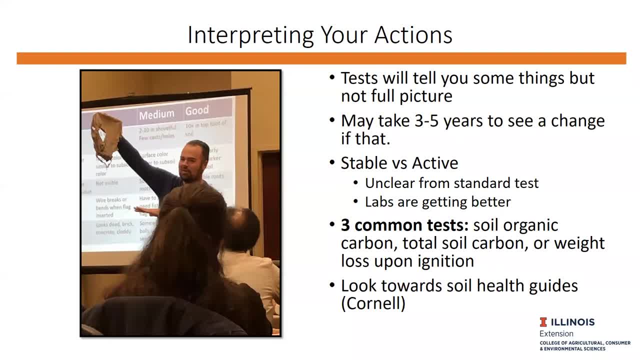 is an interesting visual estimate for some people about soil health and what the organic matter kind of looks like. The other thing to share here is that tests will tell you some things but they don't always tell you the full picture. That percentage of soil organic matter. 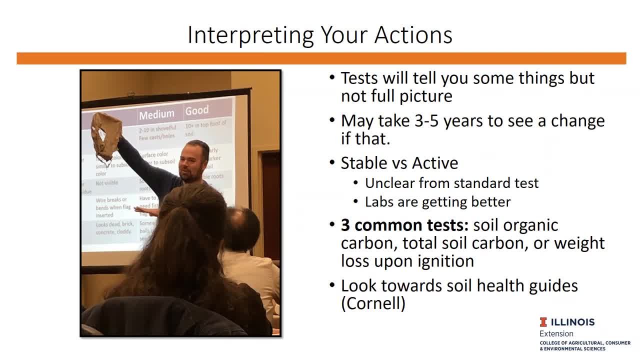 doesn't tell me if it's mostly fresh ingredients that have been added in the last five years versus that stable organic matter that is mostly of the humus itself. So we don't have a full picture. sometimes from the soil test. It may take three to five years to also see this change. 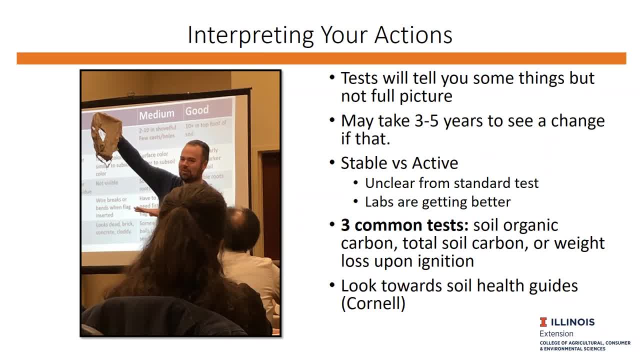 So most of the time the soil organic matter information you're getting back isn't necessarily breaking that down to stable versus active. The labs are getting better. There are three common tests when it comes to soil organic matter. The one that we mostly see is the kind of weight. 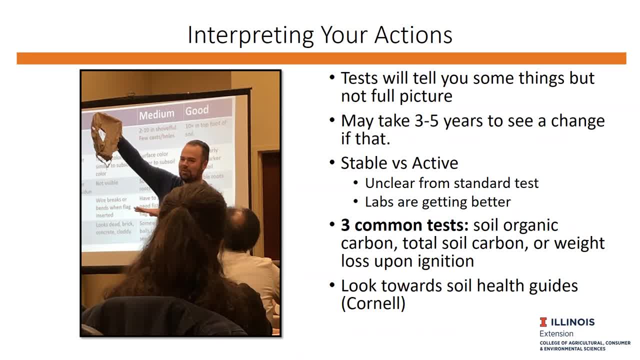 loss on pond emission. That's the most standard soil test that you see in a standard soil from a standard soil testing lab. The top two are a little bit trendier. They may be a little more costly. Also, look towards Cornell with some good soil health guides. 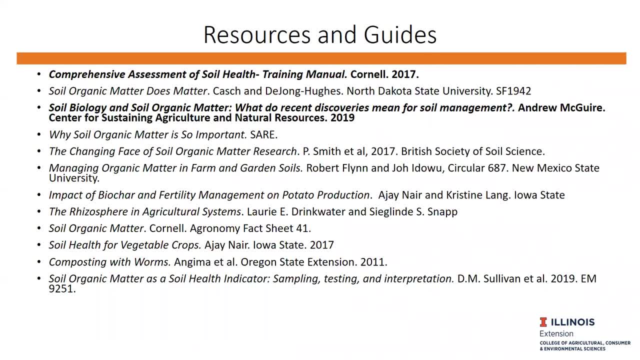 So I'm starting to wrap up a little bit here. So I would say, Zach, we encourage you to start giving some questions in. I want to mention a couple of resources and guides for you. Cornell, as you see on the bowl, the Comprehensive Assessment. 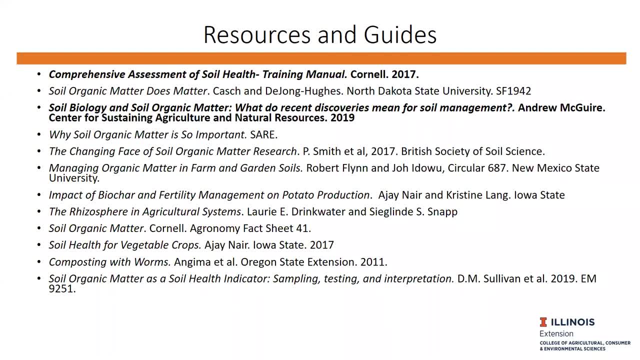 of Soil Health. it's a very good training manual on soil health and soil organic matter. I really like it quite a bit. That would be a great place to start with you. The discoveries, the changes, the research, all of that stuff. 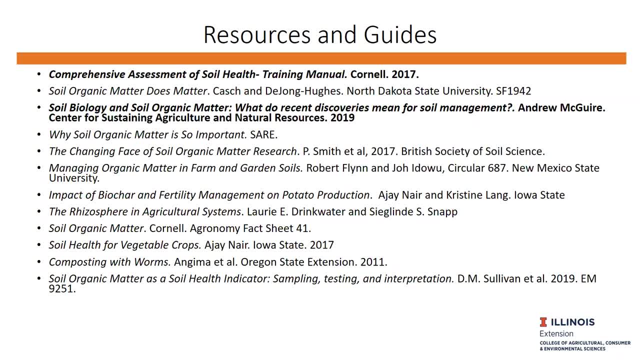 is happening in the last couple of years. It's kind of zeroed in to this document called Soil Biology and Soil Organic Matter. What Do Recent Discoveries Mean for Soil Management? Andrew McGuire has just hit it, hit the nail on the head. 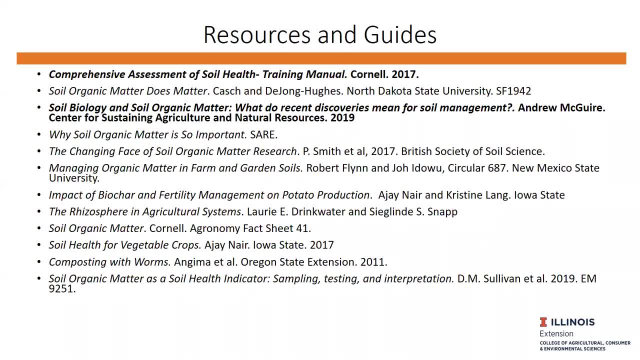 when it comes to kind of summing this up. So I really like that document and encourage you to kind of look at that. Some of the other resources here are more soil, organic matter overview, different extension and publications that can help you with that. 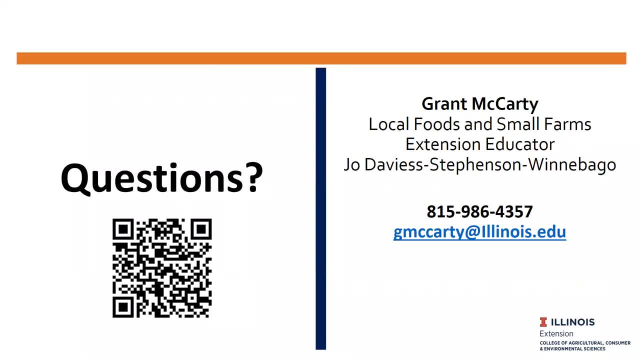 All right, So that's my phone number. That's my email. Sorry about that. We talked about the disturbance earlier with the phone call. But yes, let's get some questions answered if we can. Great Thanks, Grant. Great discussion on the differences and confusion. 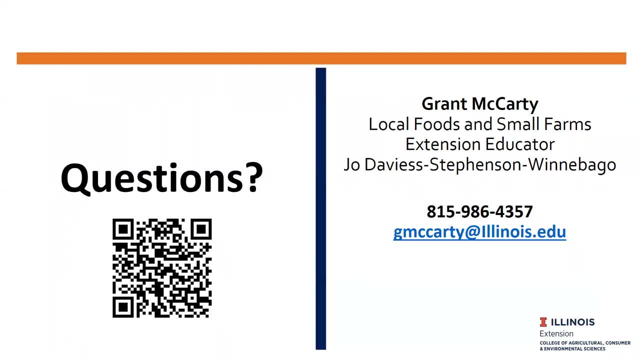 sometimes with the difference between soil, organic matter and organic matter input. So great discussion. We do have a few questions coming in that we can pull in in a second. We've got about five minutes left, so we will likely go over the 1 PM hour for this discussion. 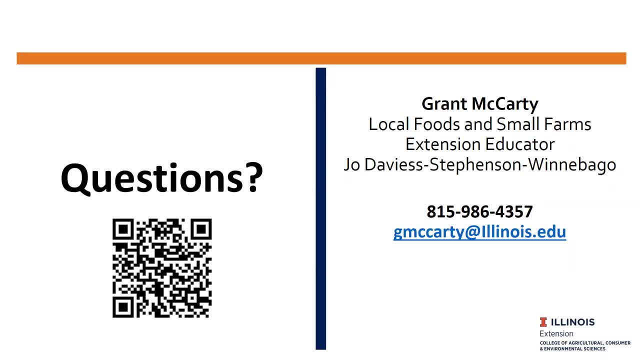 period. for those of you who need to get off the call. I actually want to start off with a comment and maybe open up for some discussion or some feedback from you. Grant related to two things: One, compost applications and also manure. 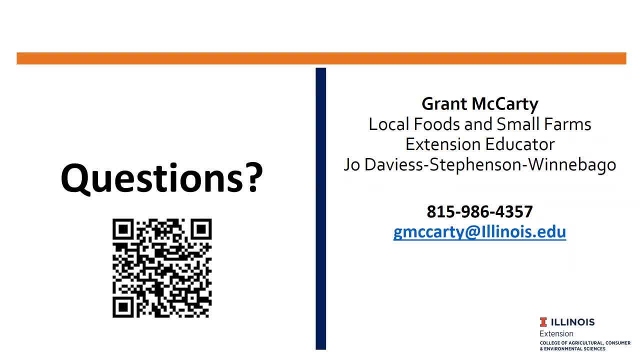 particularly the use of manure in a raw form or what you were describing as an aged form. I want everyone to realize, or just recognize, that the federal government, in the form of the Produce Safety Rule and the Food Safety Modernization Act, they have a very specific definition of what 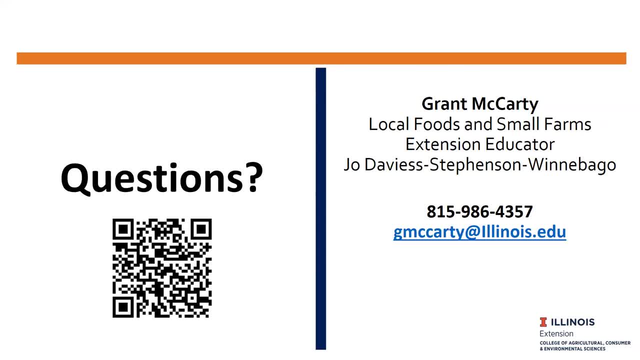 they consider to be what they call biological soil amendments of animal origin, and how they consider them treated versus untreated. So raw manure and aged and stacked manure, at least in the FDA's eyes, would be considered a raw, untreated amendment. So we need to think about those application intervals. 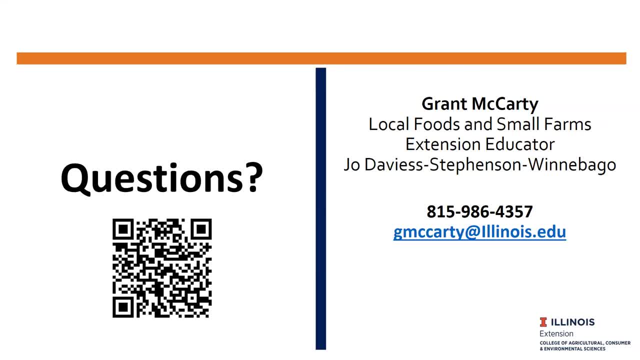 before adding to them to the soil. Grant mentioned the NLP 91 20-day rule which the FDA currently is OK with And saying: go ahead and continue to use that, But they actually have a reserve clause in the Produce Safety Rule. 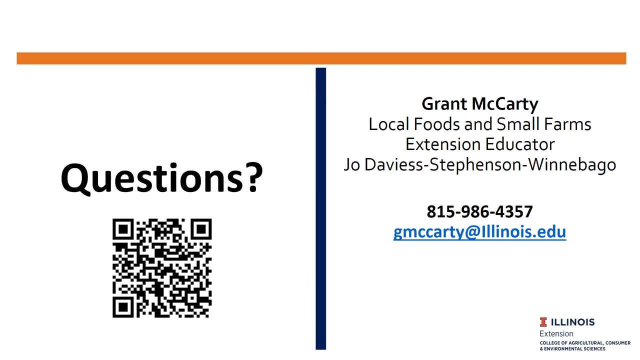 And they still haven't made a final determination about their perspective on adding raw untreated manures, in particular, to the soil. And it's a little counterintuitive too, because most of the fertilizer value from raw manures in particular come early on. 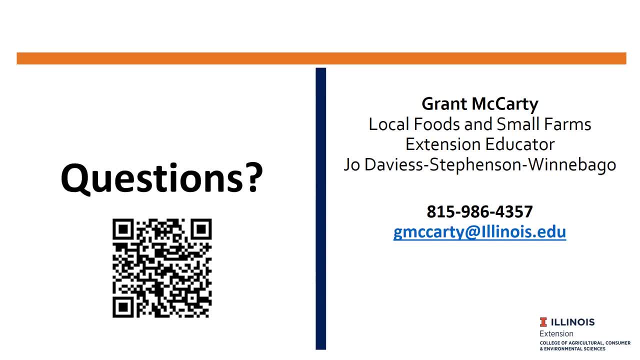 So those manures lose a lot of their fertilizer value within the first five years, The first few days, in fact the first couple of weeks. So it's something to consider with manure in terms of food safety, produce safety issues and whether we're 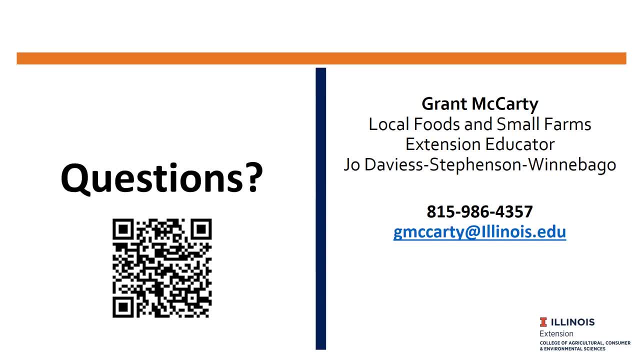 treating them as a fertilizer versus organic material. I would recommend definitely composting manures if at all possible before adding, because then that can increase your chances for adding it to the soil. The other thing I just wanted to briefly mention- and Grant mentioned this multiple times- 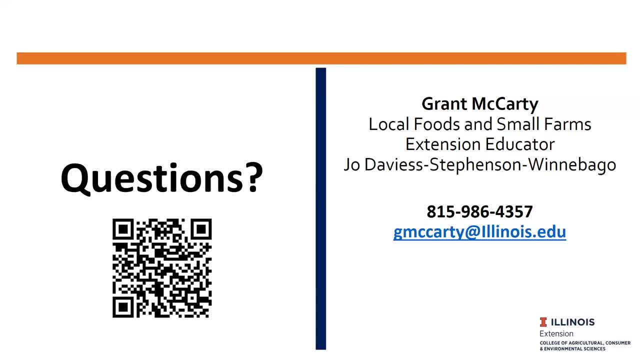 in terms of compost having low NPK values. while that is is true on a pure dry weight analysis basis, we can get into trouble- and there's a lot of interest in this- particularly with small scale farming, no-till systems, where particularly 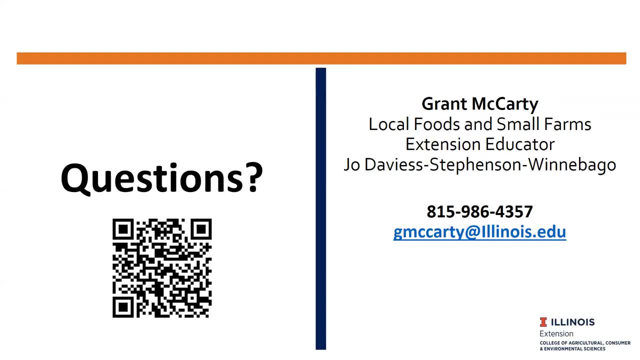 with animal-based compost, we can add lots of phosphorus to the soil, particularly if we're adding large amounts at a time. So there's this impression that more compost is always better. But in the case of phosphorus loading in soils, if we're adding compost to manures that have high levels, 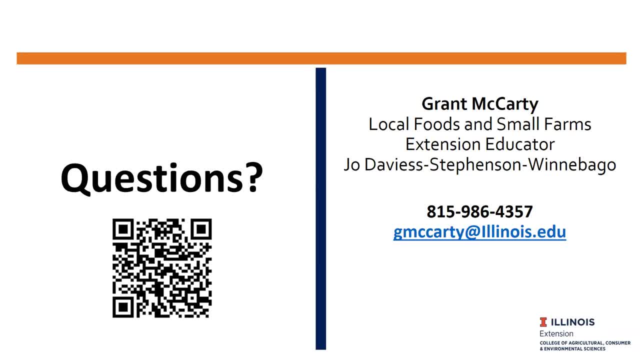 of phosphorus That can have downstream ecosystem effects, and we can load too much phosphorus, even with compost that have low NPK analysis if we're adding lots of them And we're talking on the scale of one to six inches of compost to beds and to fields at a time. 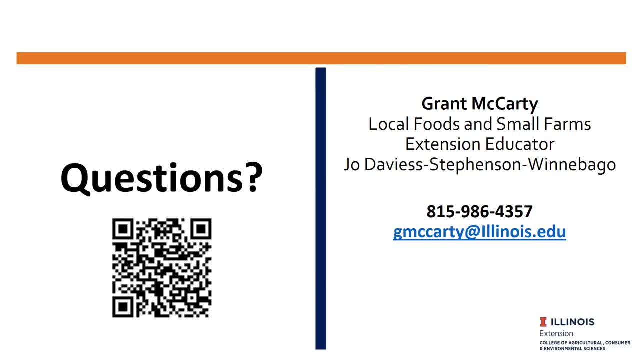 So I just wanted to comment on that. And, Grant, I don't know if you had any follow-up in regards to both the manure and compost question. Yeah, No, I mean you're. I appreciate the assistance there because it is something where, like, yeah, I mean it's like. 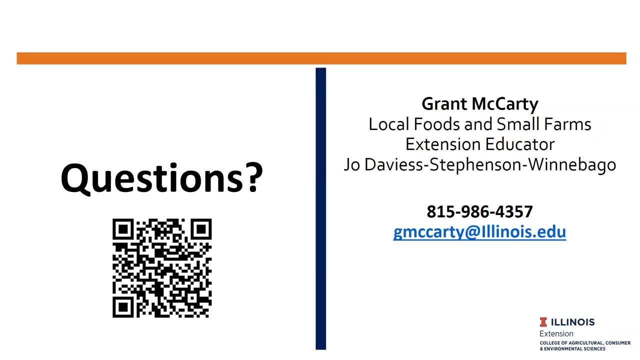 oh, this sounds great. We should have the all the time, And yet we still have to step back and think about what the soil system is that we're operating in, as well as what the growing systems are too, where the end goals are with these. 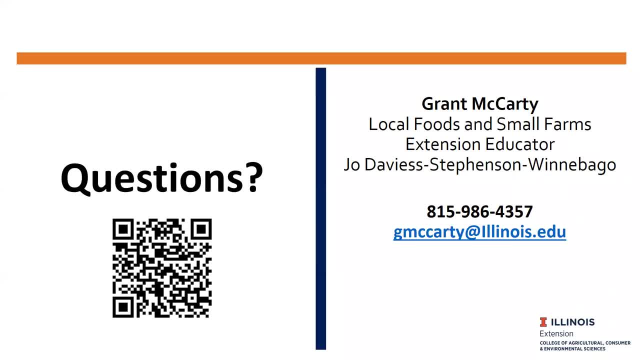 I still look heavily towards raw manure application in the fall. That's still. It tends to be where I tend to kind of have a pulse toward Right And I would totally agree, And if the compost, I mean if the manure is composted- 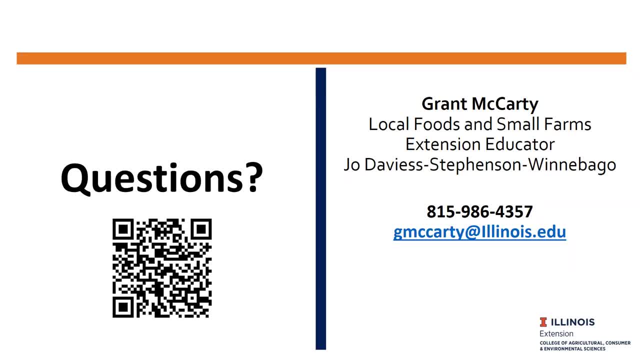 and you can certify that it's compost either through your records or a farmer's records, then the application interval is actually zero if you properly compost. I just wanted to make everyone aware of that. So it's a little confusing, And the FDA's insight on this confuses it even more. 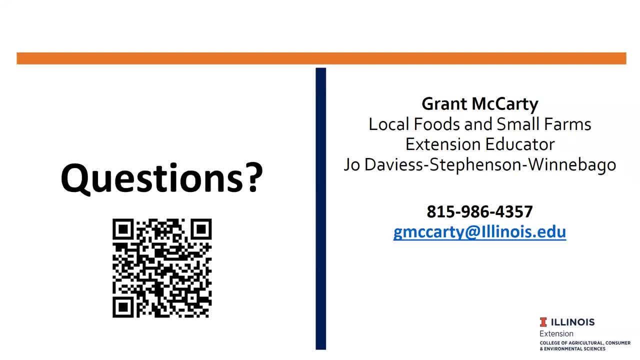 So stay tuned for guidance when it comes to, Yeah, Particularly raw or aged manure applications moving forward. Let's see here. Let's go ahead and jump into the questions here. So someone did. I brought that up because someone did have a question. 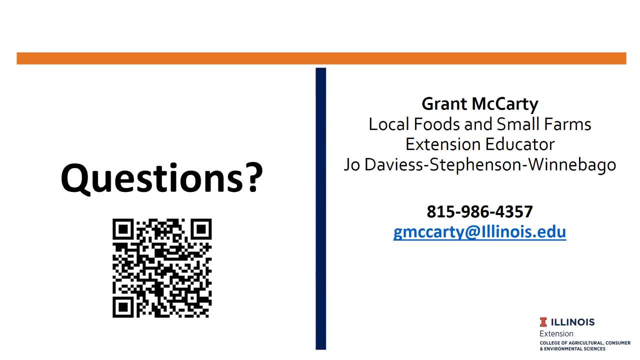 about adding chicken manure and a question about salmonella. So I think that discussion should answer that particular question. So let's go to the top. One question: you mentioned early on something about organic matter inputs that could cause compaction or reduce air and water flow. 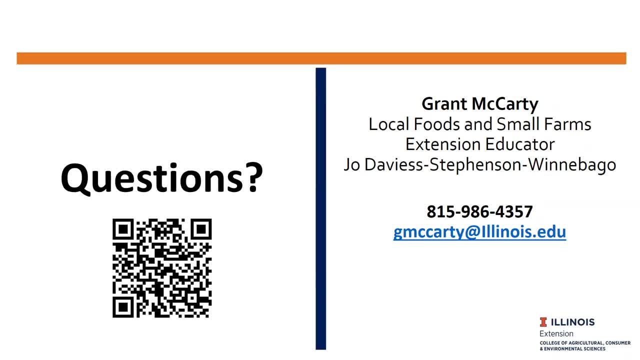 Can you elaborate on that a little bit? Sure, I would see, especially with some of the leaf litter that you might be using, you may find that that mulch layer could be restricting some of the air flow with your soil, Especially if you have some kind of product that maybe you 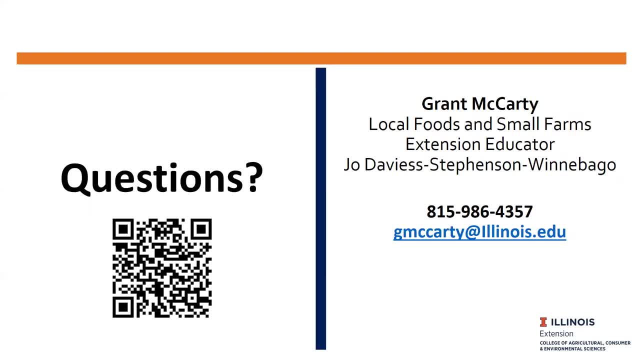 haven't shredded properly or you haven't necessarily got loft up. if you will, You may find that, especially during changes in the weather, you could Create so much pressure that goes right up onto the soil that you may have more of a compaction problem. 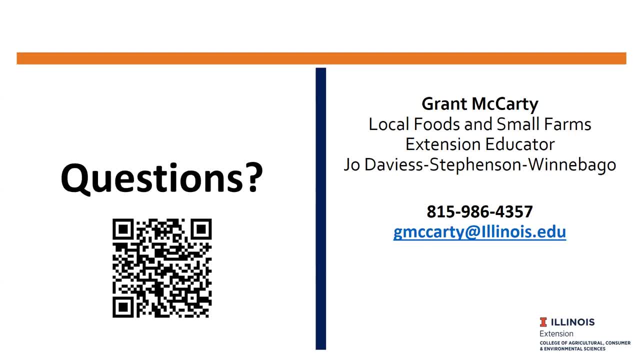 It tends to be more mulches than anything. OK, great. And then another question. I sort of answered it privately, but we can just kind of bring this up in terms of recommendations and amounts of organic matter inputs. I know you kind of hit on that a little bit. 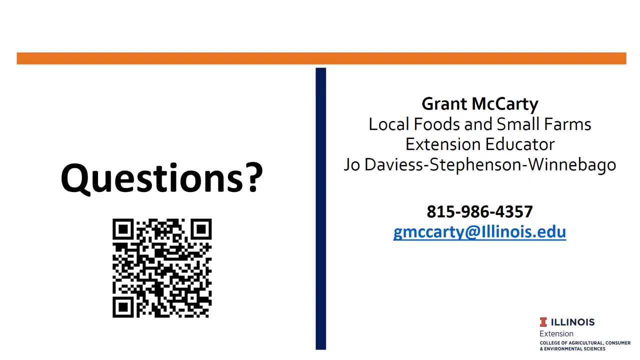 But they were referencing, laying down sheets of newsprint, adding six inches of grass cuttings, incorporating that in. And the question in the fall? and the question is: should I be adding something else? Is that good quality of organic materials? that's acceptable. 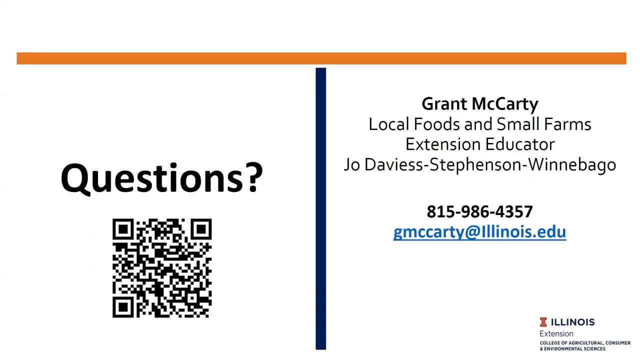 I mentioned that it was a good start but that maybe monitoring your soil organic matter levels and diversifying your organic matter inputs is important, But I think you hit on this already that we don't really have solid recommendations the way that we might with fertilizer or soil correction. 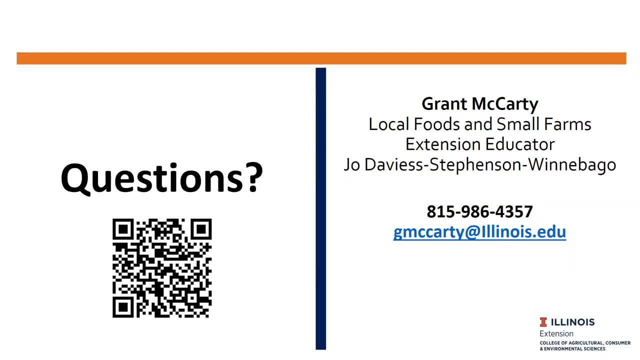 in terms of the amount of organic matter to add and what kind. Yeah, we really don't, And I think it's kind of a case-by-case basis. I think what I do tend to see and tend to encourage is just changing it up when you can. 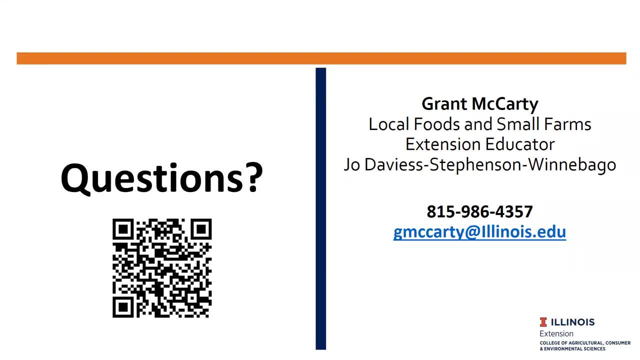 looking for different changes, because you need to have just diverse organic matters for the biological communities. OK, then a question about. I think you mentioned grazing stimulating nematode population. So the question is actually: how does grazing stimulate nematode? 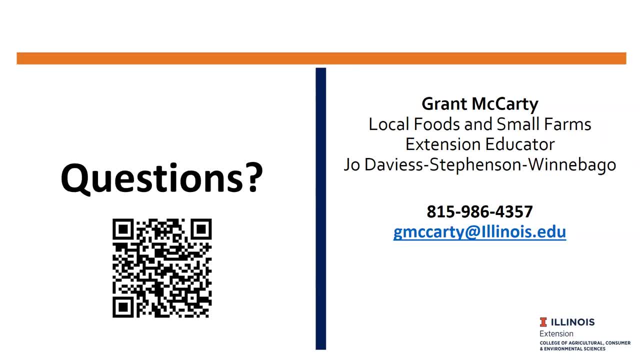 Yeah, So that grazing In turn it's meaning that the populations of prey, bacteria, fungus and so forth- that the nematodes eat on, they're grazing on it, So they're eating that. That's what that should mean. 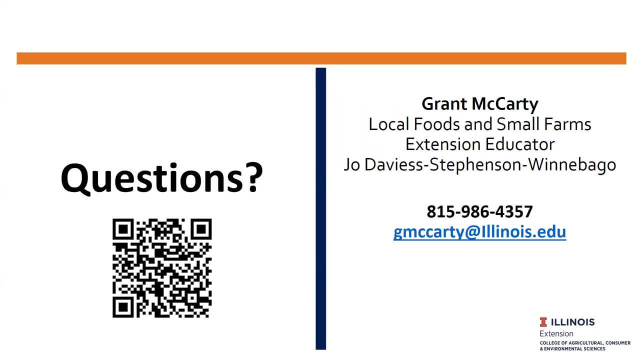 So when you see increases of, say, bacterial fungal communities and the nematodes are present, you will see them graze more actively. I mean, let me clarify, You're not going to see this, but just kind of know that that's what we're getting at here, is that they're grazing. 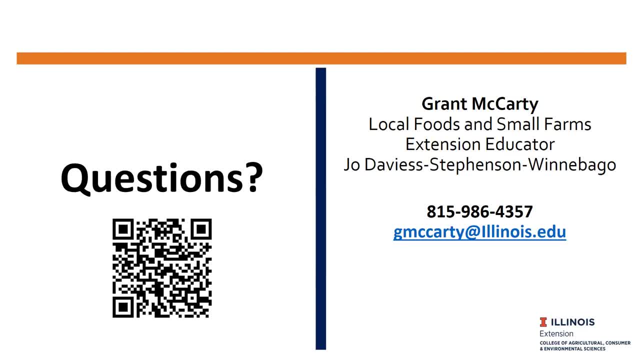 I mean, they're eating bacterial fungal, OK, great. And then there was a question about local experience with sand foin, which is a type of perennial herb, I believe. I don't have any personal experience with it. I think it's a leguminous pasture species. 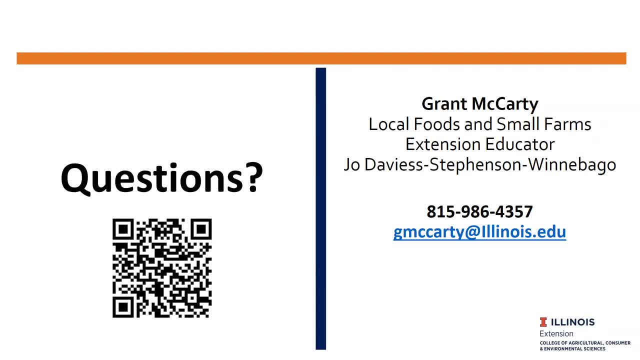 I'll just throw that out there. I don't know if we have an answer to that, but that was brought up And I know Doug's on the line. He's a co-host. Doug, do you have any experience with sand foin? 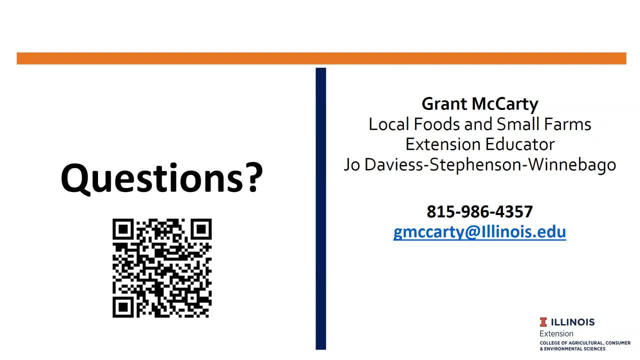 You can chime in at any time. Another question was related to modified Morgan soil tests versus standard soil tests. It was just a general question And I think that really depends on your specific soil type, pH and clay mineralogy whether you're doing modified Morgan. 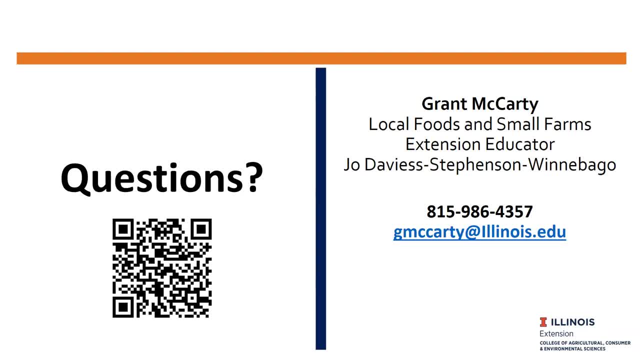 malic bray, so on and so forth. Do you have any comments on that? Yeah, I couldn't really. It depends. I mean, most of the time, most of the time we're seeing the standard soil tests to mostly address. 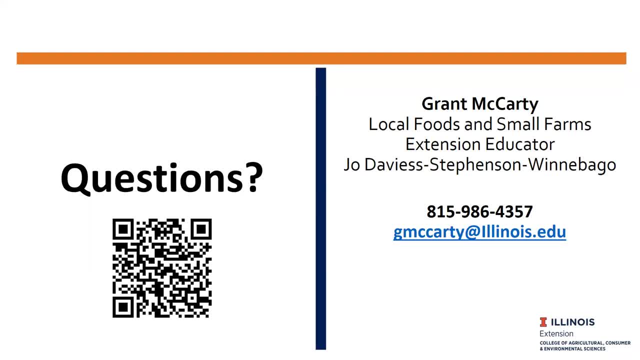 what your needs are, But if you are someone who is very active when it comes to really wanting to focus on your soil organic matter, then you may tend to lean heavier on some of these that are a little bit more particular with what your needs are going to be. 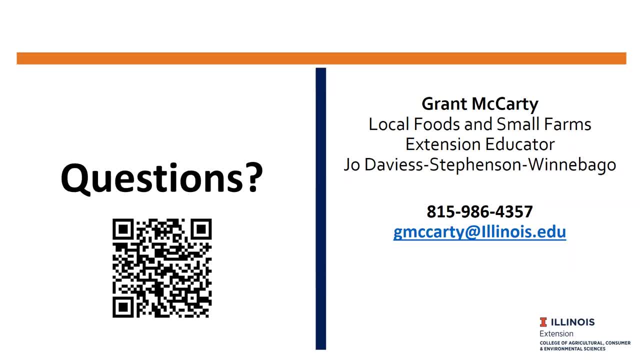 Yeah, definitely, as you've probably heard. if you've heard about soil tests discussed in the past, it really can be specific to your climate, Soil type and particularly with pH, when it comes to phosphorus analysis, that can be critical. 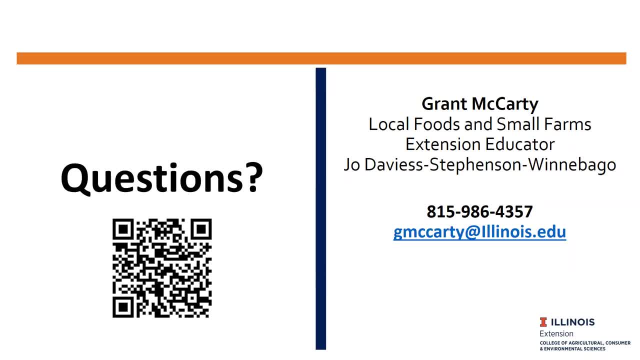 I know. if your pH is above a certain level, the sodium bicarb is probably better. If it's lower, a more acidic, weak, strong and weak bray Morgan malic. So it really, if you have those specific questions. 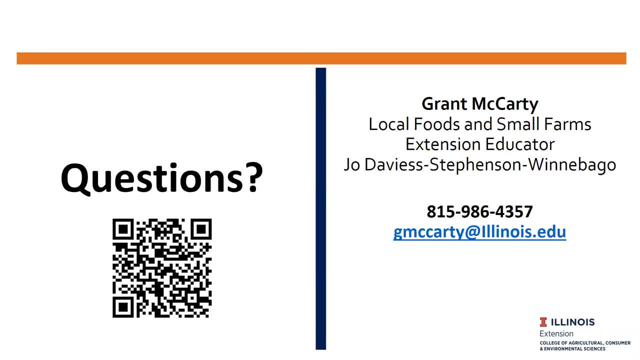 you can reach out to Extension or ask your local lab what they would actually recommend. So another question here: How does a green mulch consumption of nutrients interact with nutrient? What are the needs of the vegetables that you are growing? So in most cases, this green manure kind of product. 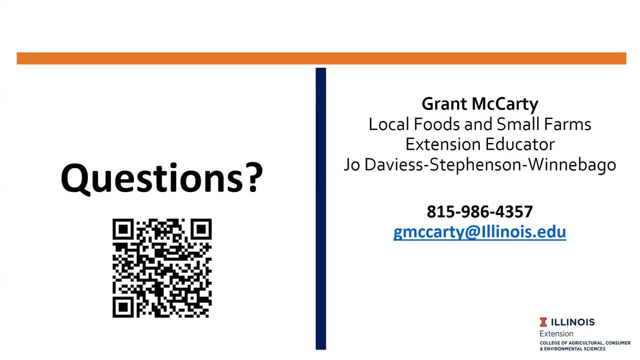 itself, especially if it's something kind of a leguminous, kind of a cover crop as it starts to decompose, it should in most cases make some of those nutrients available into that nutrient cycle for that plant to use. that You still need to create that green manure. 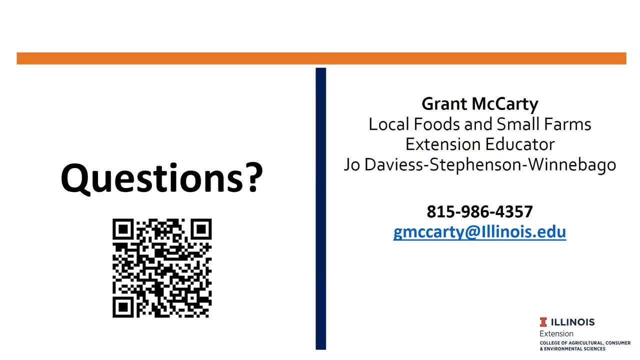 turn it into the soil and then sometimes wait a good month or two months in order for things to kind of stabilize a little bit and kind of get those cycles going. But you will still find that they in most cases will potentially address some of those nutrients. 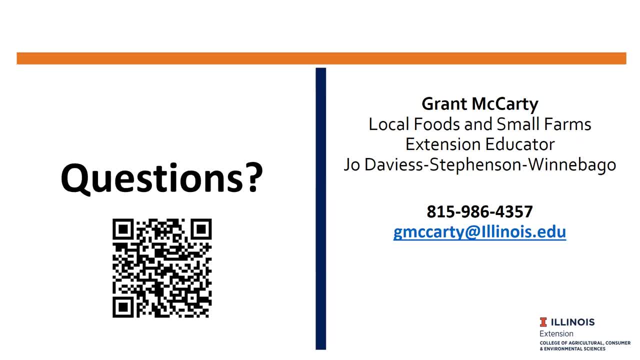 in that season, Great. So a lot of research out there about it. So a question just came in and I actually have an answer for it, but you can feel free to answer as well in terms of best method to turn under cover crop in order. 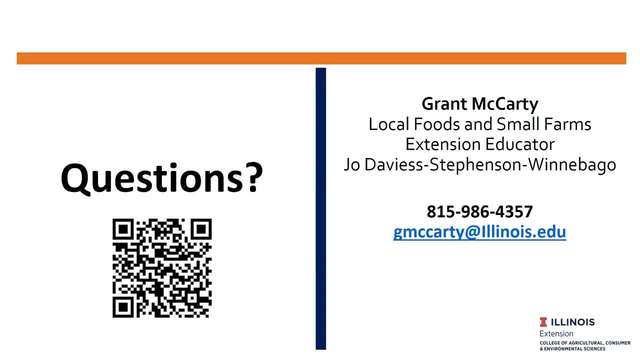 to minimize soil disturbance. So You know a lot of growers who are using sort of smaller scale no-till systems right now. I mean, one method they're using is the flail mode to terminate, and using things like tarping or soil solarization using clear tarps. 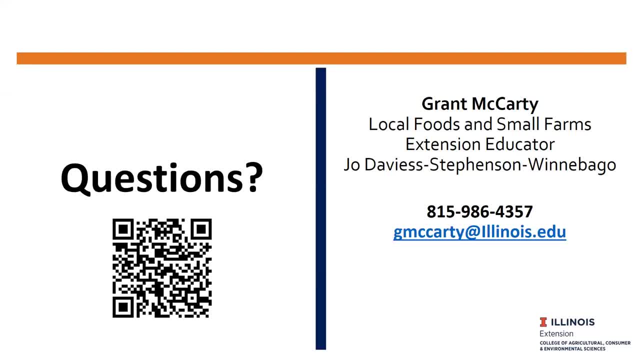 to kind of break down that material without having to actually till it in. You still have to wait maybe a two to three week period before it breaks down enough to plant into. but that is one method. Do you have any other comments? Yeah, that would be kind of the most common method to do. 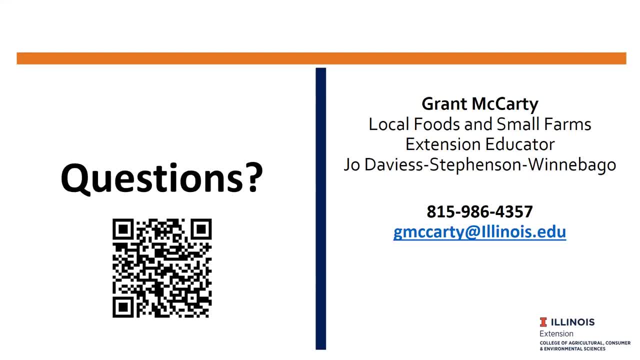 having some kind of flailing system in place to actually kind of get that organic matter in a place and kind of get a good bed kind of situated with it. Yeah, that's typically what we kind of see. It's not always a perfect situation. 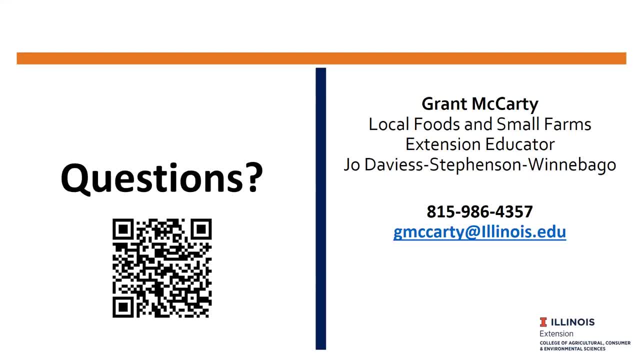 but it's something that you would play around with. OK, Someone in the chat box was asking something about zoo brew, which I'm not familiar with what that is, but I'm guessing that it might be a manure tea application or a compost tea application. 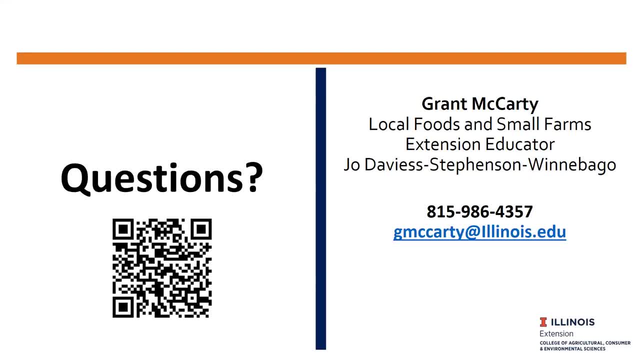 If they could clarify that we would appreciate that. But do you have any comments in general about manure teas or compost teas in terms of particularly stimulating soil biological activity? I mean, we don't tend to have just enough research to really figure out just yet if those have immediate changes. 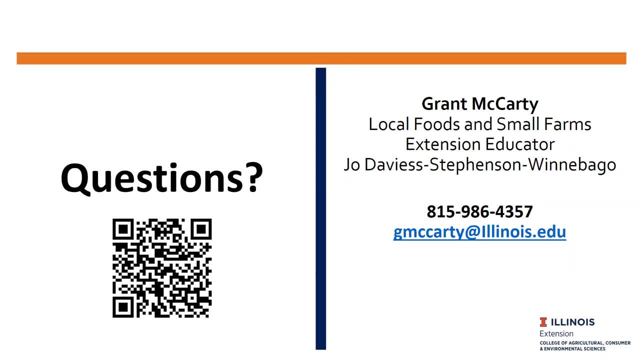 or long term changes in the soil system, the soil biological communities. Yet again, there's just so many factors that are going into that biological community that, introducing something that would have gotten there or never been there, we just can't really vouch for it as much as we wish we could with it. 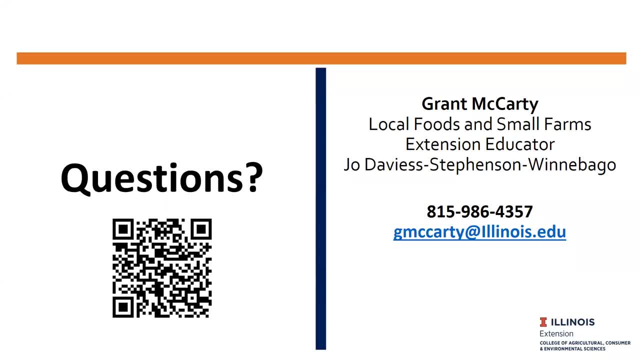 So there's just lots of questions and unanswered at this point, So we'll go ahead and make this the last question. Again, thanks everyone for sticking around. Does adding cardboard or newspaper under mulch impede soil aeration or cause other issues? I leave horse manure and wood shaving piled one to two years Can be added directly to perennials and garden annuals. should I age it longer before application? So I would think with your cardboard situation, if it's wet, if you have noticed that it is breaking down. 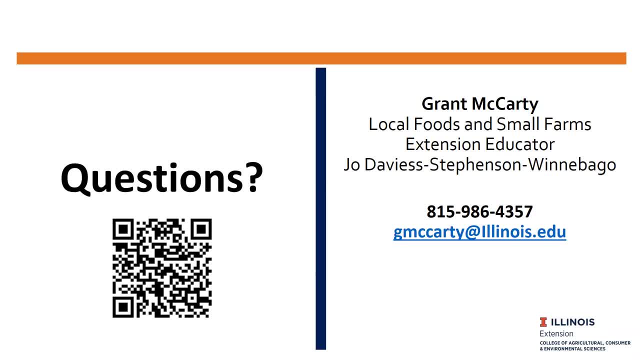 it should be OK. I'd still be a little cautious of it, just because you may have some limitations when it comes It comes to actually having some air exchange within it. As far as the second question, second part of that kind of the manure of it, it sounds to me 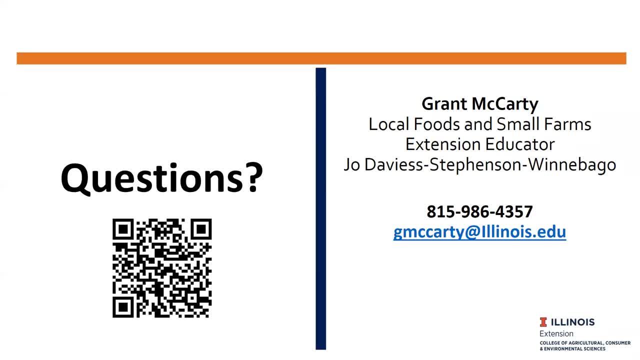 like it has been aged in those two-year process, So you should be able to then kind of utilize it quite well. So I would say it sounds good. But, like I share with you all, there's so many questions sometimes about what the best practices are. 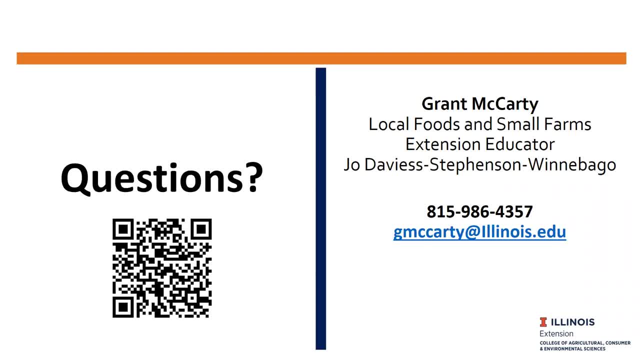 And yet again it's going to get back to your soil, Your soil texture and what the performance of that you've seen out of your soil too, Excellent. Well, I really want to thank Grant so much today for sharing his experience here with us.